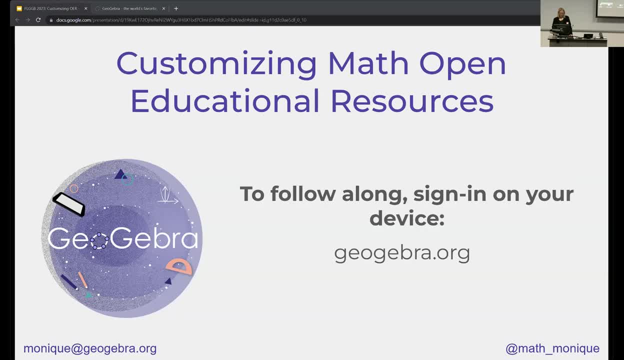 Okay, Monique, we are slowly starting ready for your presentation. I started the recording to record the session. We are so happy to have you here. Monique was with us last year. You can find her also on the GeoGebra YouTube channel recording from last year And she 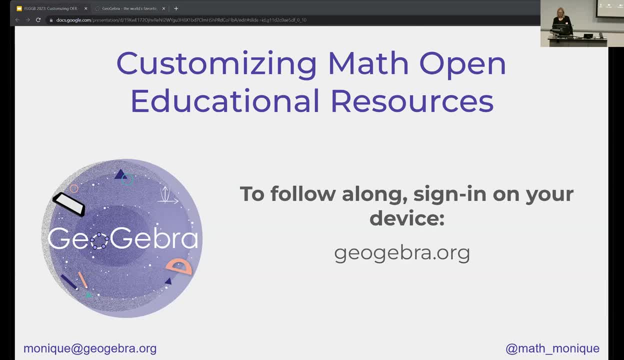 will be talking about customizing MAP- Open Educational Resources- Very, very, very important thing. We have a little bit of a glimpse of that when we have our Austrian friends talking during her in-live presentation, But now it's a whole session which will be focused on that. 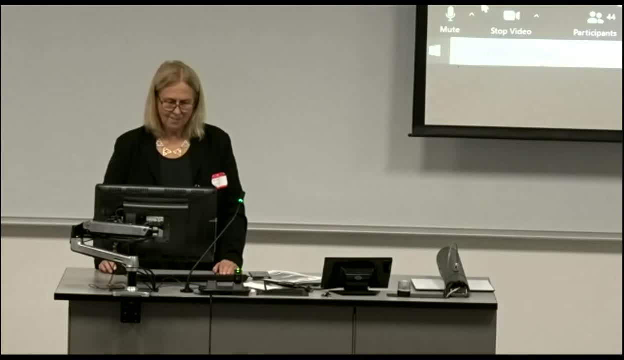 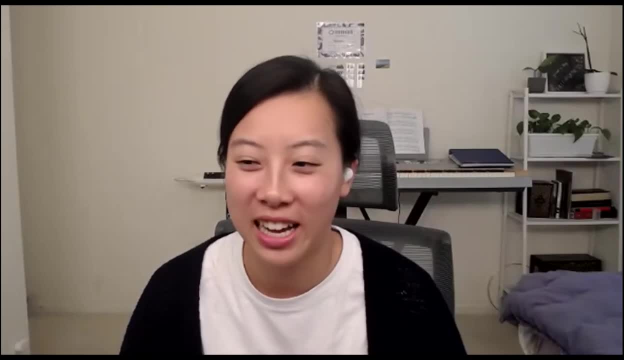 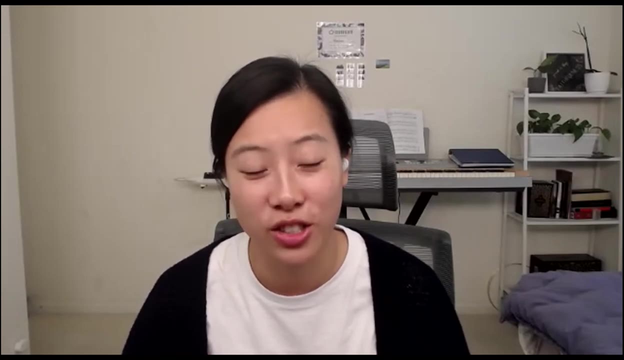 Thank you, Monique, for being with us. We are so happy And this is the stage is all yours. Thanks, Kasia, Thank you. Thank you, Monique. I am very happy to be here. I am on the GeoGebra team, as my official title is Lead Instructional. 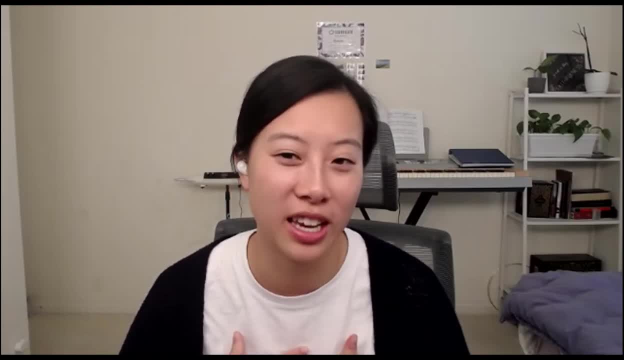 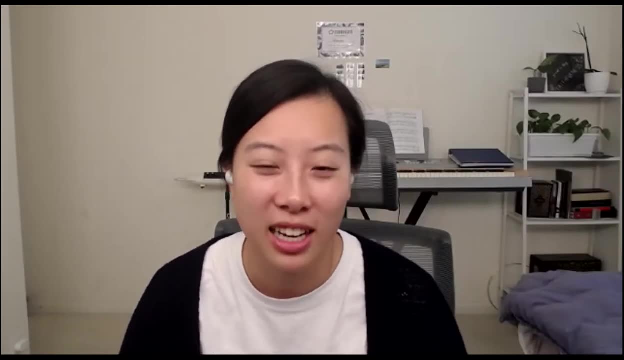 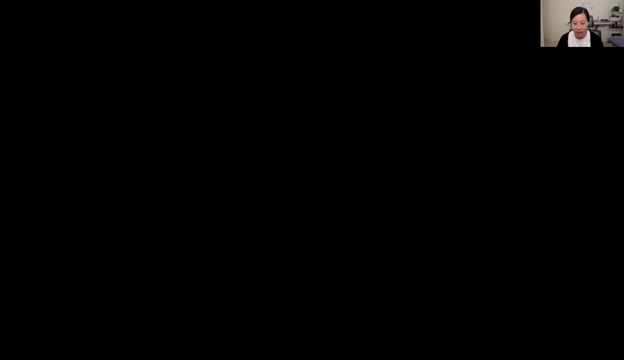 Designer, But my name is Monique and I am actually calling in from California, So the conference started at about 5.30 am for me, But this event is always exciting for me. I was sharing my screen and I'm going to share it again, But something you can do as. 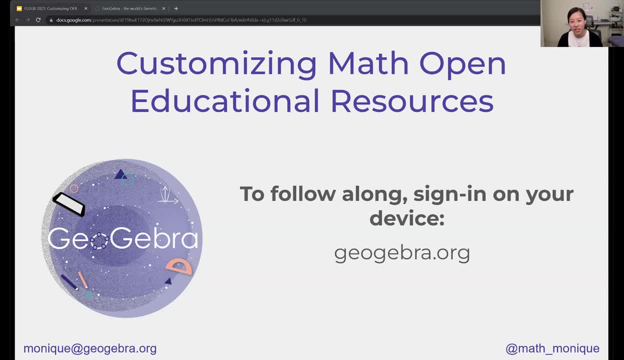 I'm continuing to just introduce The session and kind of get us started. I'll give you a couple of minutes just to sign in on GeoGebra. You do not need to download any of the apps or anything like that, But just if you have an account, which I assume you have one at this point after watching. 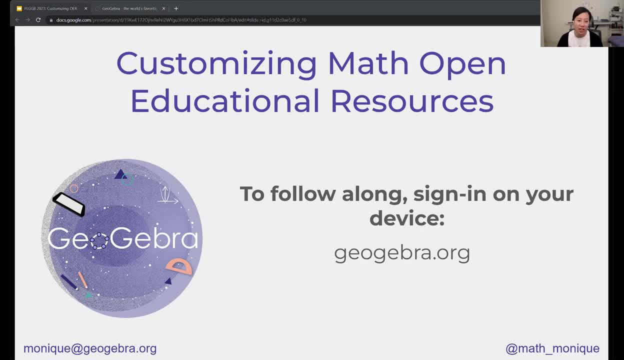 all of these wonderful sessions. just sign in. It will help if you would like to follow along and follow where I'm clicking on the web page, or it will help when there is an email or something like that. So I'm going to share my screen. 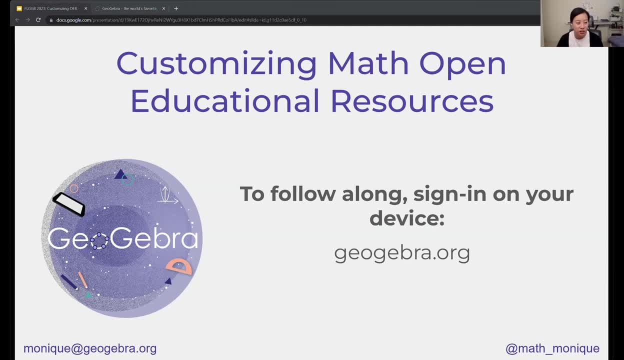 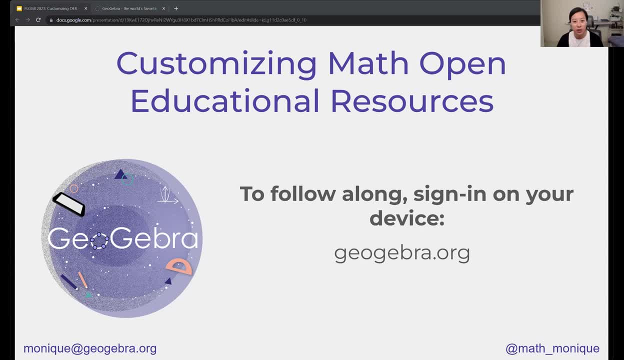 I'm going to show you a little bit of the session, So this is my interactive portion of the session as well. Yeah, So that's a little bit of introduction about myself. I have been using GeoGebra since around 2014, 2015.. 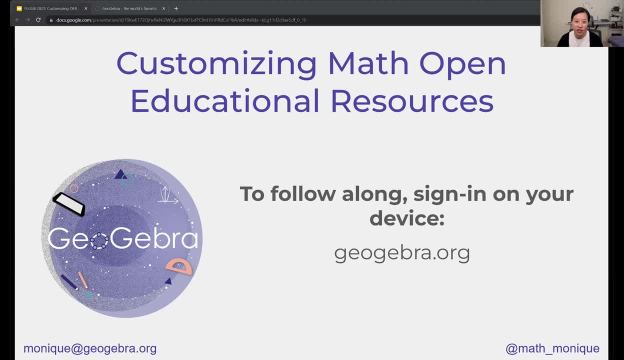 Used it in some classwork doing some numerical approximation work and methods. But I didn't really start using GeoGebra regularly until I started working in interactive, digital, open educational resources. So I started using it. I started using it in my course design. 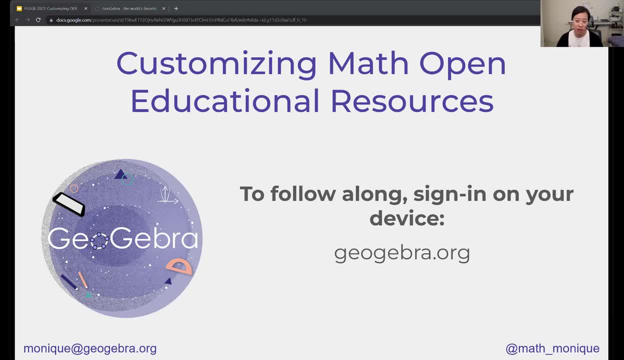 So that's what I'll be using the term OER, But when I say OER I just mean open educational resources, And I have been doing what I call like backend support work, which is just creating, to support or supporting the creation of digital resources and materials, especially ones that are open. 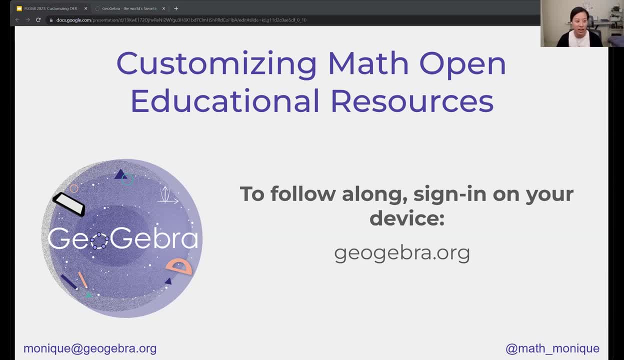 And so I'll get to talk a little bit more about what that means. But yeah, I am now at GeoGebra And I have been in my current role for the last three years, So I'm a student last about two and a half years or so on the content team And this is- it's just an exciting 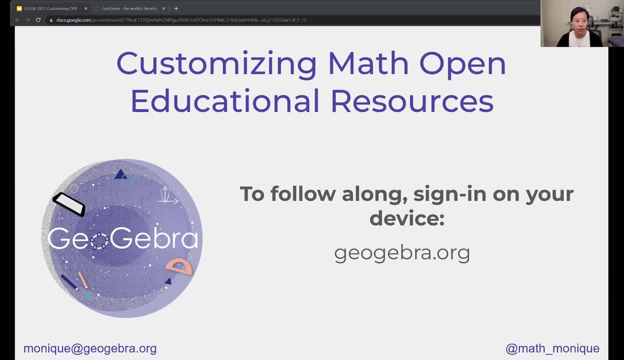 endeavor to talk about the ways that you can use GeoGebra beyond just the surface level resources or calculators that you see on the website, And so my goal in this presentation is hopefully to not only talk about how to mechanically use some of the features on GeoGebra. 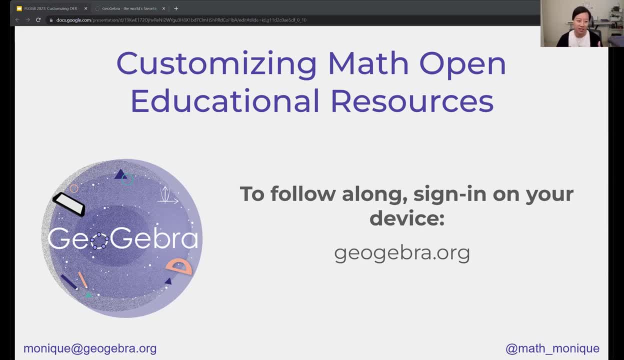 that have been mentioned in the previous sessions, but maybe it's. you need someone to walk through with you and show you exactly where to click and what to do and how to do it So you're confident on your own, but hopefully also just show some tips and tricks that I personally use. that might 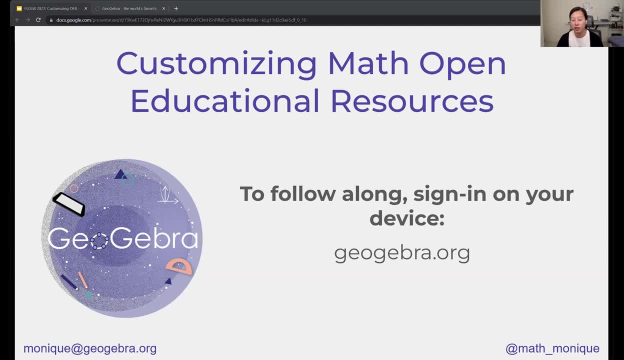 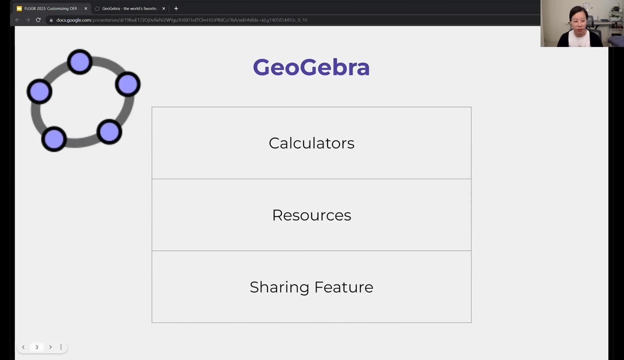 be able to help you with your workflow or even tell you some of the wording or how to explain just the power of GeoGebra to people who may not have used it before. All right, So just an overview of GeoGebra Generally. when in our presentations we talk about how we have three main components, One is the 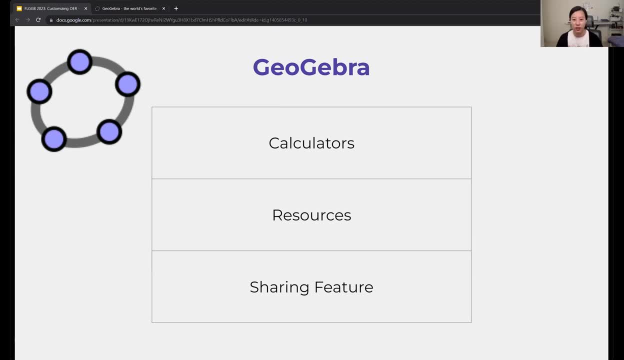 calculators- So you probably are familiar if you've been watching this conference or you've been participating in this conference- start off as calculators, like really nice graphing calculators that have gone above and beyond being able to use in the browser, through apps on mobile and with 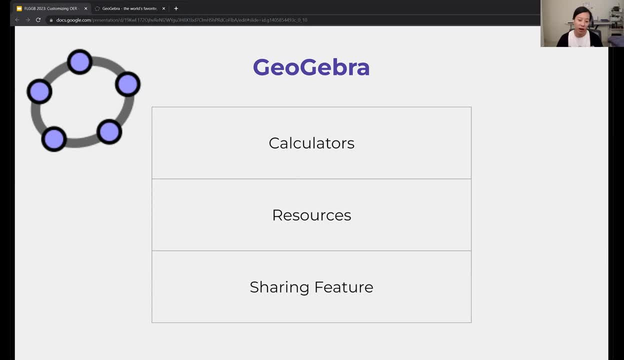 different exam mode features. And then you have the calculators that you can use in the browser. And then you have the calculators that you can use in the browser through apps on mobile and with different exam mode features and 3D graphing capabilities, things like that. Another is the. 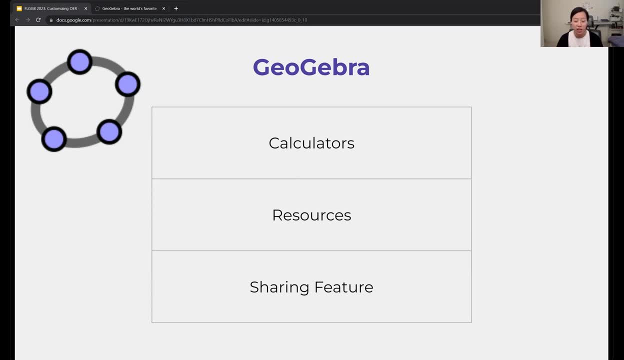 resources. So, using the powerful engine of the calculator, you can actually create really cool interactive resources and activities, ones that you've seen in the sessions prior and what we will mainly be talking about today. So that is mainly what we will be talking about, and how to, and 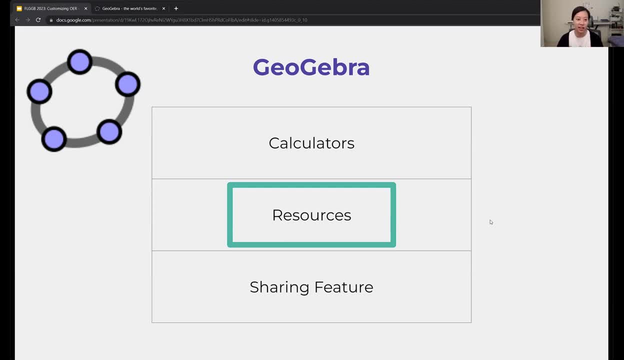 because we're going to be talking about how to use the calculator, we're going to be talking about these resources, So let's dive in and see what we have. So this is, this is a calculator, that is, you can even alter and create these resources yourself. And then the last component of GeoGebra. 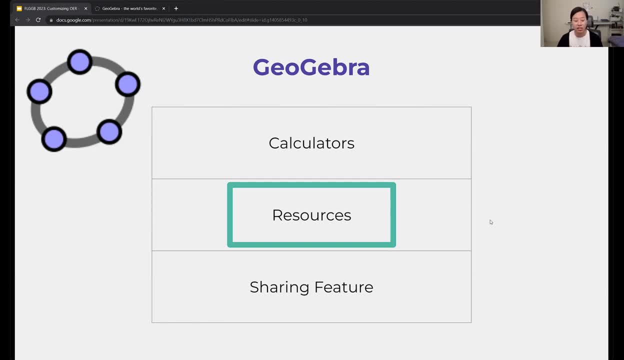 which is on the newer side, is our sharing feature. So this is GeoGebra Classroom, which I will introduce a little bit of in a bit, But it's how we can share the resources that we make, or the and the activities that are built off the power of the calculators. 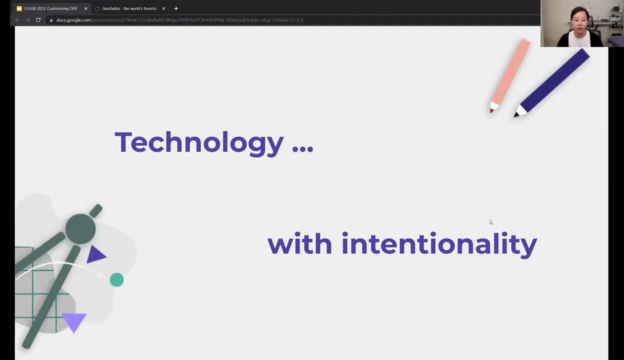 And so the first thing I'm going to introduce today is GeoGebra Classroom, And so this is a I did want to talk about, though is something that really we should be on the same page about. as I kind of continue forward, before even talking about resources and the ones that you might want, 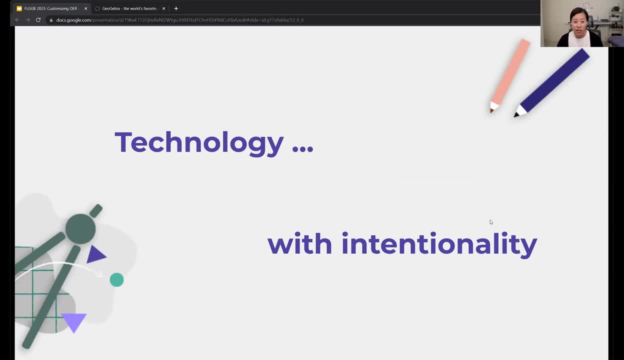 to look for in your classroom use or anything like that. Technology is very powerful, It can be, But I think we all know, and through the pandemic can testify to, how important it is to use technology intentionally. And so, in the same way that, yeah, we have things like smartphones now. 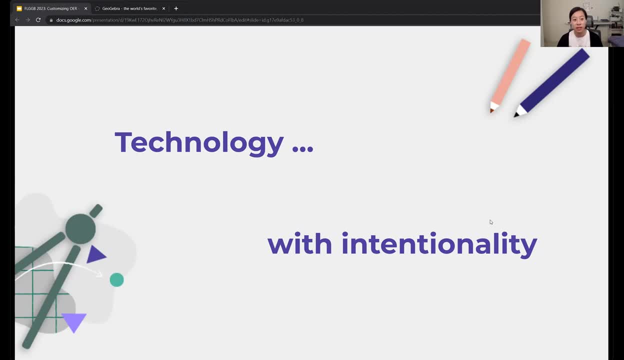 which can do a lot of great things, it can also sometimes be a hindrance, And so the example that I've been using recently is the example of just a well-drafted email, because I think everyone kind of understands an email compared to the traditional snail mail and writing papers, and 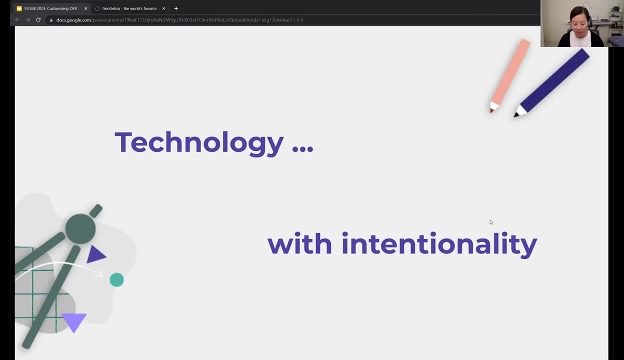 having it sent. you know taking data, I mean, if you're working with people who, like you know, have so many days to send and it having, you know the possibility of it being like getting wet and getting ruined and ink smudging and things like that. 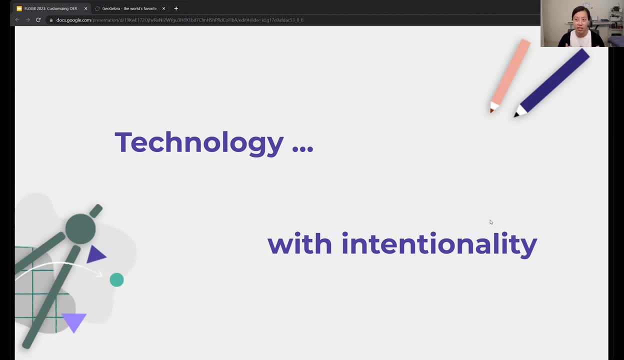 or getting sent to the wrong place. we have this really cool technology of being able to send something digitally that can be easily forwarded or you can easily reply to it. It sends instantly. It looks nice, It can look nice, Yeah, And it's just the. 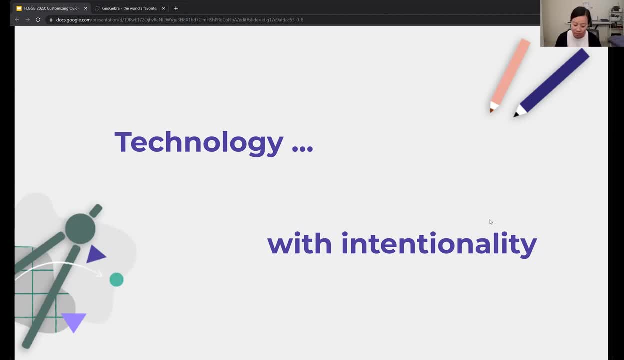 there is an ease of that: you don't have to have a pen on you, you just have your computer, um. but we've also all seen just the example of a poorly drafted email, which I think you see, you know what I'm talking about- just chunks of text, um, maybe it's not very formatted, and 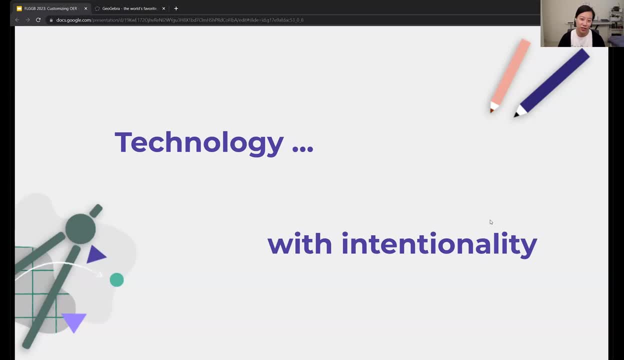 they did not put a paragraph on a new line, or there's fonts that are really hard to read, or, um, just different bright colors that hurt your eyes. um, yeah, we've seen emails like that. um, but we can't deny that an email is very useful, um, but if we use the, the email format, well then. 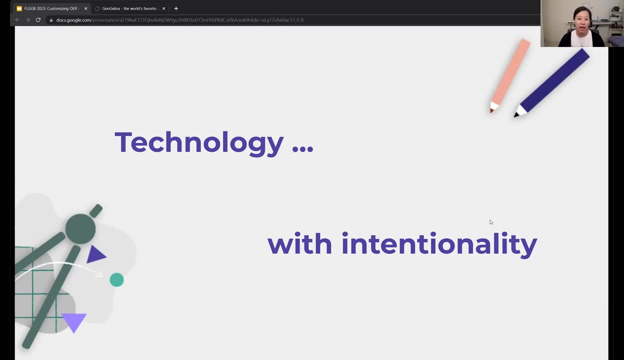 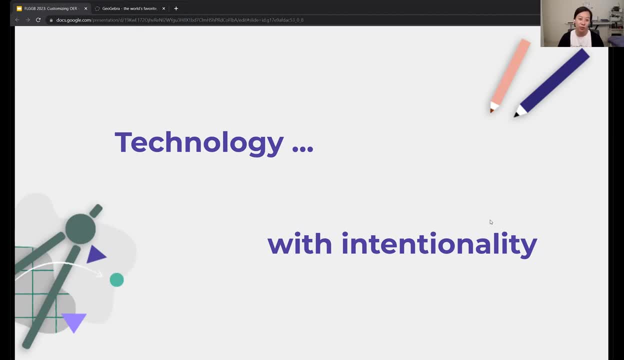 with just specific choices that we make, we can really enhance um our communication abilities and in the same way, I think you've seen in the previous sessions, we've seen a lot of really cool uses and applications and the ways that it can connect to the math concepts that we're talking. 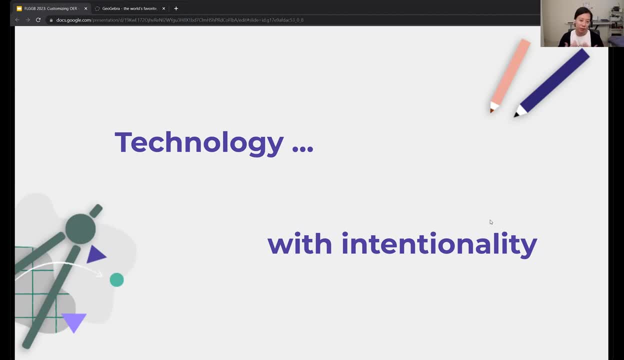 about. but I will say- and as a representative of GeoGebra I will say very boldly: if there is something that can be done better elsewhere, don't use GeoGebra, like if there is. uh, if something can be done better on pen and paper than on the computer, do it there. um, but if you use GeoGebra, well then there are. 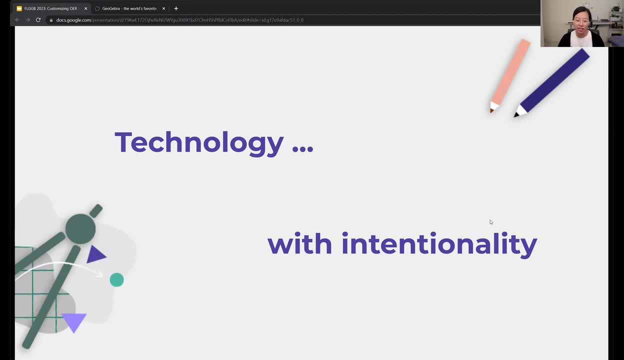 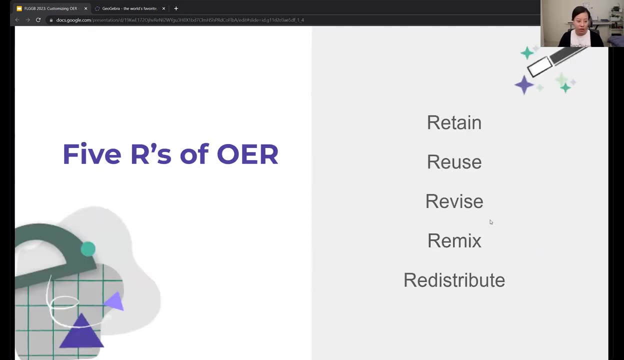 opportunities for to really enhance your instruction, um, really get students to make those connections, opportunities for you to ask better questions, um, and just really understand, uh, not only math in a new light, but also understand technology and technology use in a a new light. and so one of those ways that we can use technology differently- 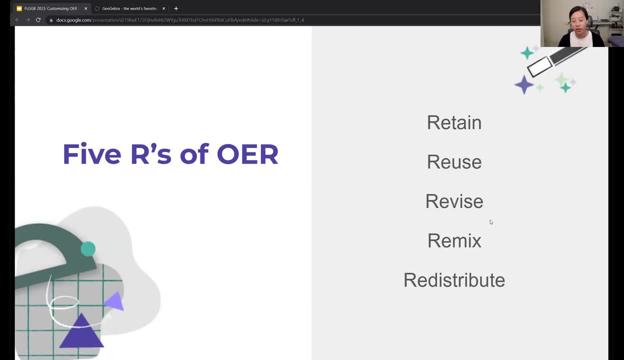 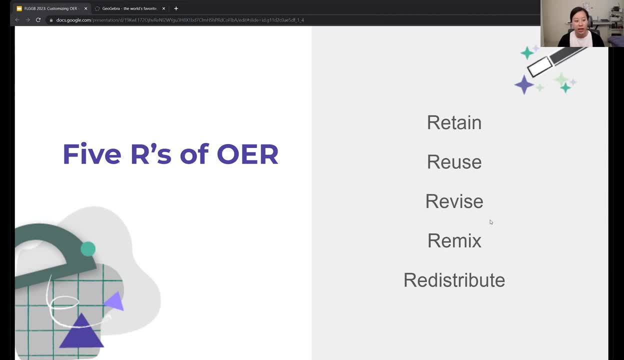 the nitty-gritty of OER and things like licensing or anything like that, but the idea is that OER is open. so the uh, you can. you find it online and it's free to use. it's free to. you can keep copies of it, you can reuse it, you can make changes to it. 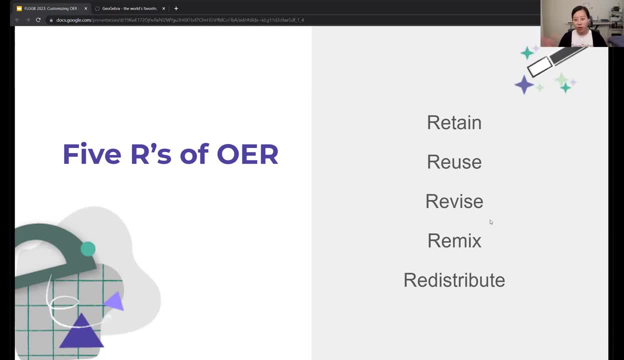 you can pull in uh from various OER resources and put them together and you can take what you've made and redistribute it. so I listed the five r's of OER here on this slide, um, just to get your brains thinking a little bit about. okay, what can I do with whatever I see on GeoGebra, because I don't. 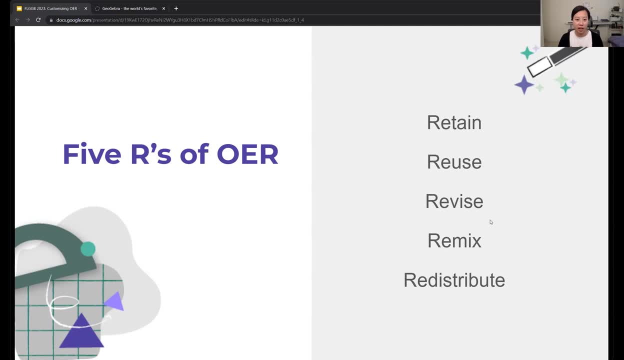 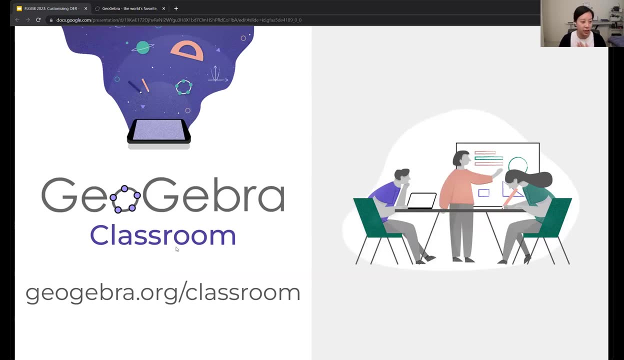 just have to use it as is. I can do more with it, um, and so we'll talk a little bit about that today, um, so I'm going to go ahead and share my screen with you guys, so I'm going to go ahead and share. so, first off, because I don't think it's been shared, at least, um, in the virtual sessions, but I 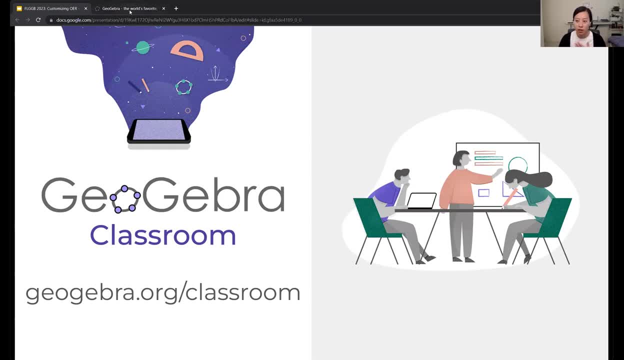 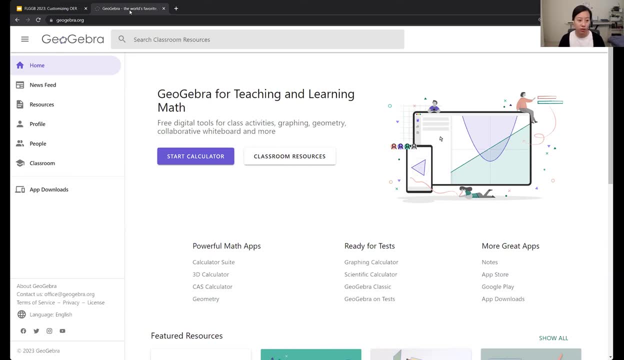 wanted to show a little bit of our sharing feature, GeoGebra classroom. so it's been mentioned a few times, but uh, basically, when you come onto the GeoGebra site, you can look for resources in a bunch of different ways. so you can either just go down here, use the calculators, but I'm talking 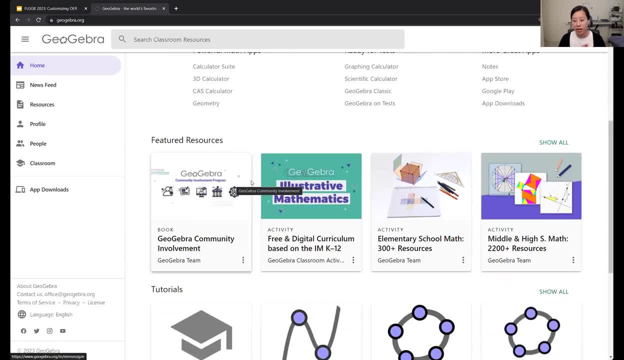 about going down to some of these links and looking at some of the resources. so on our site we have a curriculum that is authored by illustrative math, a version of it here. we have elementary school math resources, middle school, high school math resource collections. so if you click on some of these resource collection links you can go through. 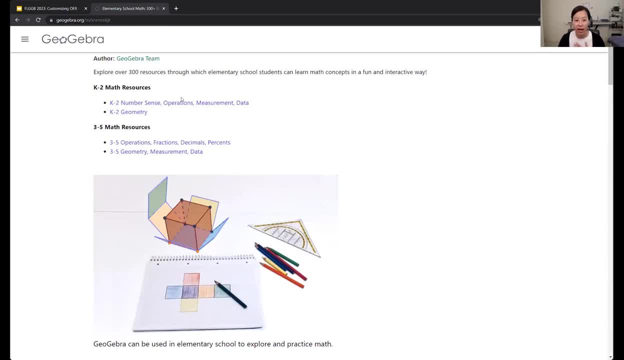 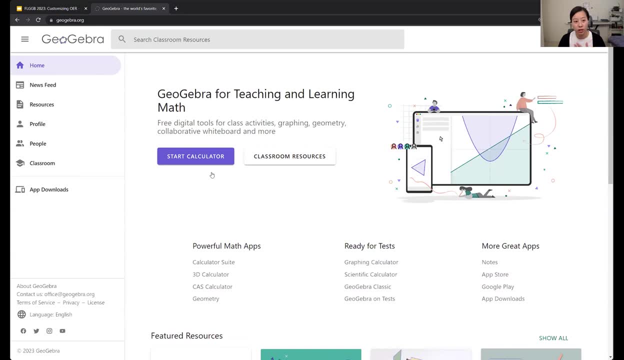 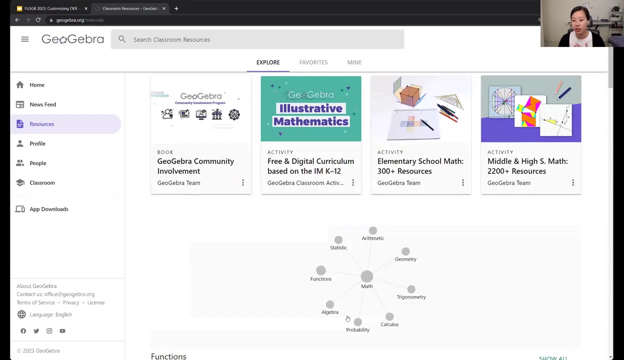 and see some of the curated options that we have and then, anytime you want to go back to the home page, you can click on our icon or you can go under this tab on the left- resources- and just explore. so you can explore by various concepts and topics. you can scroll down, find something. 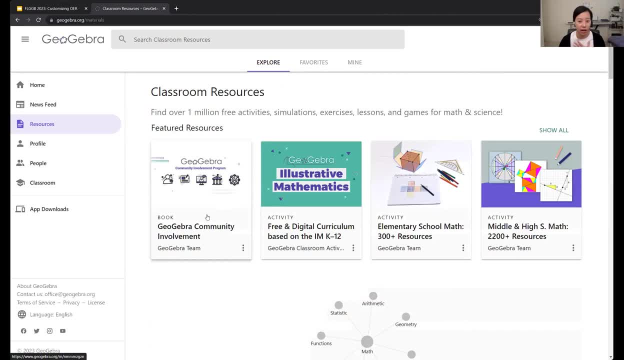 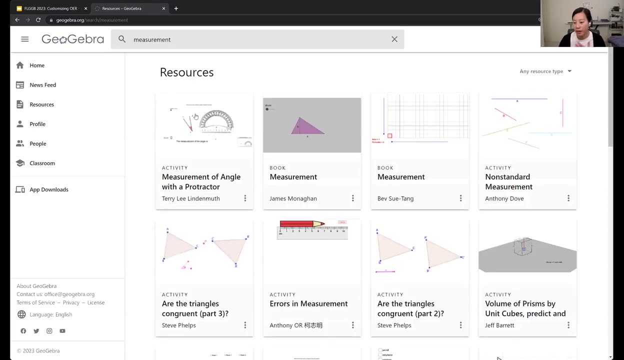 or generally how I, as an instructional designer, how I assume everyone's looking for resources, is: you have something that you need to teach this week, so you need to search for a particular topic. so maybe I am searching for something in a measurement, and so usually these measurement activities are something like upper elementary. 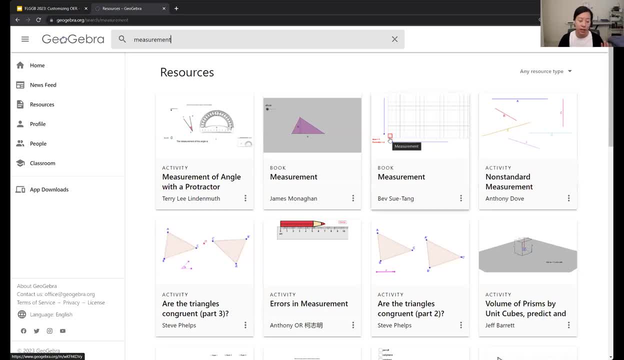 level I like, at least in the US. but you can search for whatever topic in math that you are looking for so there can be resources for higher level advanced mathematics. our calculators do handle a lot of those higher level math concepts or even just something that's towards the elementary level. 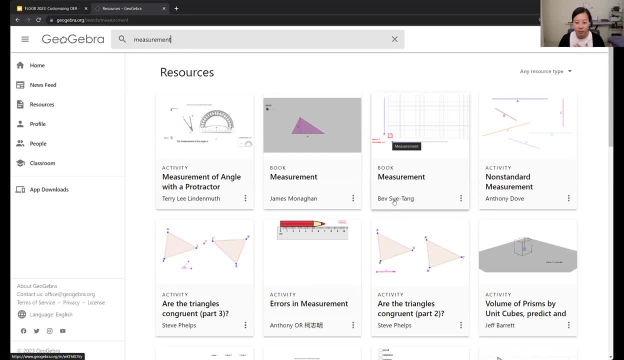 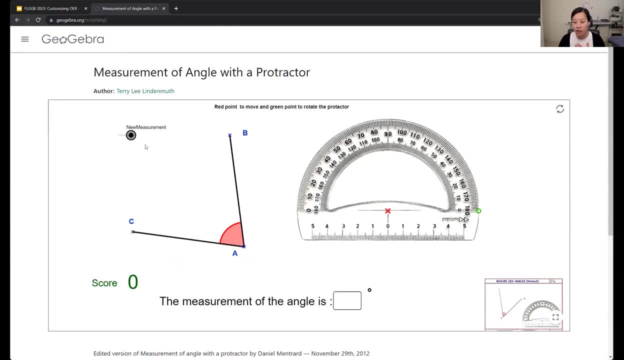 just because our resources can be interactive. so I'm just going to pick, click on one of these links and you can see there is these resources here and these are. these resources are resources in particular that I'm searching for right now are all created by the community, so 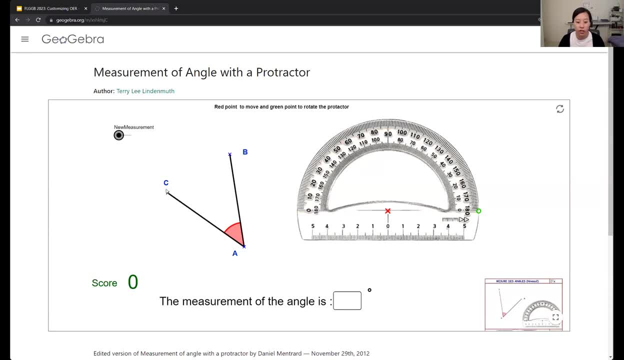 there are a lot of great options for just seeing the creative things that teachers want to make and want to use GeoGebra for. these are not the ones that you just search for, are not necessarily curated by the GeoGebra team, and so if you want to see something that's curated by the GeoGebra team, 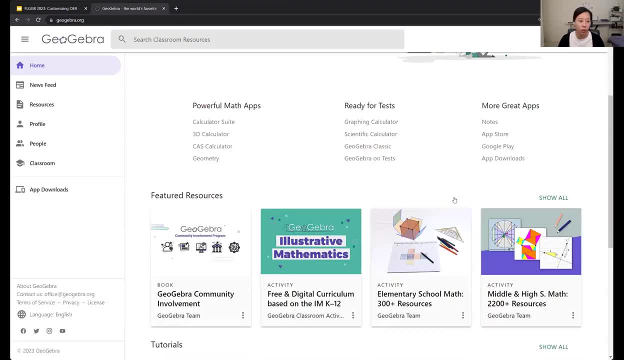 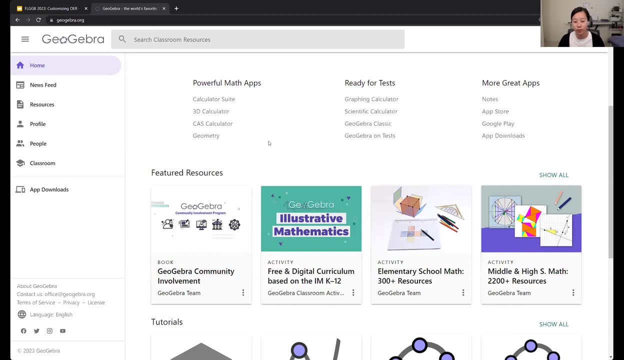 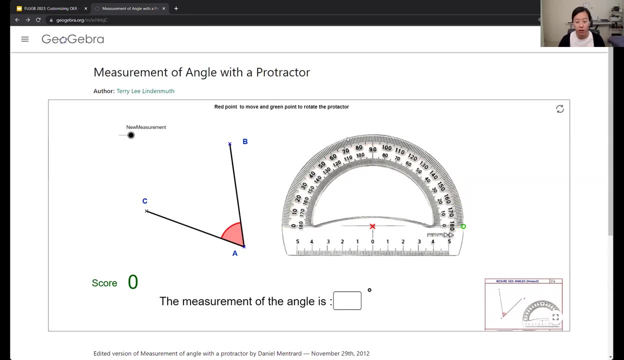 like I said, you can go to the home page and just click on one of these featured resource collections, but a few ways that, as we're talking about OER. one of the things that you might want to do with OER is: you just want to retain it, you just want to keep a copy of it and you just want to save it. 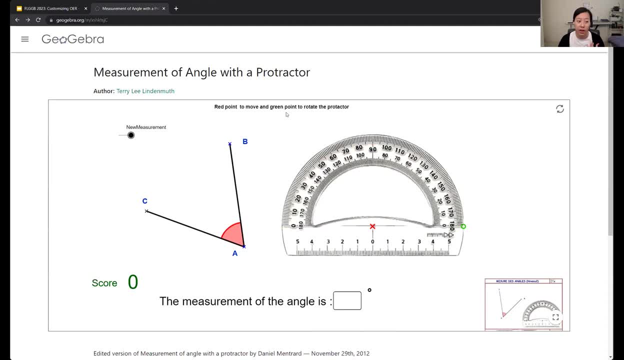 and use it for later. so I'm signed into my account right now. but something I can do is I can save the link, just copy and paste the link somewhere and save it in like my notepad. I can do that, and something I can do is just take the link. I can share it with my colleagues or share it with my students. 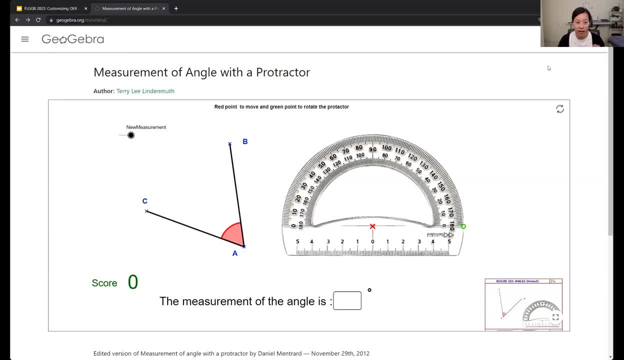 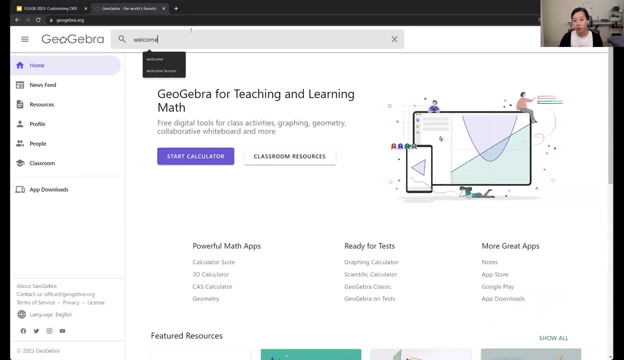 directly. that's fine, but something that I could do is I could also just assign this lesson, and so when I click this button and click assign, actually why don't I show you a resource that I like to use that shows a little bit more of the features of GeoGebra that you can find in some of these? 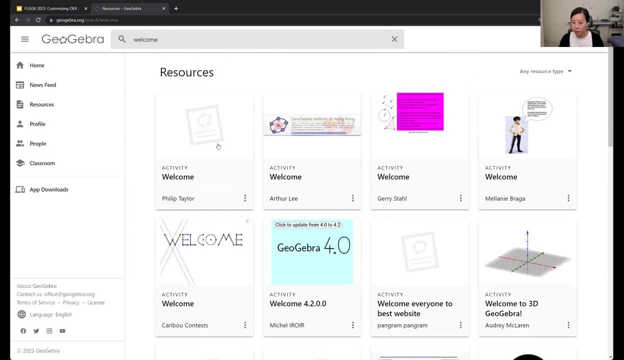 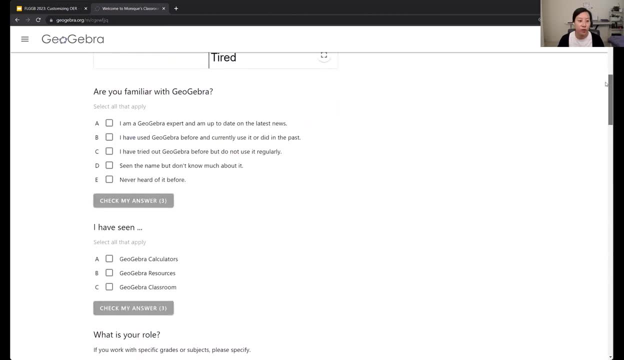 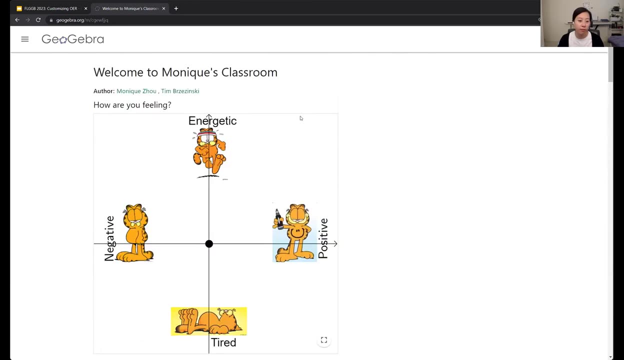 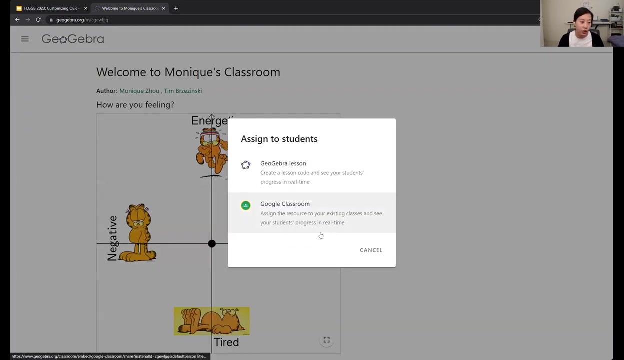 resources here. here we go. this is a welcome- uh, kind of welcome- to GeoGebra activity that I had created in a another account. um, and instead of just sharing the link with you, I will show you the power of GeoGebra classroom. I can click the assign button and if I had you in a Google classroom, I? 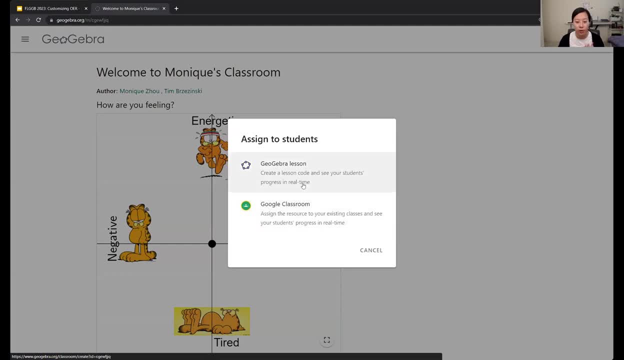 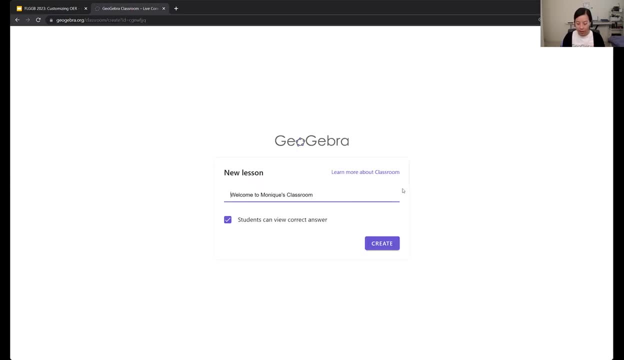 could assign it in Google classroom, but since I don't, I am just going to create a GeoGebra lesson, and when I click this option, what this does is it allows me to create a lesson um a live lesson. so let me name this so that I can reference it later. but yes, so here is an instructor view of this live lesson. 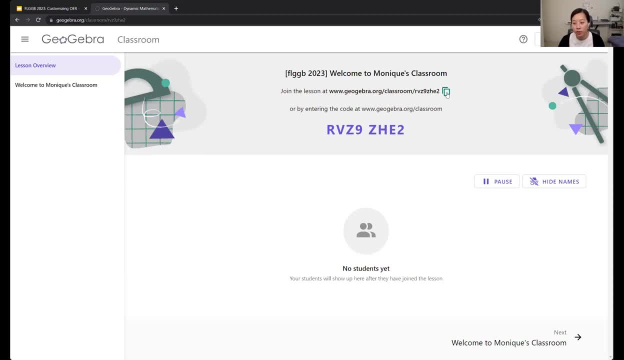 that I can now distribute to my students. so I'm going to copy this link and then maybe I can get some help sharing this link to all of you all who are online. but uh, basically you can just click on that. uh, the link that hopefully will get shared to. 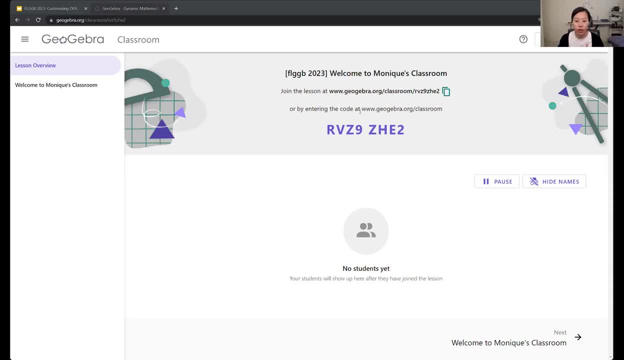 everyone eventually, or what you can do is go to GeoGebraorg slash classroom and there will be an option for you to input this code, so you can go to GeoGebraorg slash classroom right now and put in the code. so yeah, that is what I truly I枠t do. 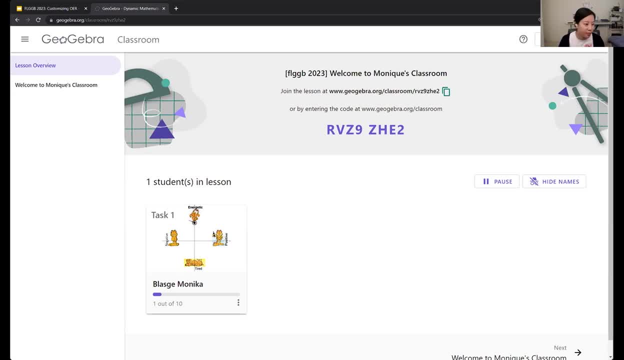 so if I click add focus the view so that'll create thatилась call. I can go down here in these key así so I can go through all of these features that are for discussions and give. I can click lock on one And so you can see from this page. I can see anyone who just hops into the lesson. 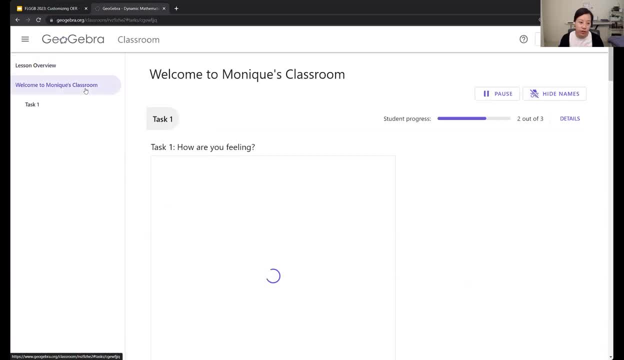 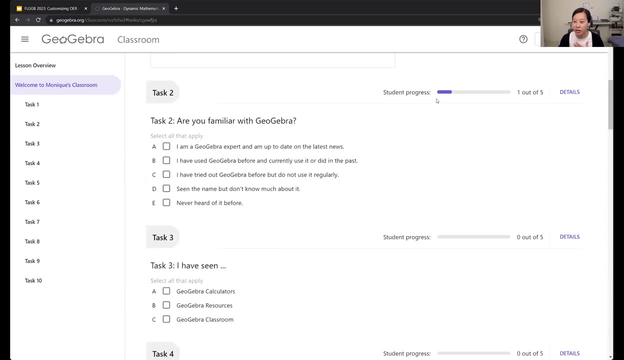 Um, I can go into this tab here on the left. I can look at just general progress in my students. Okay, I see two out of four have worked on this task, or two out of three out of five, as it's updating in real time. One out of five. Okay, I can look at that. I can look at each of the. 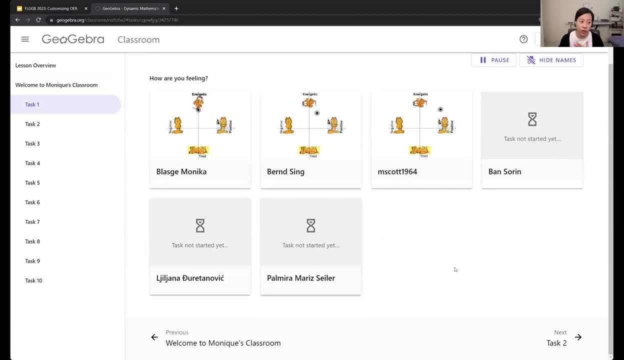 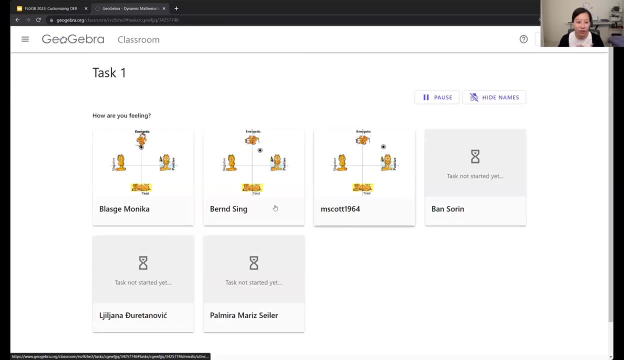 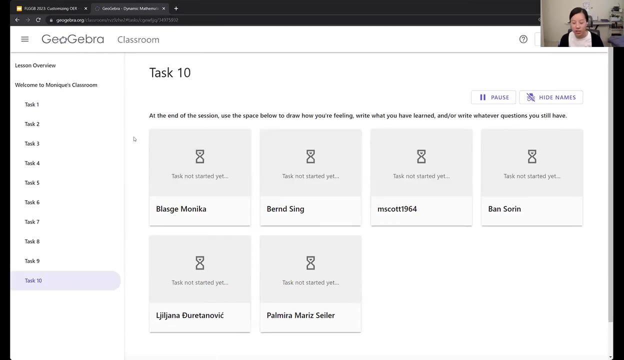 individual tasks. so I can see just a general overview of the first activity, where I'm just trying to figure out: oh, how, how are my, uh, how are my students feeling today? How are you all feeling today? Um, yeah, I can see no one has started at the one at the very end, which is: 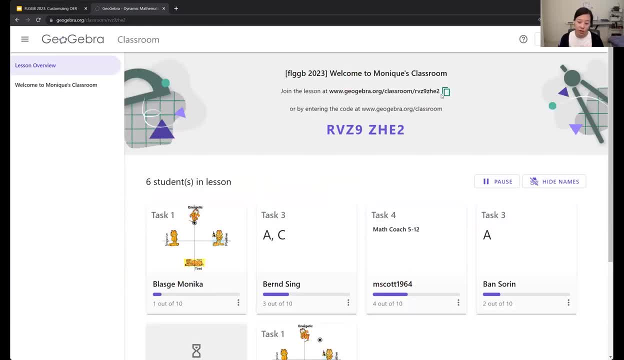 expected, but, as you can see, with this link that's created, I can just copy and paste this into whatever LMS I'm using If I wanted to do a one-off activity, like I just wanted my students to do. just this one interactive activity on um graphing linear functions. 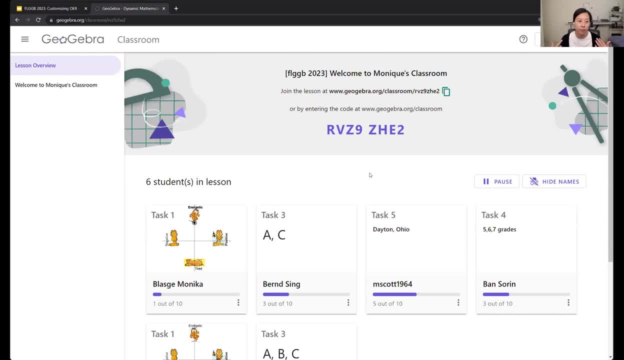 Then then I can just create this one and go send the link in my zoom chat or just have them join on their devices with this code: Um. and also, you don't have to have an account to join as a student um. for the purposes of this uh conference, I'm asking that you join um with your accounts. 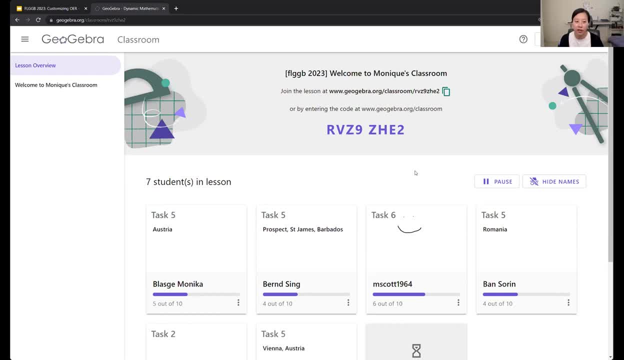 but uh, if it was just a one-off activity, uh there, and if you're not signed in, then you can actually just input your name and join. Um, if you are logged into your account, you have the extra benefit of it saving to your account. 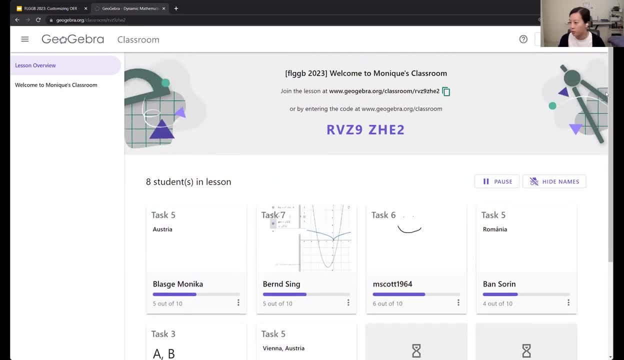 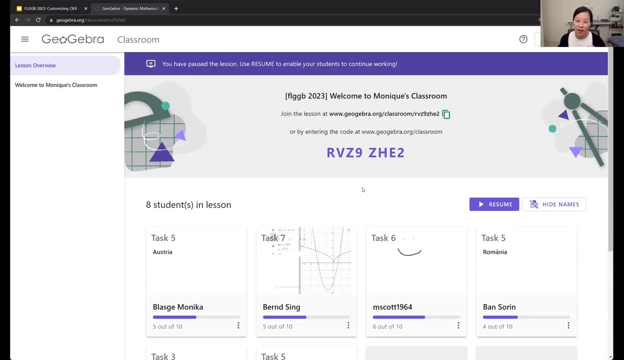 Um, a few other features before I move on. but, uh, I can actually just pause the class. Um, and usually, if I were uh showing this in person, um, when I hit the pause button I hear an audible oh uh, and then I can make an announcement. Maybe I can clear up any sort of 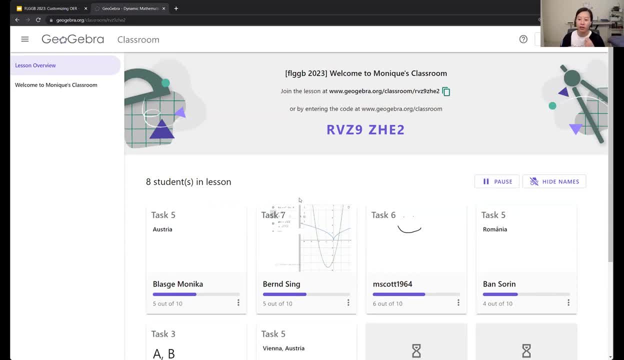 misunderstanding Um, and then I can make an announcement. Maybe I can clear up any sort of understanding that's going on, Um, and then I can let you keep going. I can also use the pause feature if I wanted to create these links and send it over to my students, but I pause it so they 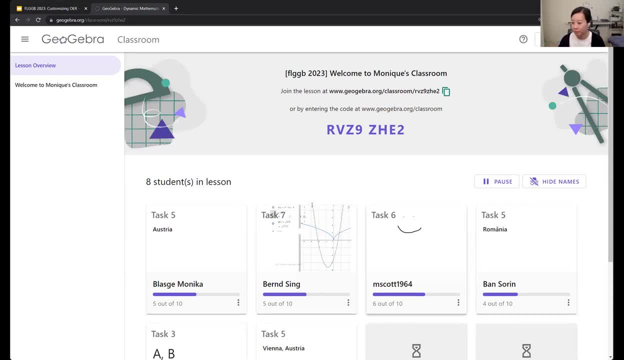 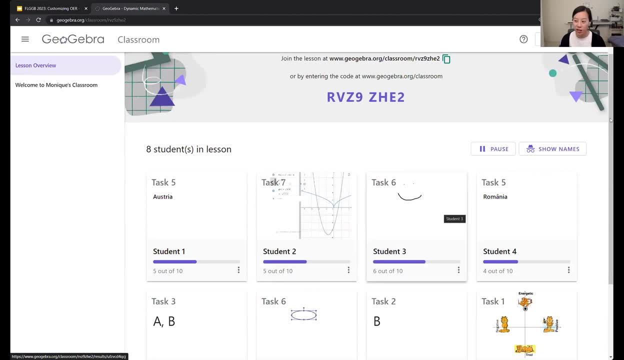 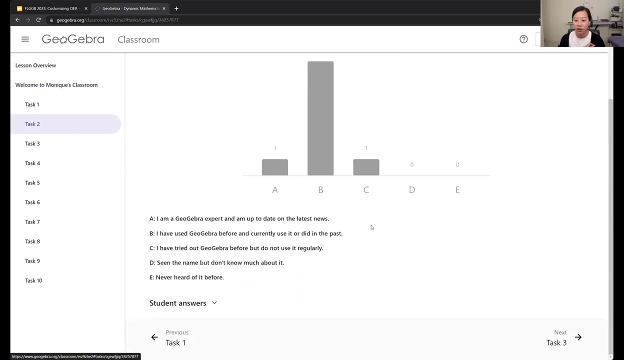 don't work on it right away. Um, I can also anonymize the students, So that way, what I can do is I can continue to show this um projected onto a screen in the classroom and maybe we can discuss. um, oh, like, look at- let's look at- this question. I would like to see if there's any. 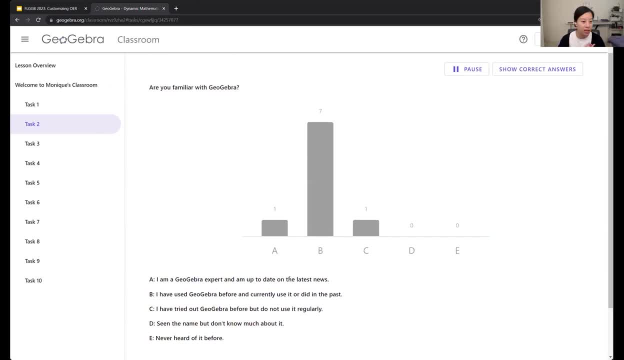 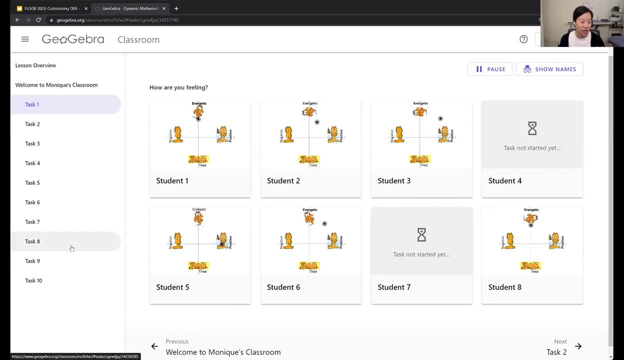 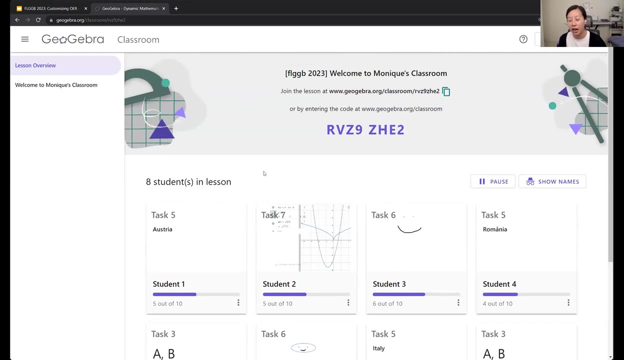 questions. I was asking how many are familiar with GeoGebra and we? maybe we can discuss this or maybe you know we can generally see how the class is feeling. We can all empathize with one another and I can make adjustments to the class. um as I continue on. Um, and so this is uh. 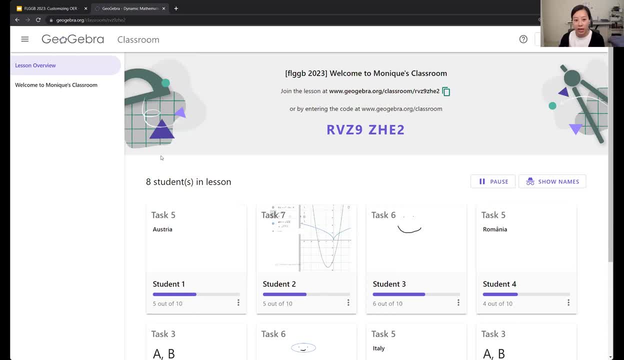 how I mentioned that we can share these resources. but, uh, what I can also do is I can also go onto this menu. I can view what the students are viewing. So if I open this up, I can see, you know. 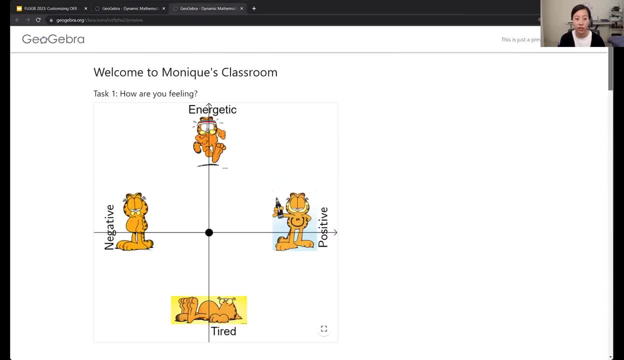 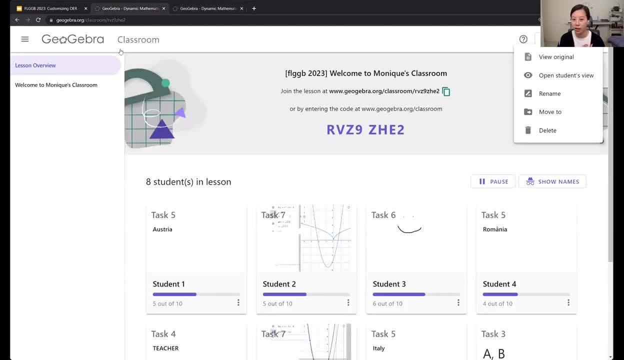 in a new tab I can see. okay, this is exactly what the interface for the student looks like, So they won't see the extra uh bar on the side that I have access to. I can also view the original. So maybe I was uh, I wanted to see. okay, exactly which resource did. 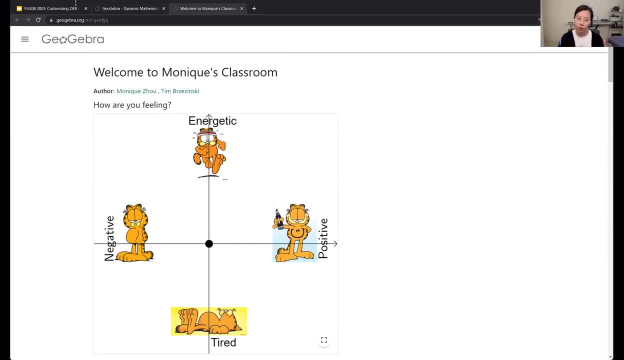 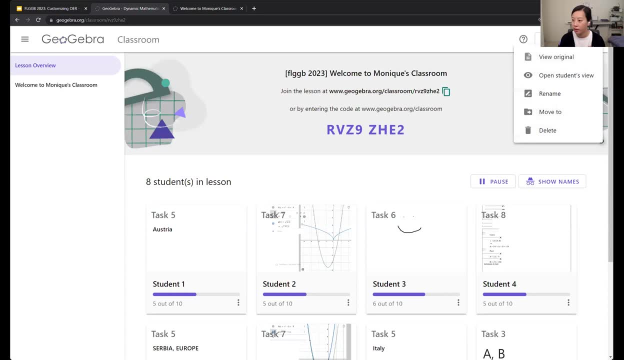 I pull this from And I wanted to look at maybe the original author or something like that, see what other resources, resources that they might have. Okay, Um, yeah, I think that's about it for now. Um, so, if I let's say, I also just 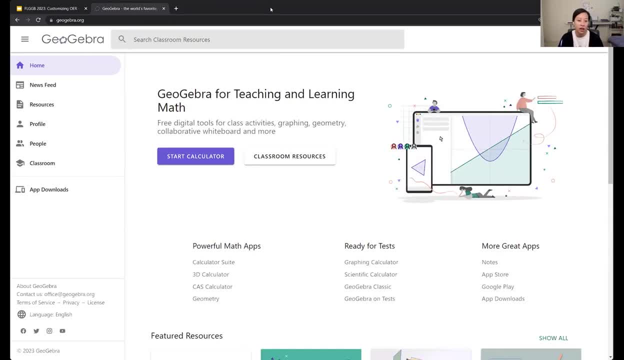 closed out. I left the link here. Um, how I can access this uh live classroom again is I can go to my profile, I can look and here is the lesson that I created, And here's that view again. Um, so this is very helpful. 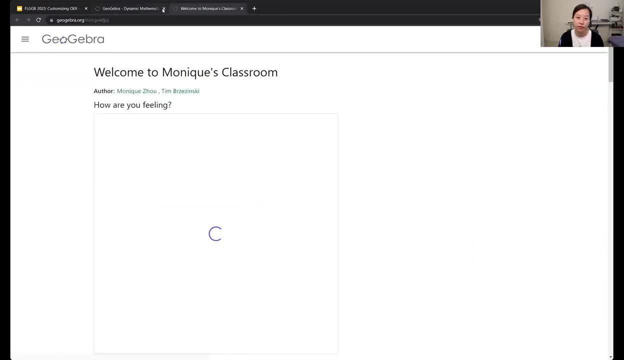 Um, and so let's go back and look at. okay, I've found some resources that I really like on the site and I just want to save it to my account. There's a few ways to do that I mentioned. you can just use the link. the link, the way that it's formatted is you have geogebraorg. 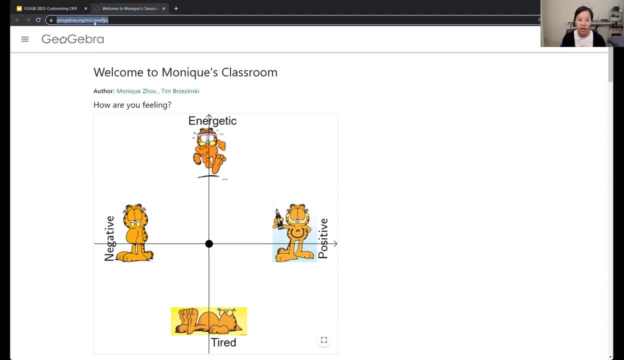 There's a slash- M- M stands for material- And then there's this: um, eight digit code that follows or, um, eight letter code, Um, and so this code is basically how you identify each individual activity, Um, or individual page here, Um. but what you can also do is you can go to the three dots in the 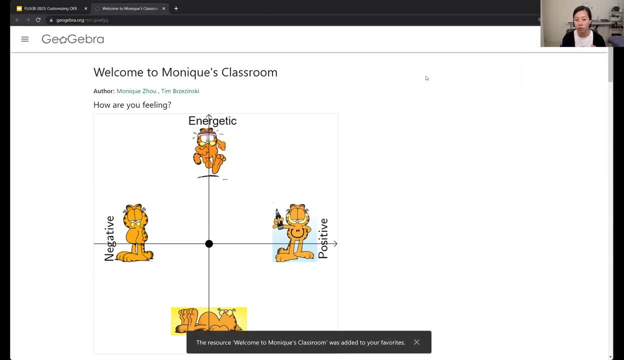 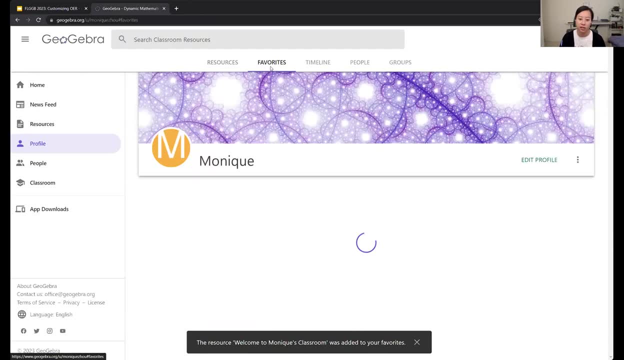 menu You can add to favorites. So if I wanted to save this one to my favorites, then when I'm on the homepage I can go to profile Um and I can look under this tab, favorites, and I can see some of the extra resources that I saved Um. and then now again talking more about just how we can use. 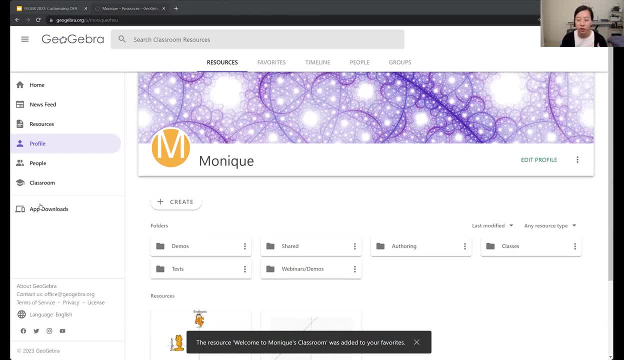 technology Um, and then I can go to my favorites Um, and I can go to my favorites Um and I can in uh OER. not only can we just save um and reuse all of these uh resources like I can go. 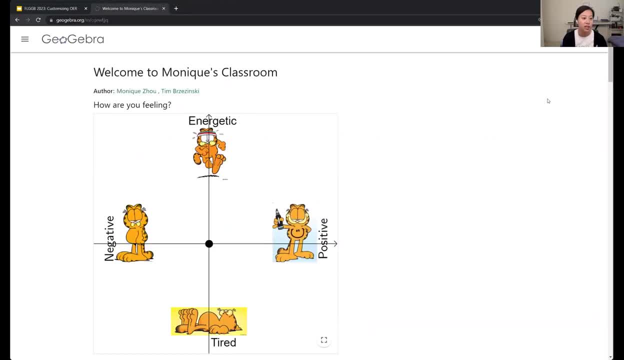 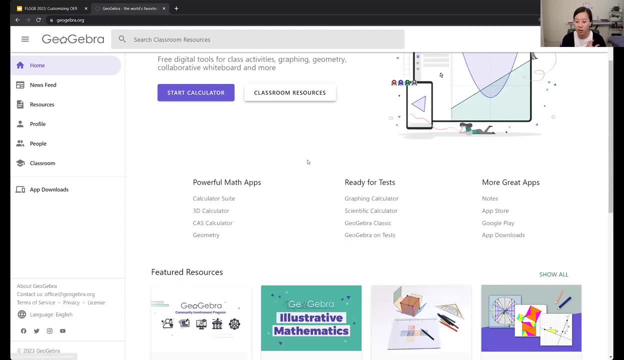 to go back to this link, I can make a new classroom, uh, because I have a new session in a conference or something like that, or a new, uh, new period that I'm teaching. But, uh, something I can also do is I can actually make a copy of the individual resources. So let's take a look at 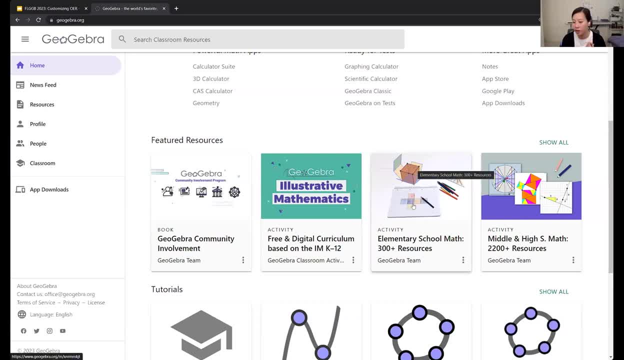 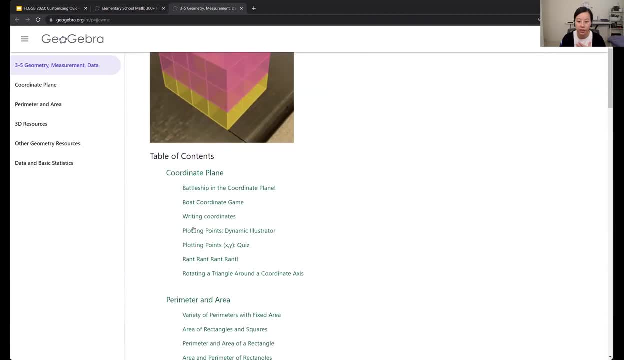 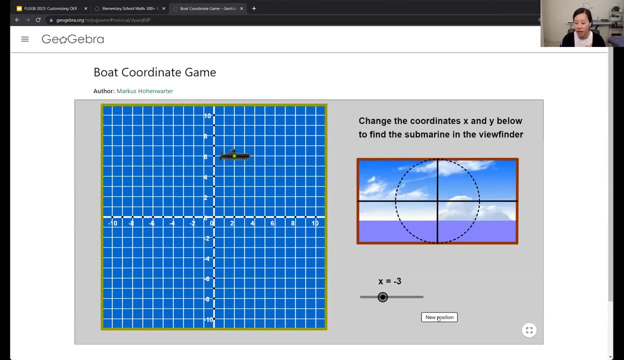 um, maybe, uh, I wanted to look at some elementary school resources and look at this boat coordinate game So I can take a look. I really like this because it's um, so it's a little, it's a game, So maybe I just wanted to include this as a little bit of a. 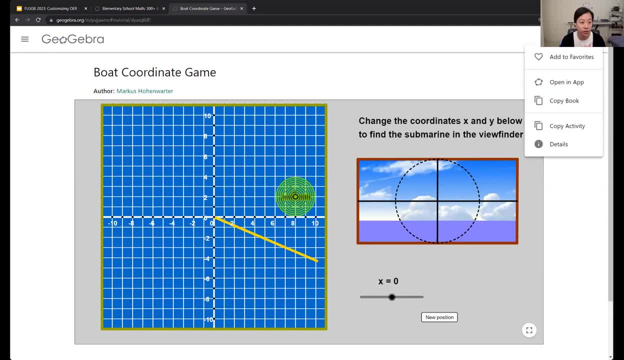 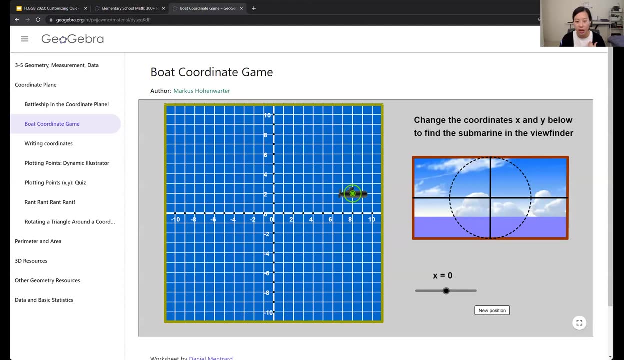 warm-up in my lesson. Something I can do is I can go to the three dots in there right, And I can actually copy this individual activity. So the way that the GeoGebra structure works is a collection of activities is in a book And then each individual resource or page here is an activity. So I can actually 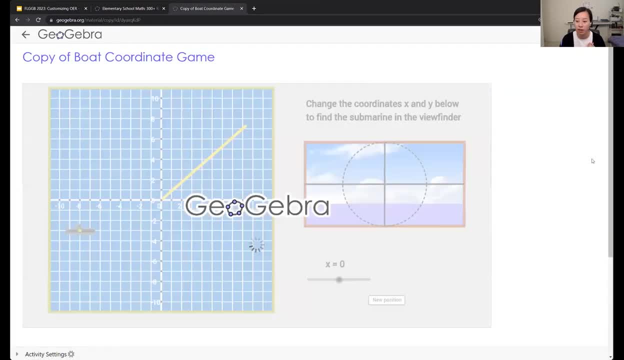 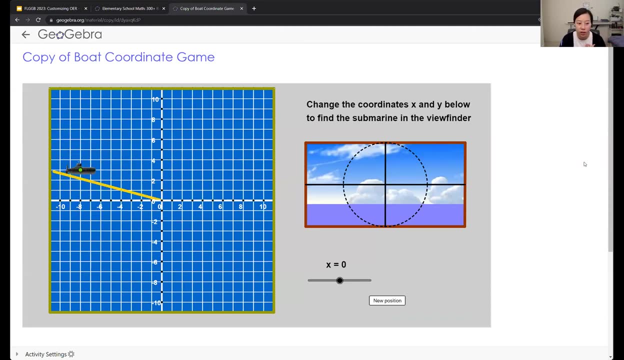 copy this activity myself, Um, and maybe I wanted to uh customize it a little bit So I can actually copy this activity myself. Um, and maybe I wanted to uh customize it for myself and for my own class. One of the ways I can do that is I can just go uh here. So I'm here in this editor mode. 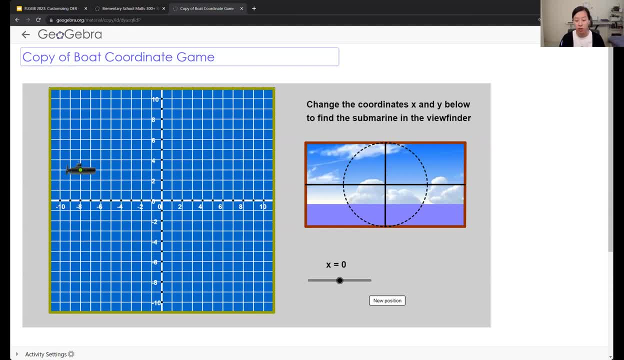 Um, it's me. this is a copy, so you're not going to change the original. So if I made a copy of, like Karen Camp's uh Pythagorean uh exercises, then I can just uh, I don't have to worry that. 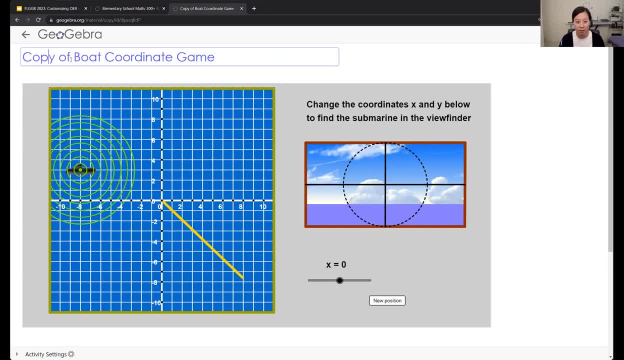 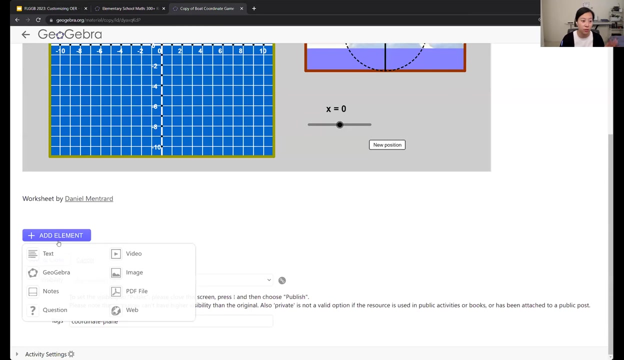 I'm going to mess any of her original up, Um, so maybe I'll write here this game: I can change the title, So maybe I can put like: um, Monique's the first period, Uh, and then I can also, uh, add a few different elements. So maybe I wanted to. 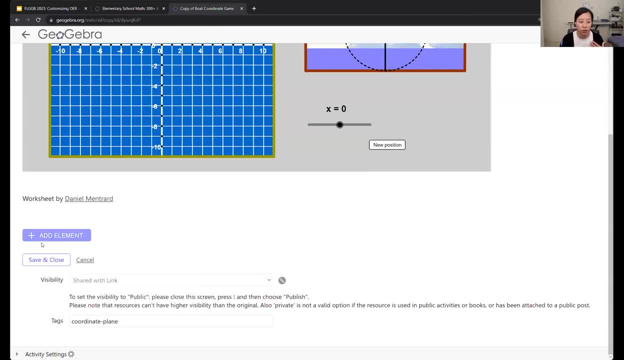 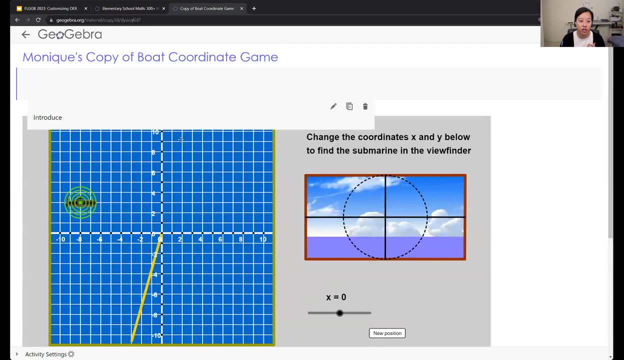 uh, include some text. So this interactive part is really cool, but maybe I want to introduce um, um, um, um, a little bit of an introduction to this So I can add element. I can pick the one I want. 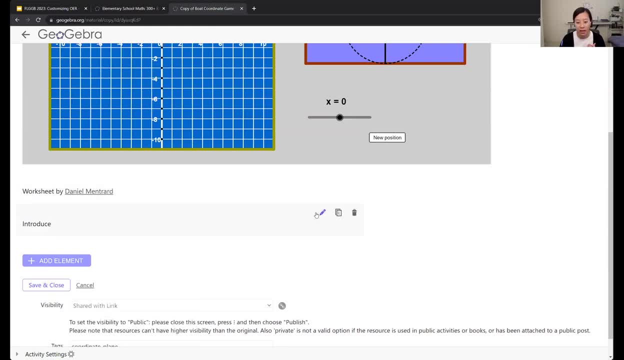 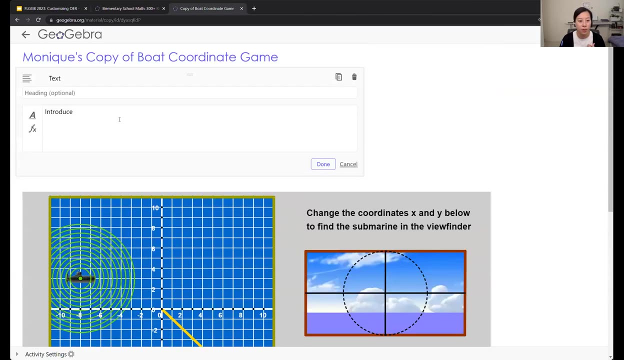 and then it gets added to the very bottom. Um, I can click on the little pencil or click just directly inside: edit it around. Um, I can actually copy each of the elements. I can delete them, And then I can take these and drag it around as well. So maybe I just want to introduce this. 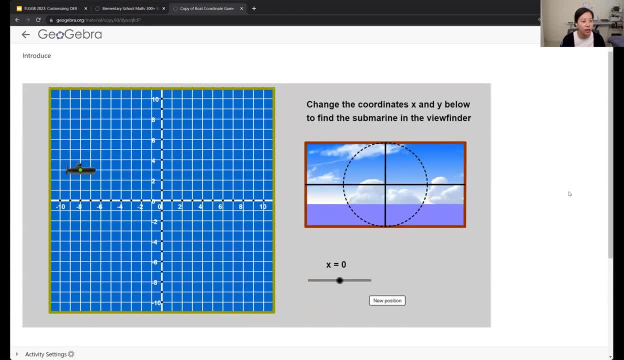 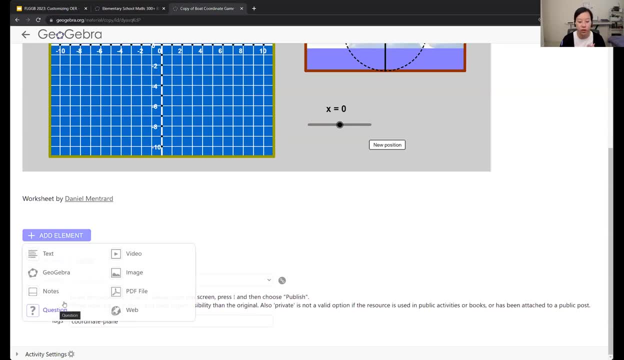 a little bit, maybe a little bit of instructions, Oh like, try dragging the sliders Um, um, um, um, or I can also add a question. So you can also add, like videos, images, PDFs, web links: Um, that will be um. so, if you have something you want to embed, 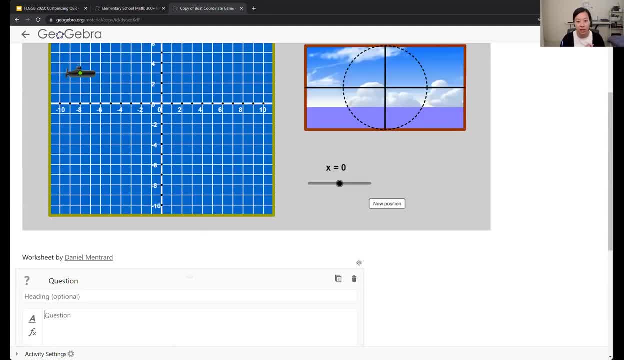 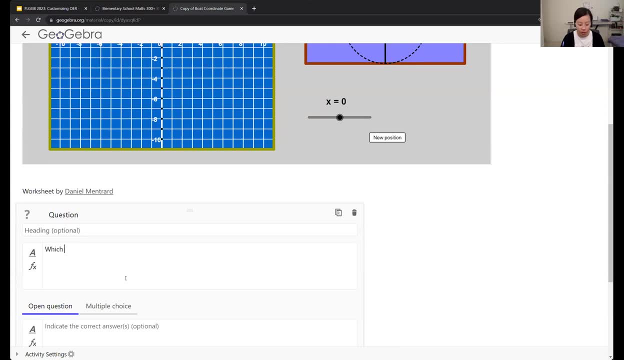 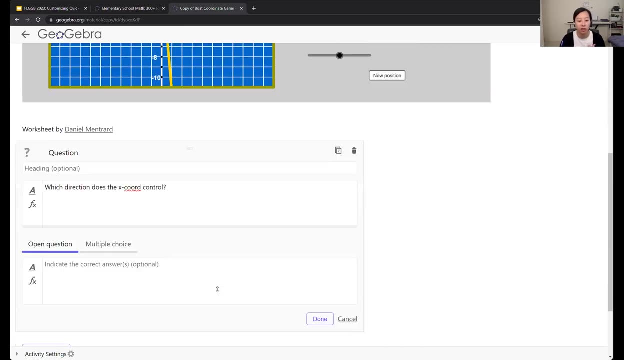 uh, that might be useful, but maybe I want to add a question at the very end, um talking about: okay, like, what's, uh, which direction does the X coordinate, uh, control? um, um, um, um. 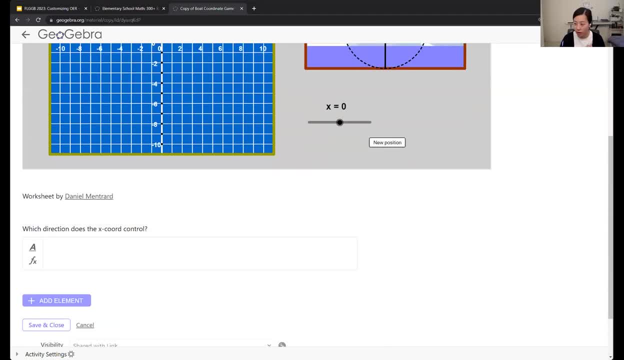 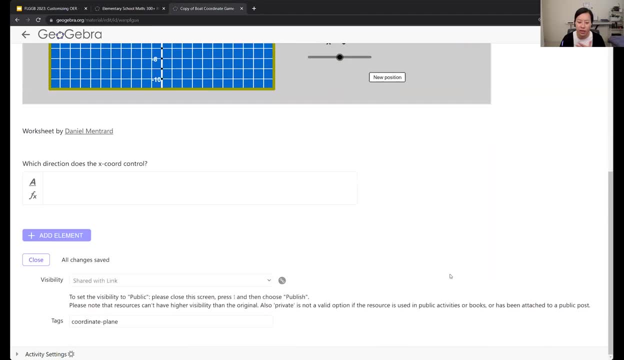 what does that mean? So I'm going to add that here And then I can save everything. This doesn't auto save, which I find personally um useful for if I do a little bit more intensive work. But, um, yeah, you can just close this and then, uh, some extra buttons I wanted to note here. 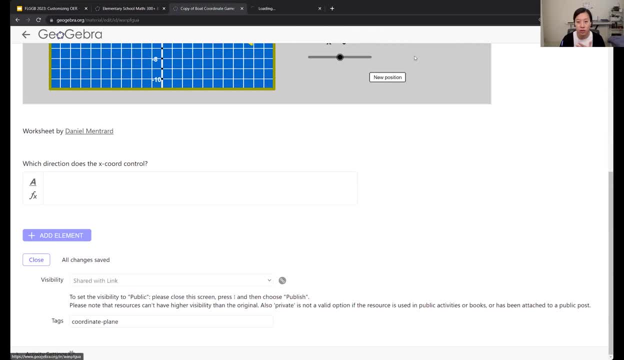 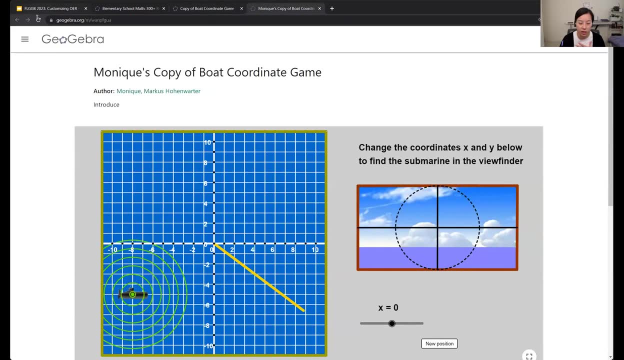 There are- uh. here's the view resource, So I like to open this in a new tab. If I just want to take a peek and look at I'm editing, um, I save it. I want to look side by side. I just refresh the page and check any of the extra changes I might. 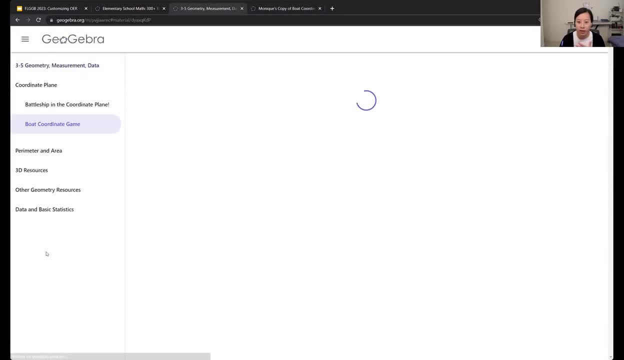 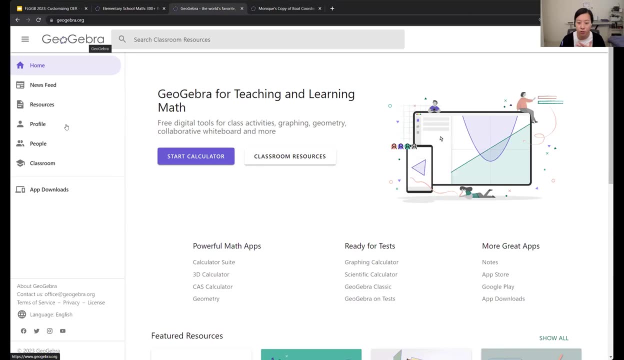 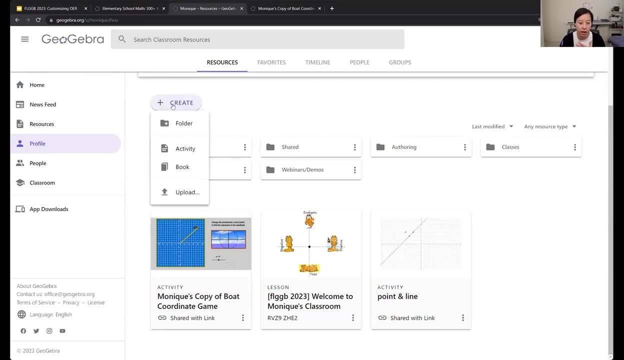 make. But yeah, if I close this, if I want to find what I made, I can just go to the homepage, go to my profile and here is that resource, right here. And of course, from here I can also create folders. like you can see here, I've created some folders. I can create a folder. 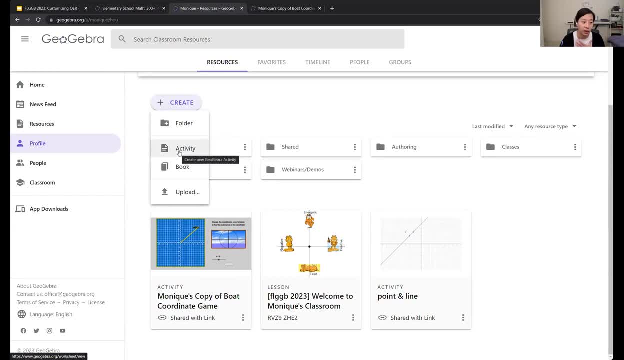 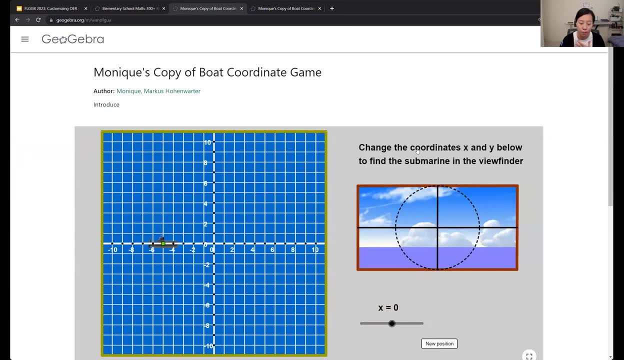 I can also make my own activity if I wanted to. I will go into that a little bit later- Or you can create a book. So, like any of the other resources that you find on the site, you can also just assign this. So if I click this and I kind of hit this Jojoba lesson thing again. 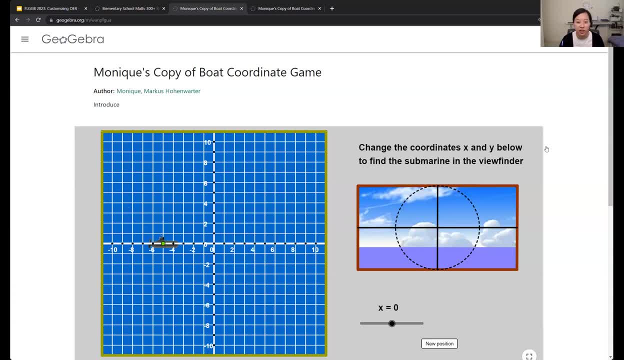 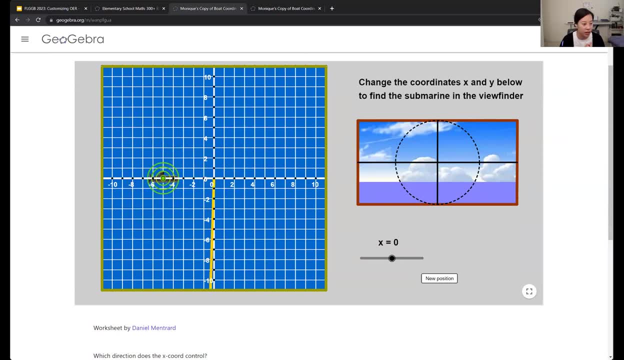 I can create a classroom, I'll get a code, I can send the code and then we can all work on this boat together. All right, So we just talked about the ways that we can retain some of these resources. on Jojoba. 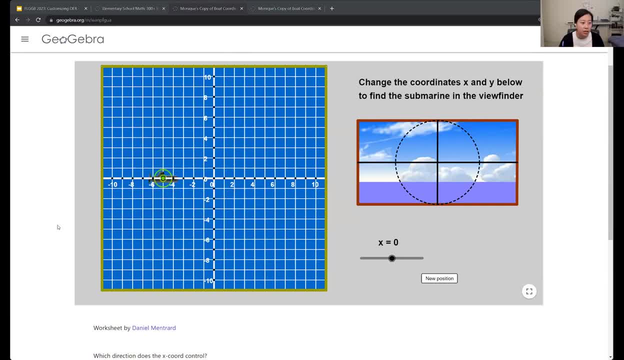 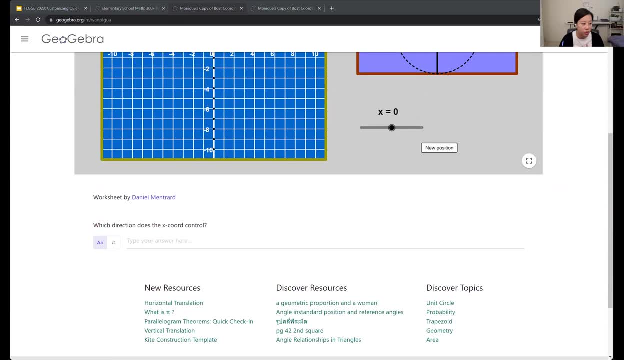 how we can reuse them and use them for various classes, revising them. So I showed you how to make some changes And then next we are going to talk about remixing. All right, So I am just going to check the Q&A really quick in case there's some questions I can. 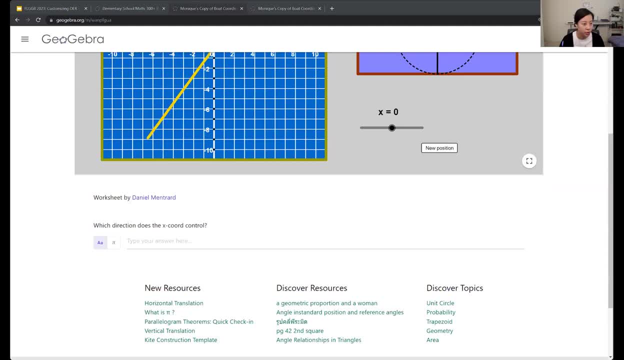 answer here, But it looks like we are good. If you have any questions, you can put them in the Q&A. I will try and pause occasionally and see if there's any questions that are appropriate to answer in this moment, But otherwise I'm going to chug along And of course, these sessions will. 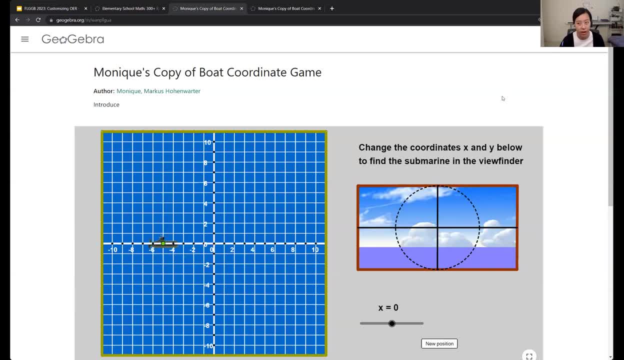 be recorded and they will be posted online after the fact. So I know I'm speaking a little fast. I just want to cover as much ground as I can And then hopefully you can go back and just have me on 0.75 speed or something like that. Okay, So that is just looking at one individual. 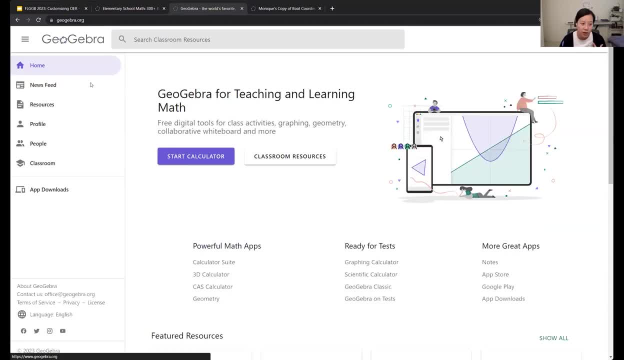 resource, some of the ways that we can change it. Now, I know a lot of you are just busy teachers and there's some things that you- just you don't want to worry about creating or remixing too much, But you do want to. just you know you don't want to, just you know you don't want to, just you. 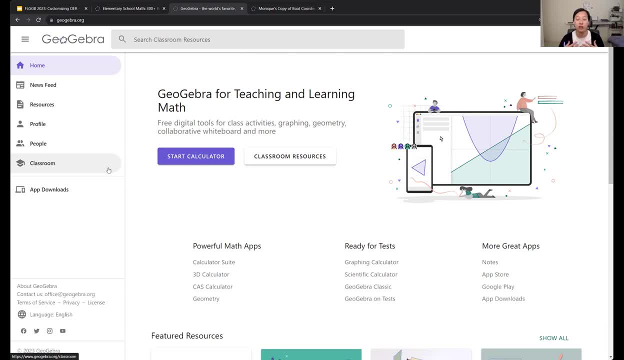 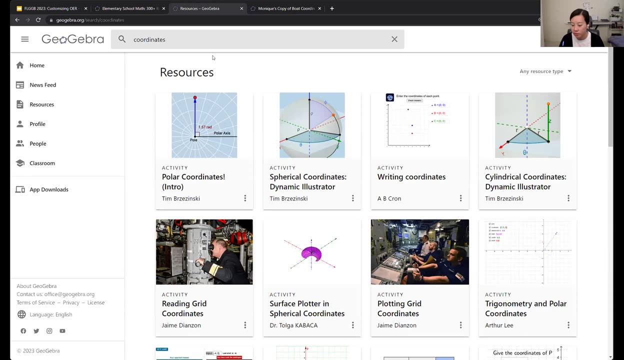 don't want to just collect a bunch of links and maybe assign in GeoGebra classroom, assign an entire set of resources, Like okay, first I wanted to go through, let's look at if I search for coordinates on the site. Yeah, maybe I was with a class and we are talking a little bit. 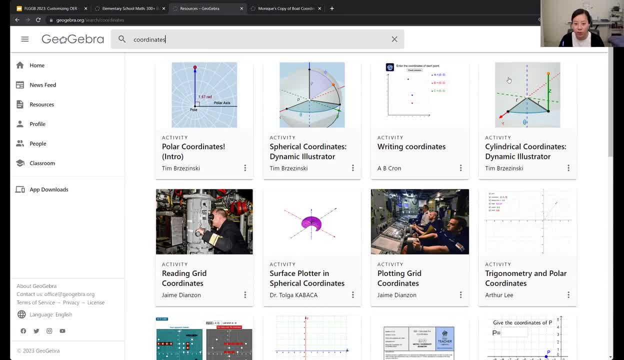 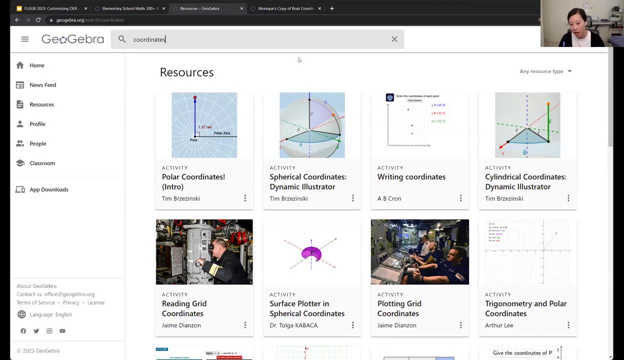 about non-Cartesian coordinates And you want to talk about polar coordinates, spherical coordinates, cylindrical coordinates And maybe I just want to introduce it in one day. Something that we could do is we can actually pull all of these collections ourselves and create. 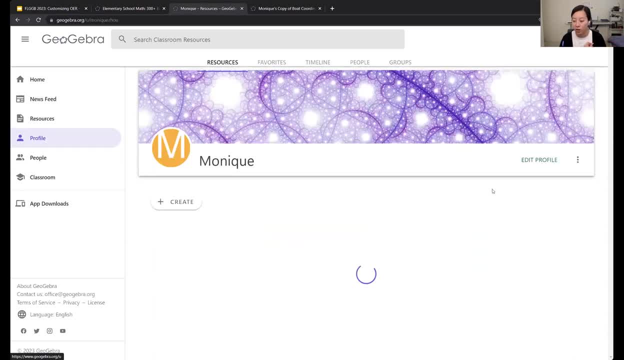 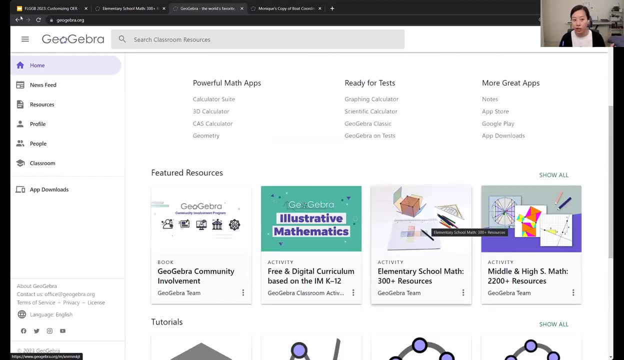 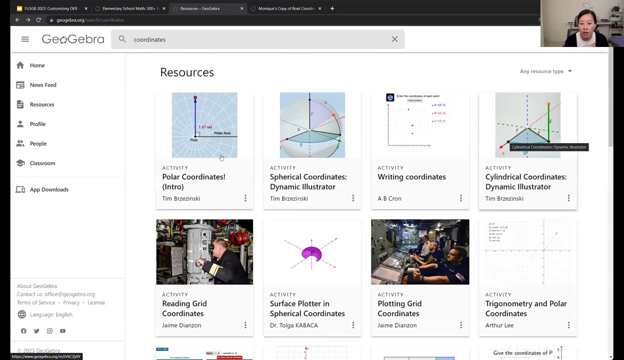 our own book. So on the home page, GeoGebra has created a collection. we have created collections ourselves, but you can also create your own collection. So if I searched for coordinates and I wanted to pull some of these resources, for example, one of the things I like to do is I like 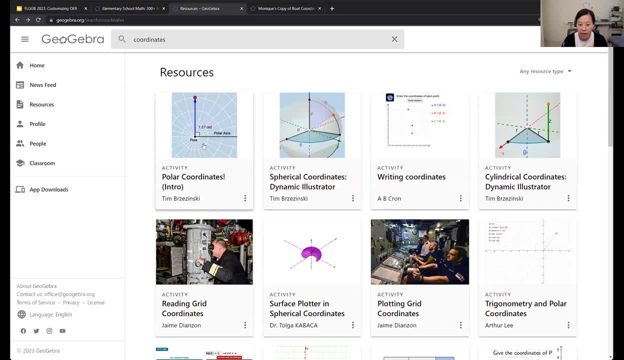 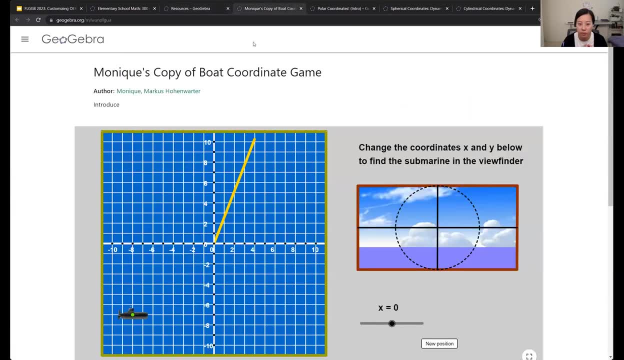 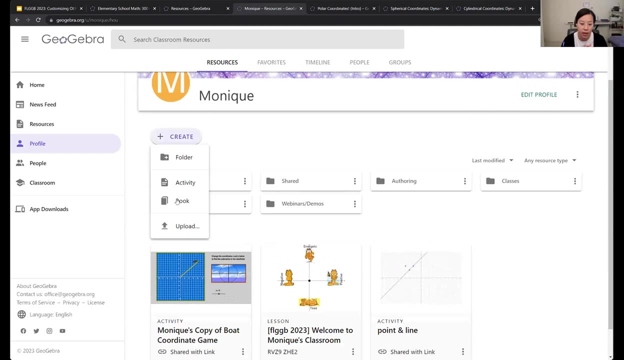 to just open these in a new link. So what I can do is I can just pull some of these resources. I can right click this and open this in a new tab. This is generally how I like to do my workflows. I'm going to go to the home page on this tab, Under profile. what I can do is I can create my own. 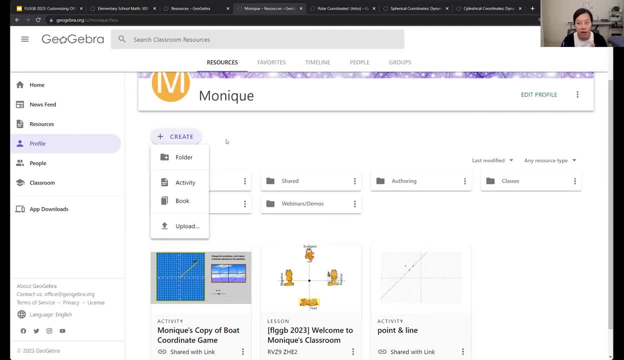 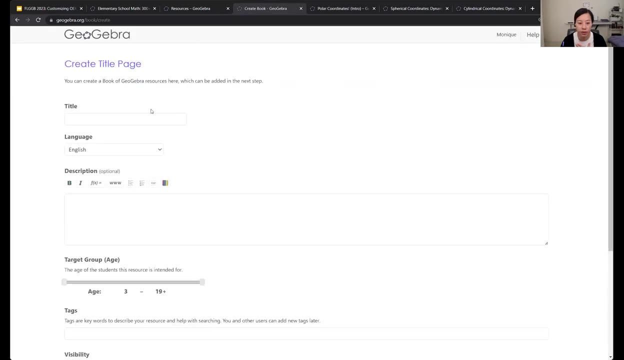 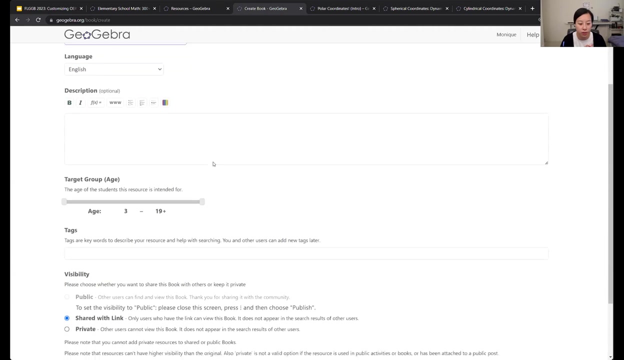 book. So for me personally, the way that my workflows generally work is: I work in my profile a lot So I can click on book. I can create a book, give it a title and then most of the permissions are automatically. 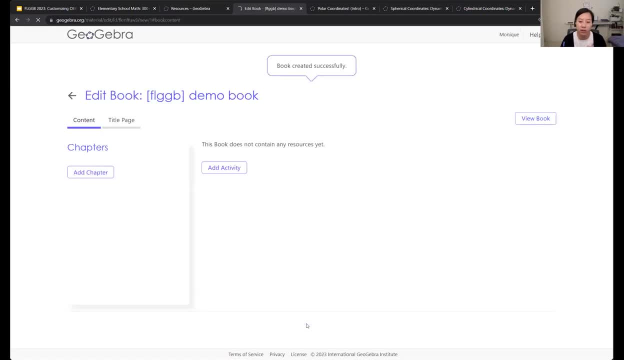 these are usually shared with link, So I'm going to save this So that way you can't search for it on the GeoGebra site, but if you have the link, you can share with someone. they can view it even without an account. But, as you can see, you can create a book. There's a lot of different ways to 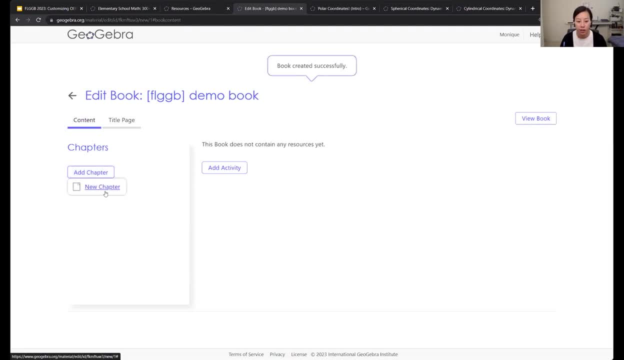 do this. You can add chapters So you can section them off. So maybe there's something for a warm-up that you want to use. Maybe there are some, maybe there's the main content. Maybe you want to add an exit ticket. 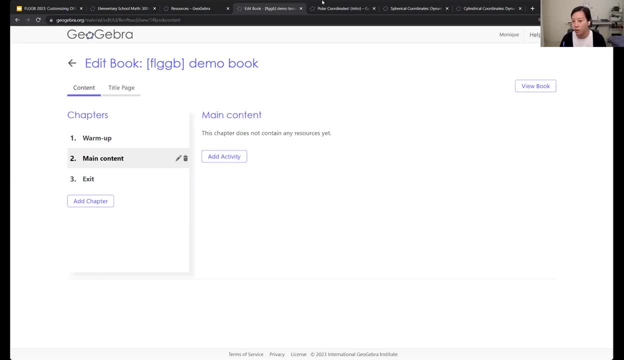 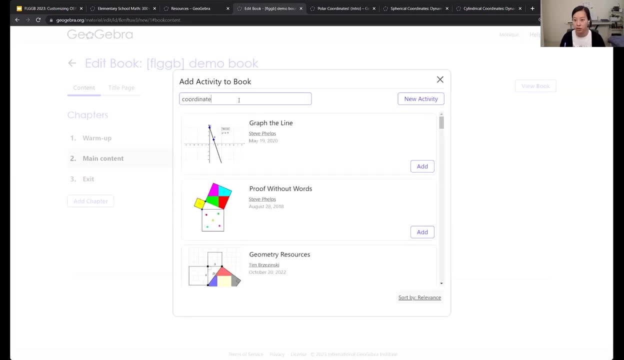 And then what I can do is I can add activity And you can search for this again. I personally don't love to search through here because it's the thumbnails are a little bit small And usually I have the links that I am looking for myself. 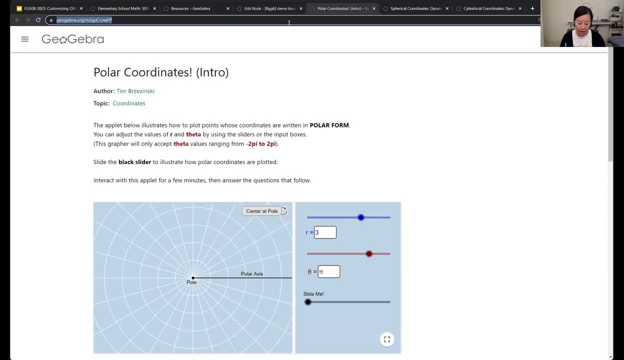 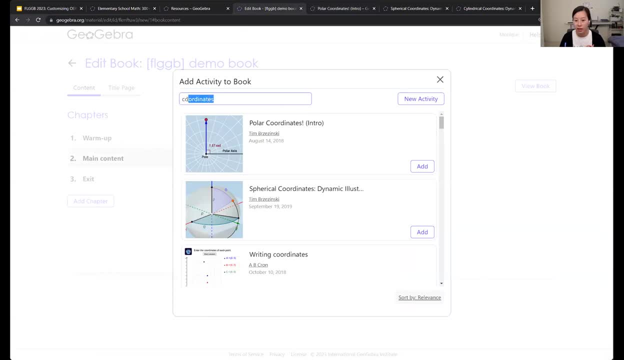 So this link here. So what I personally like to do is I like to copy the link And then I can. so I can. just if I know this is the one I like, I can add it. I can even click here and pop it open in the new tab. 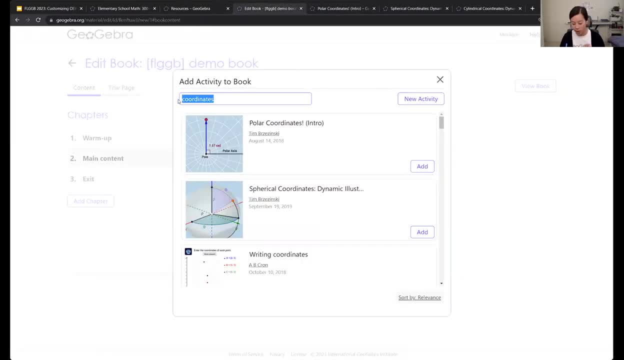 and see: oh, this is the one that I was looking for. But I personally like to just paste the link where I found it. The way that GeoGebra reads this link is it reads the last eight digits of this code. So what I will also do is I will just when I go to the link. 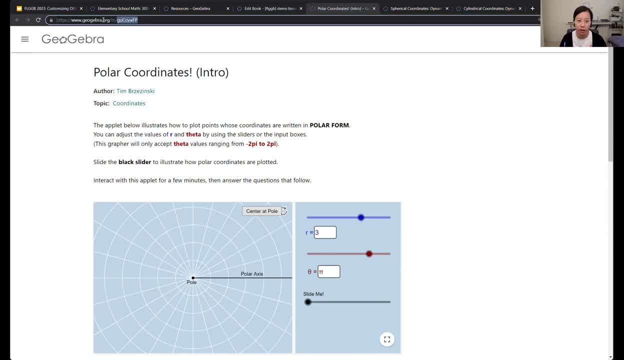 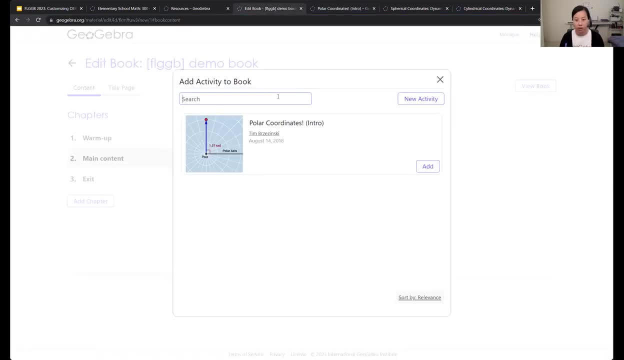 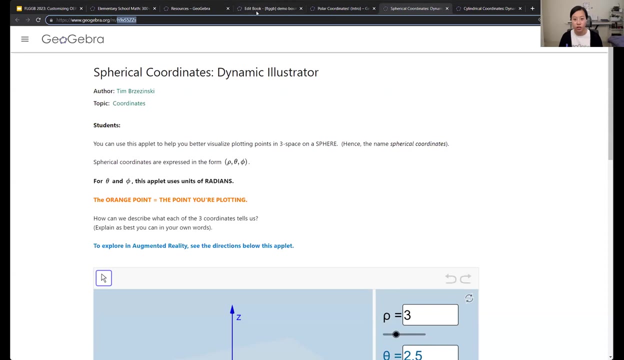 I will just double-click on the very end of the URL and it will automatically only highlight that code. So I can copy that code and I can just here go. Let's try a different one so you can actually see it change. 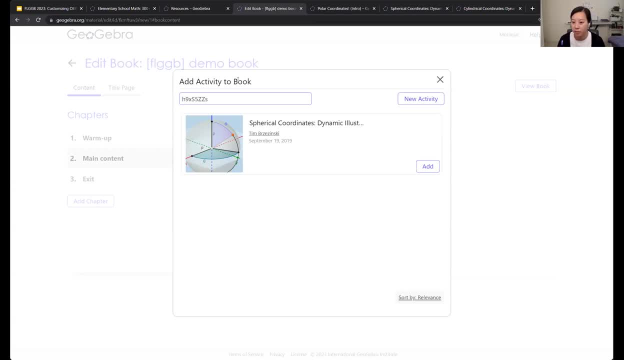 There And then the code just pops up. So I can add this here And it's under main content. I can add this one here. I can also rearrange it, So maybe I'll just move one up. There you go. 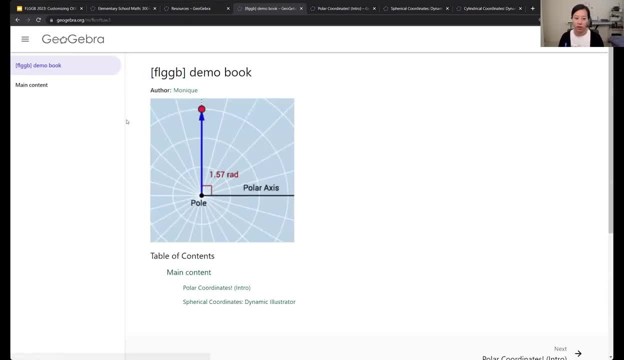 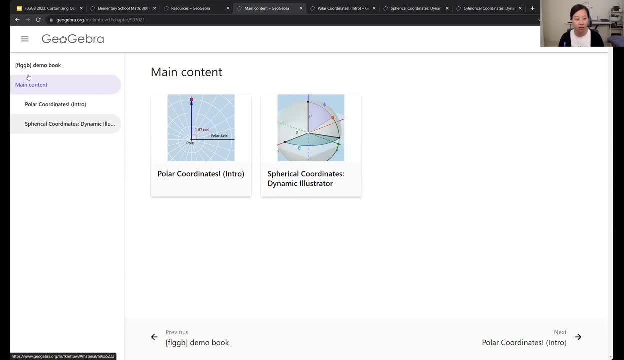 And then maybe I'll just view the book and see what it all looks like. So what it does is, if there's nothing in the particular chapters, it will hide it On the left side, So that way you don't see. oh, I had like a warm-up ready or I had an exit ticket ready, but I'm going to insert it later. 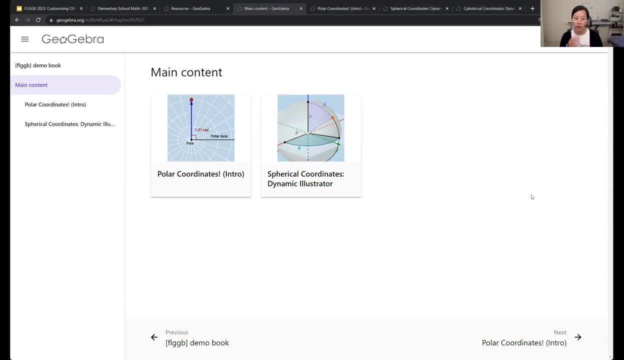 So this is another way that you can save resources and kind of incorporate into your workflow, especially if you work in different teams or you want to use, create collections of things over the course of, say, an entire year. Also another thing that I use on my website: 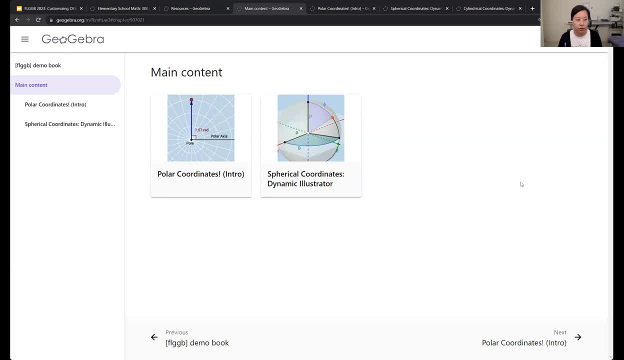 So if I go to my website, Another thing that I use on my team is: if we're trying to both work on, I'm with a teammate, we're trying to work on the same book together and really pool together resources together. One thing you can do is have a shared account. 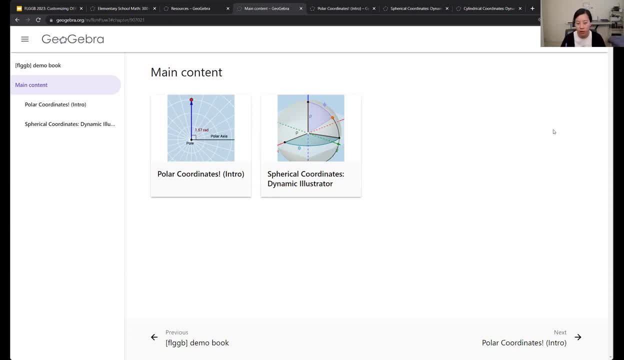 So maybe there's one particular account that you use for your team or your department. But another thing you can do is if you have your own separate GeoGebra accounts. So you can go to the menu on the top right And you can go to details. 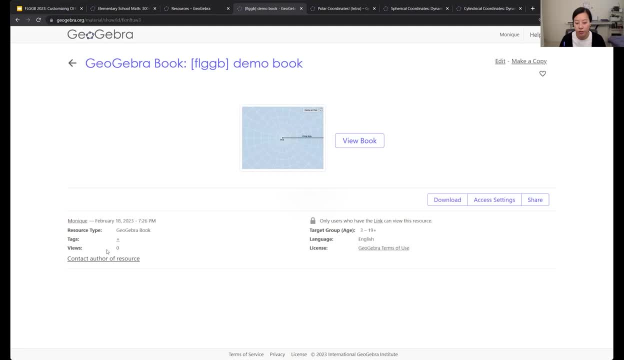 So, whether it's a book, whether it's activity, you can go to details. You can look at a bunch of the details here And I like to go to access settings. You can see it's shared with the link right now. 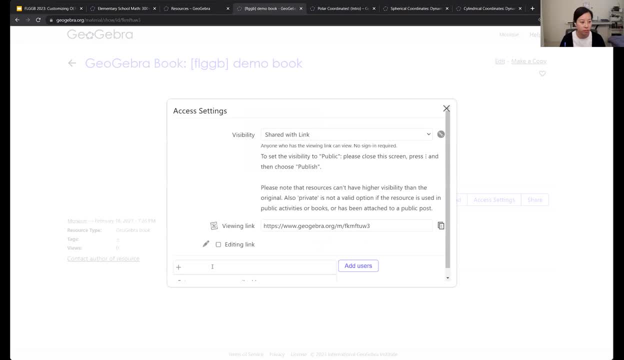 There's the viewing link, But I can actually just add users here, So maybe there's one particular person I want to add, Or what I can do is check this- And this is an editing link, So that your colleague can also. just you know, you copy this link, you paste it and you send it to them and they can work on it. 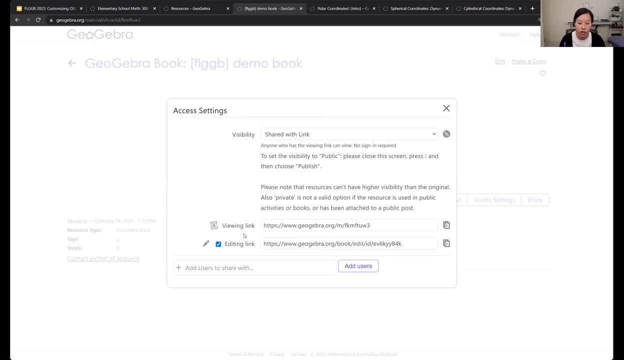 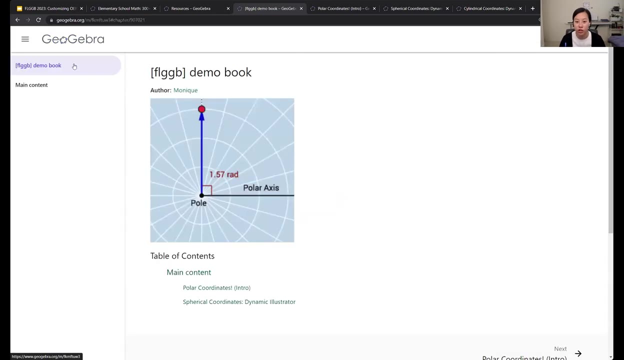 Then, when you're done, you have some demonstration to do or something like that- you can uncheck And then that way only you can edit this again. So just a few little helpful tips, In case you wanted to just use GeoGebra a little bit more intensely. 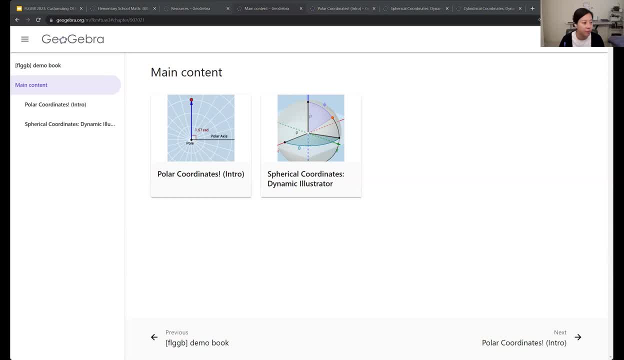 Okay, So that is some of the just mechanics of things you can do to save and edit and play around with some of those resources. And now something I wanted to just show and just encourage is the using GeoGebra very differently in the ways that you might expect. 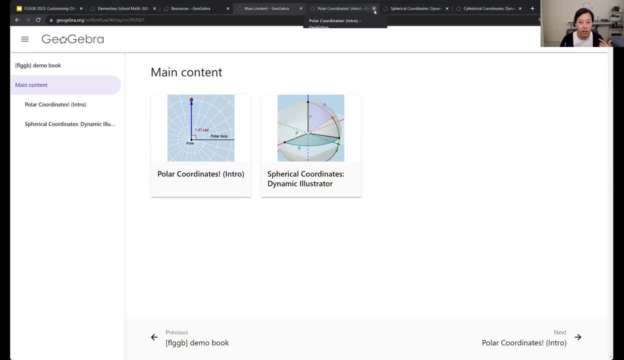 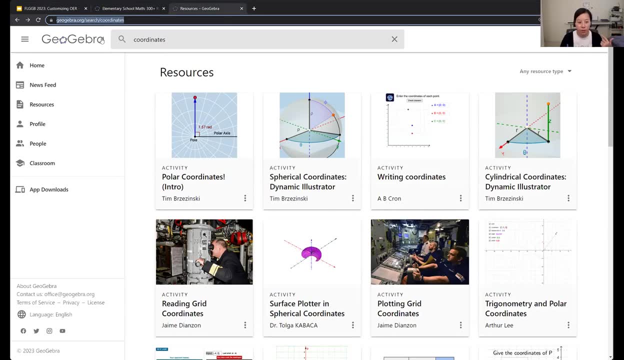 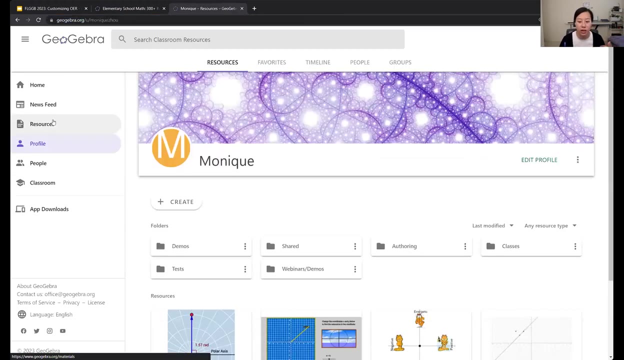 So I will just talk about how GeoGebra could be. You might think that you could use GeoGebra, And then the ways that you can kind of elevate, Using the resources that's already created. So let's just go to. 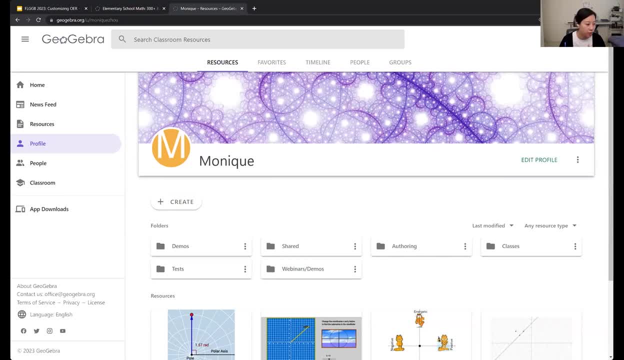 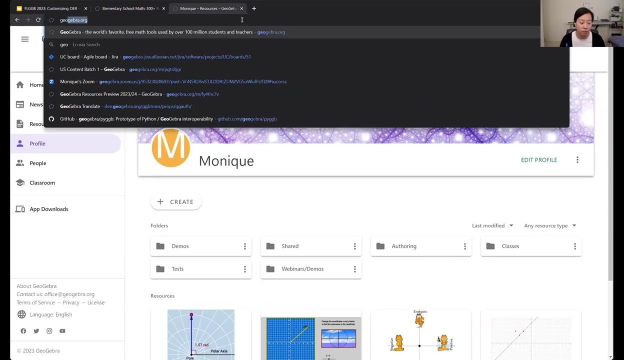 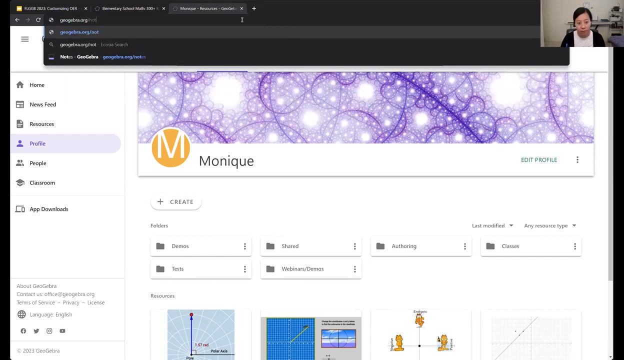 Here And I will look for. Let's see, Something I can do is- maybe Here's an example of: I have A, I saw a PDF online and I'm Let's, for example, say that I am Working with an elementary class right now. 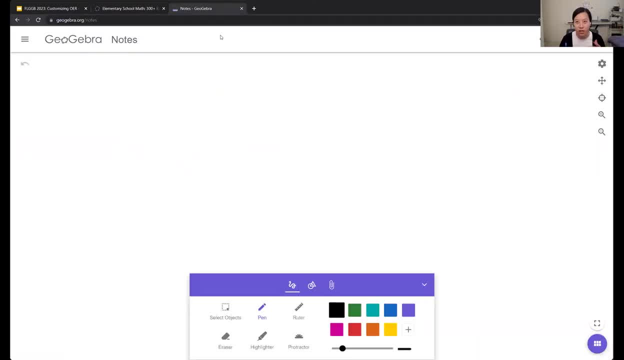 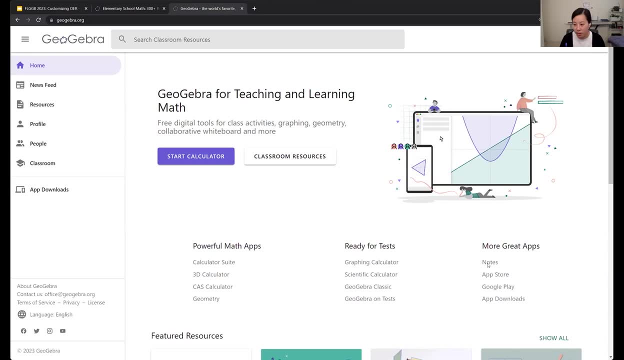 And I might go to GeoGebra notes and let me- sorry, let me back up a little bit. Let's say I'm on the homepage of GeoGebra. One of the things I can do is I can access notes, Which is basically a whiteboard where you can place a lot of things. 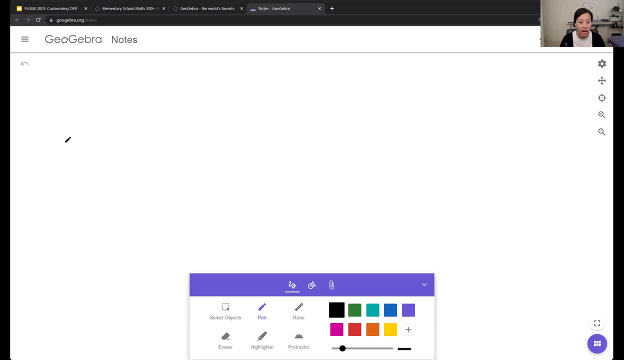 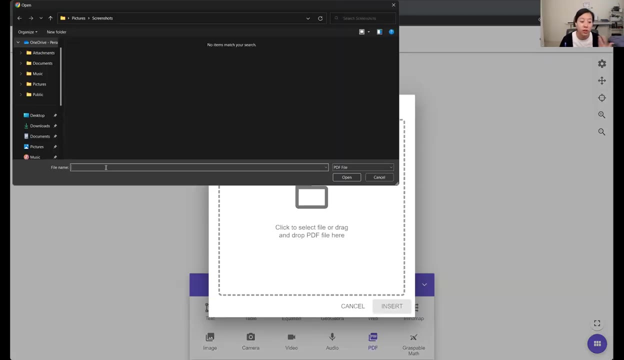 You can actually. You can actually save these and embed them Into activities, But for now I'll just show. I might've seen a PDF of something I was working on With Or I was going to use for skip counting, So let me. 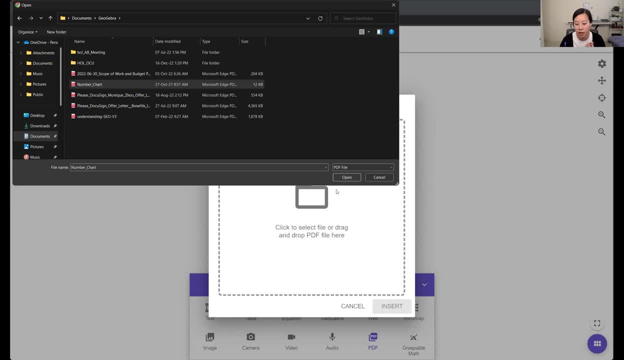 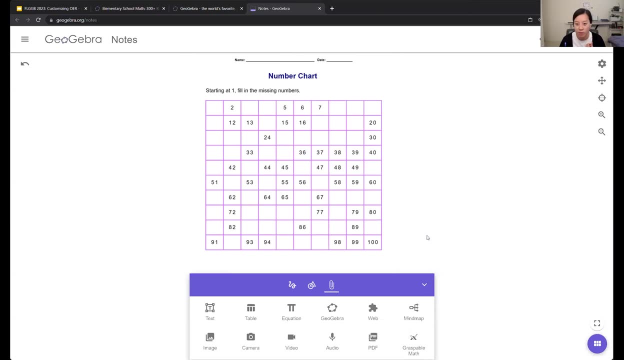 Find Here. So here's an example of a worksheet for a number chart. It's just like a hundreds grid. And then something I can do is I can Save this, I can share it with My students, I can have them just use the little. 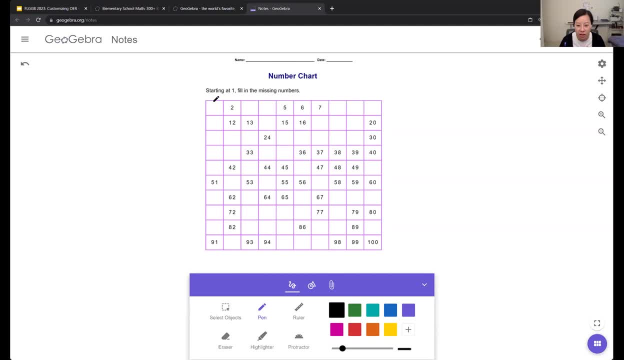 The pen tool and fill it out Like this. I can do something like that, But this worksheet has like a one-time use. There is a. it's a little bit of a hassle to Get them to draw on it digitally, So 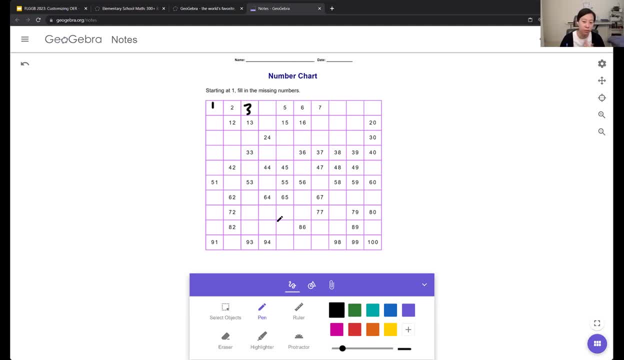 I'm going to show you how to do that. I'm going to show you how to do it digitally. My preference for something like this is just to Print it out, but that's Can get difficult If you have to distribute this online. 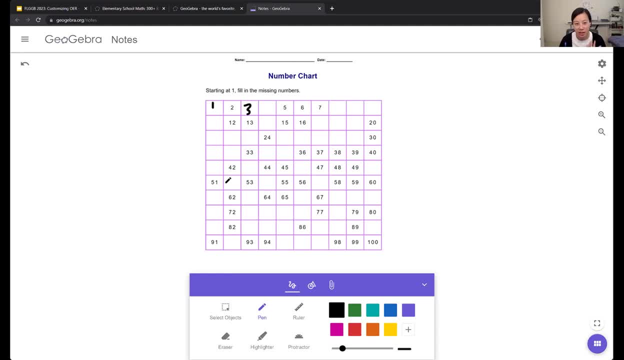 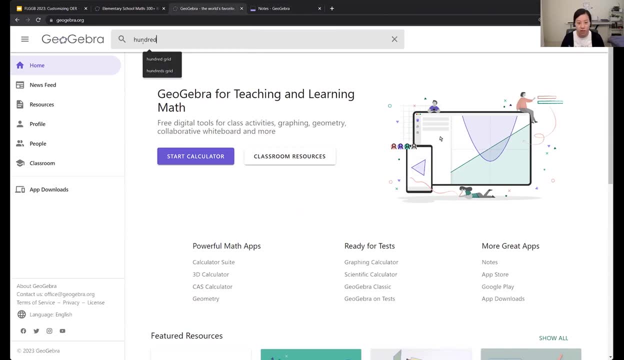 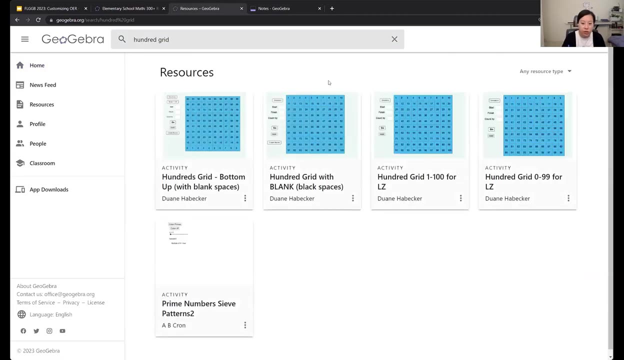 Printing paper costs a lot of money These days. So something that I would actually encourage you to is, If you go to Geogebra, you go search, search for a hundreds Grid And then you'll see some resources for just hundreds of goods that you 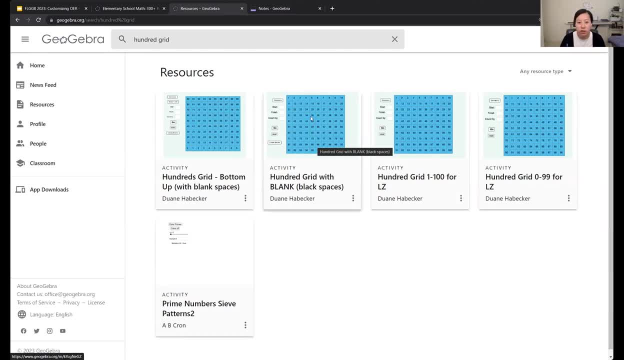 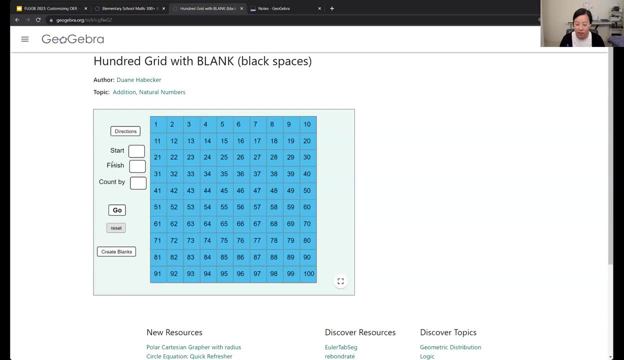 can use. So maybe like, Well, let's do this one. So here's something that I'm going to have bigger made, And Sometimes you can just share this link Or share this with George of a classroom and just say: 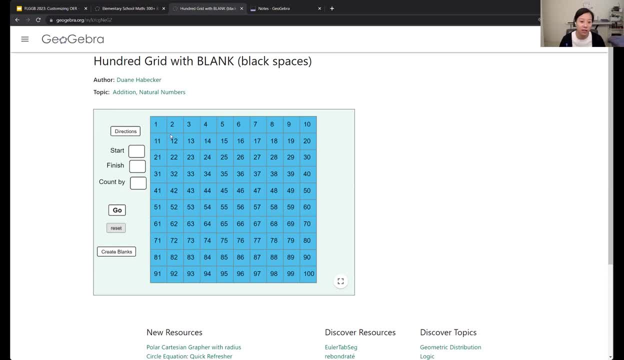 Don't give too many instructions And just If the students ask What do I do, And then You can say what can you do with this, Like, what are some? what can you interact with What? what? How can you make this change? 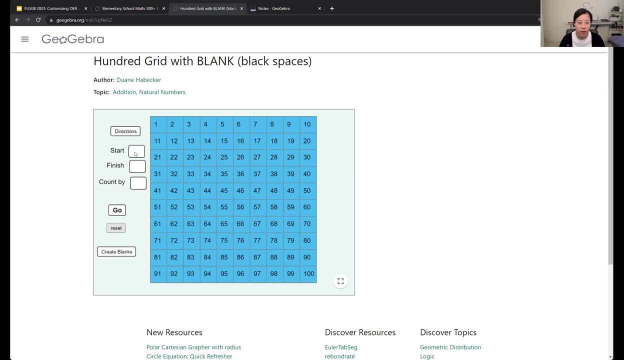 So maybe they'll click on a button and they'll see some, some directions pop up. I'm a little bit hidden. Maybe they'll try and click on the squares and they'll notice that they change colors. Maybe they try and put some. 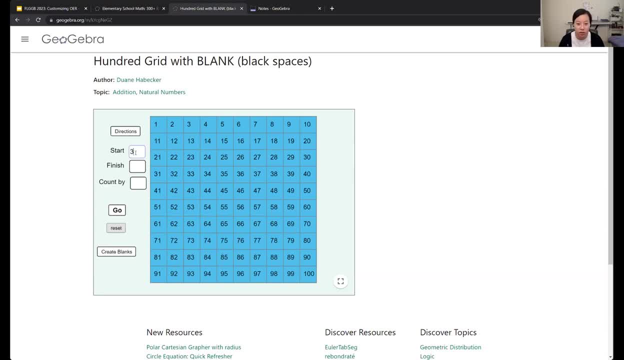 they notice that you can input something in these input boxes, So Do that. Hmm, Okay, That's interesting. Okay, That resets that. Oh, interesting, So I can create this button and it'll randomly pick Which ones are blank. 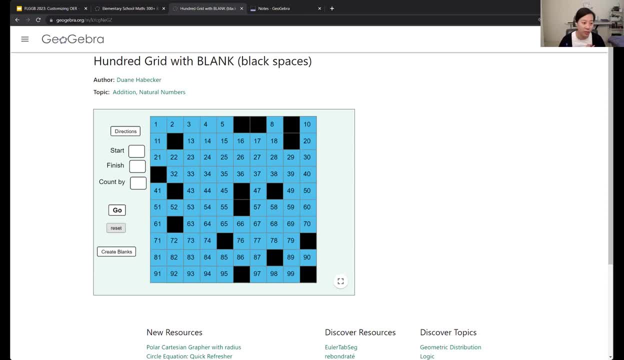 All right. So I really like this resource And I can, I can, I can use it, So I can use it in my activity. But how can I use it and really remix it for the purposes that I like to get into? 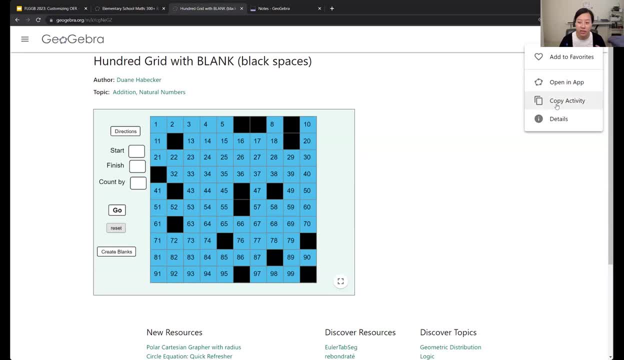 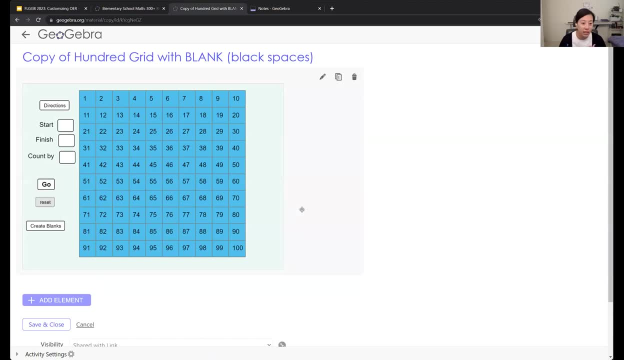 Something I can do is make a copy, So I can copy this activity As it is right now. There you go And let me save this, And so this particular applet in this activity, I can make a copy of it. 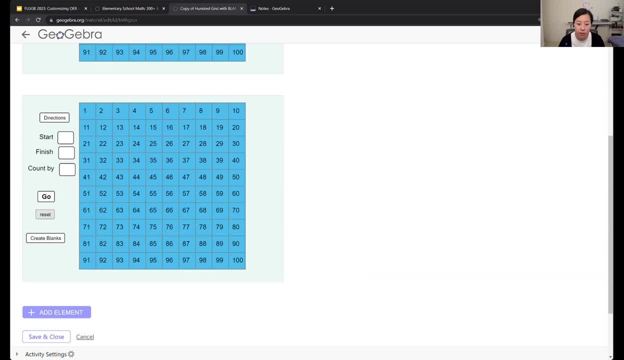 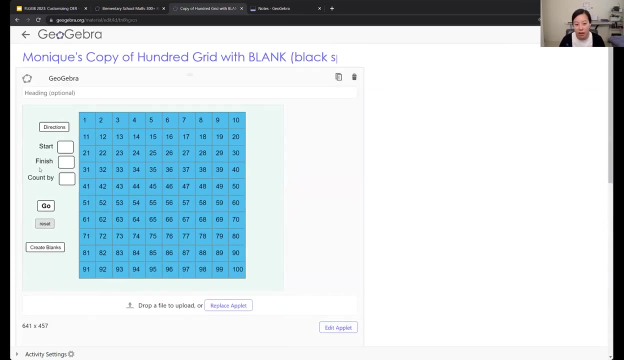 And I can actually. what I can do is I will save it And I can show you just the different ways that I customize each of these So I can make copies and customize it. So what I might do is I click here and I can actually save this in a different state. 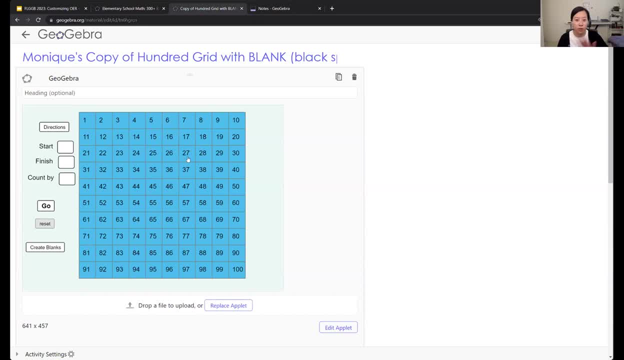 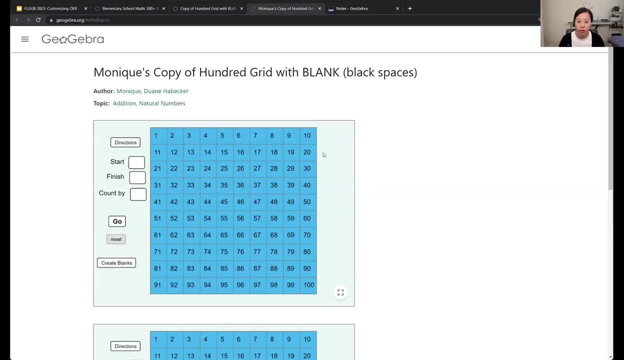 So right now, this is what it is just initialized At the very beginning. when you open this link here, I'm going to open what this looks like in a new tab. So right now it opens like this and this is what it looks like: reset. 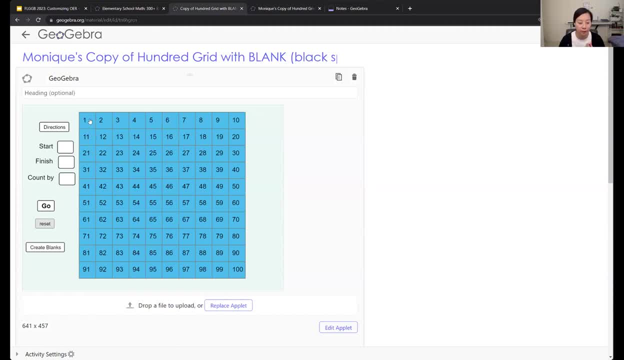 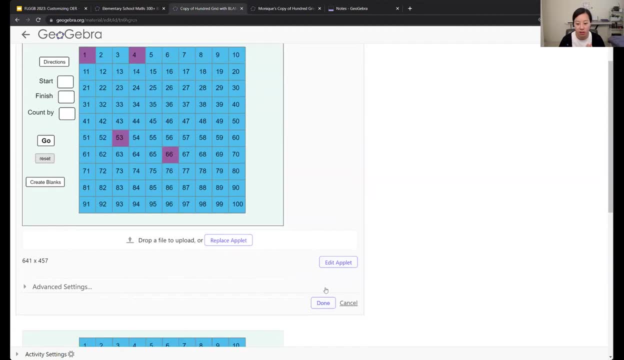 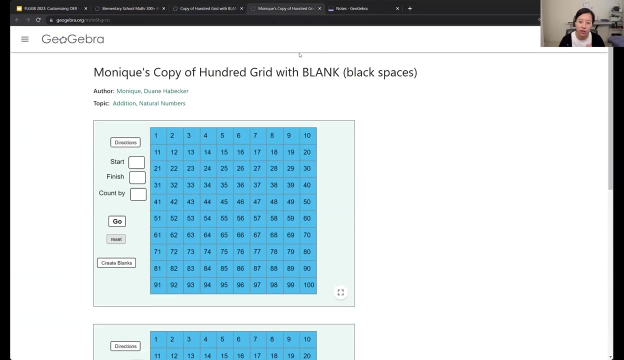 But what I can also do is I can say, okay, change some of these like this and hit done. I can hit save. Go to this new copy of the link. So this is my copy of the resource. You can see there's two of them. 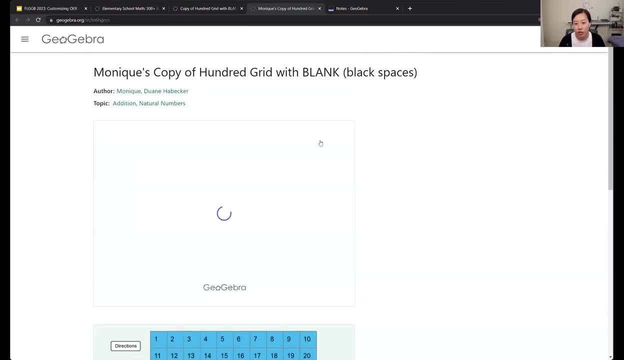 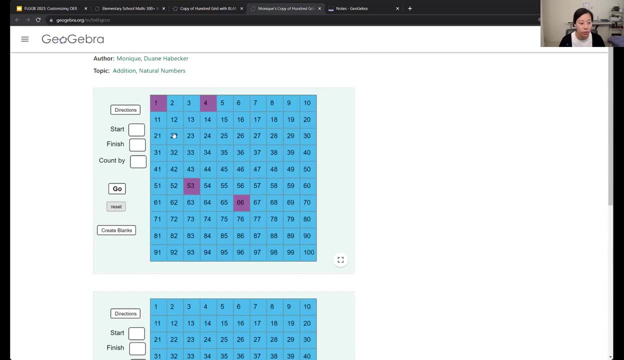 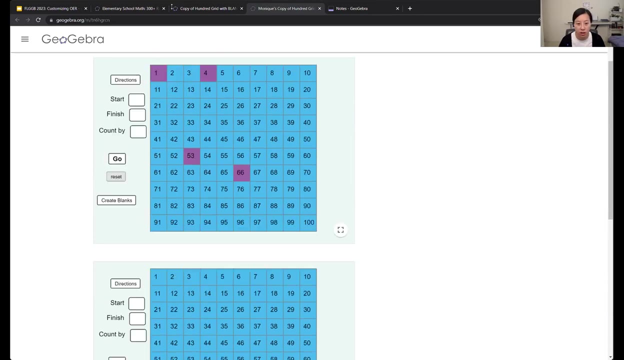 I'm going to refresh the page So you'll see that this is the original. It resets, And then this one Is what it looks like with that new save state, And so this can you can get creative with it, You can have students. 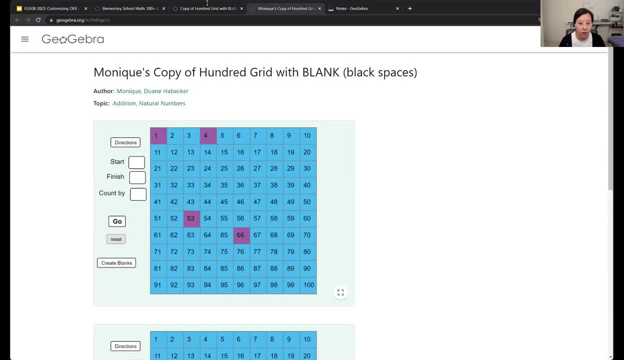 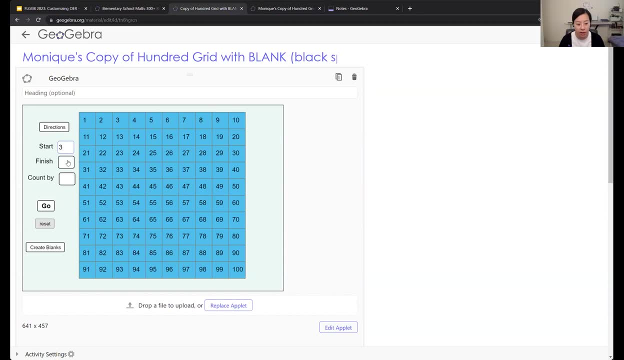 You can select all the boxes, So maybe an example is I'll reset this. I want to start at three and I want to finish at 99.. Count by threes Go. I can just Make some of these Back to the original color. 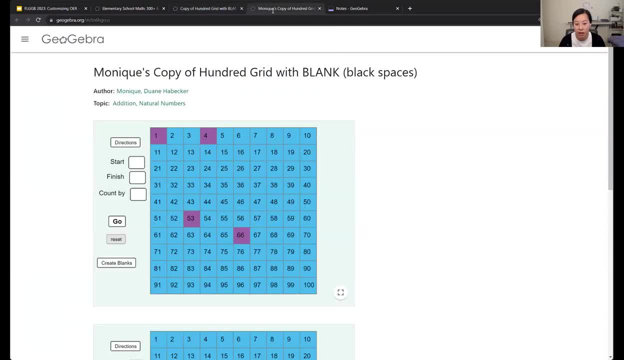 Save it And I can do more of the boxes. but I can say have students Add some instructions that say, hey, can you Fill in like: are there any squares that are not the correct color for skip counting like this: 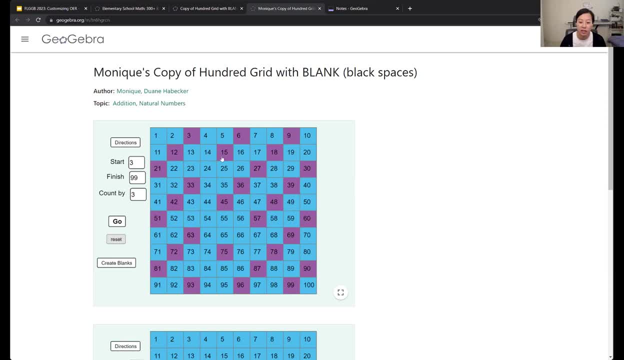 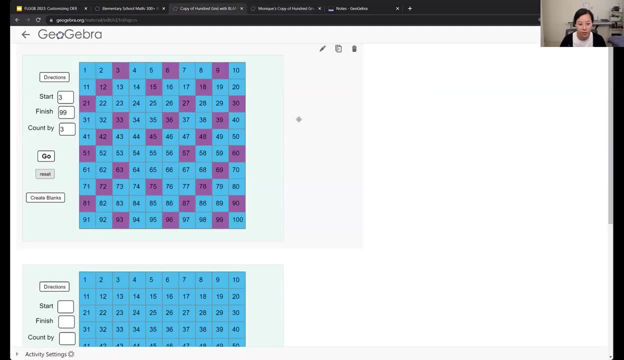 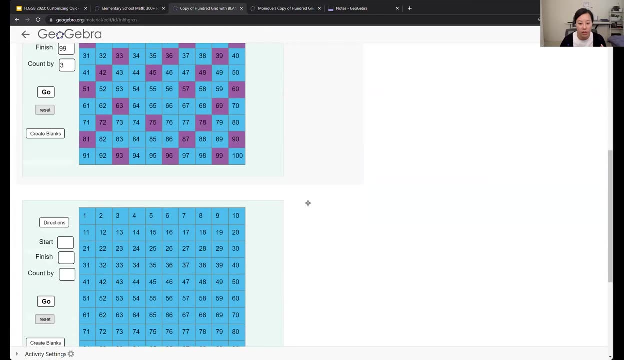 And you can have them figure out how to Click and Click them to the appropriate color If you wanted to. here let me make a copy of this, For maybe the actually let me make a copy of this blank one. 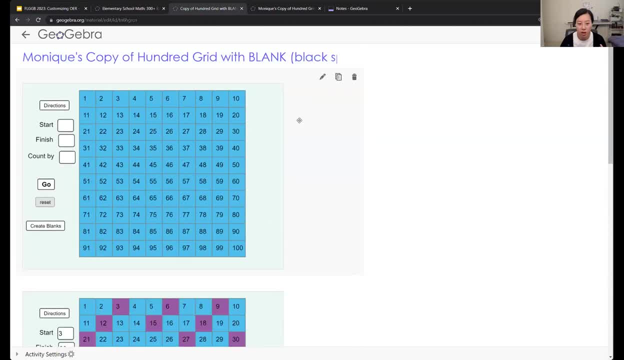 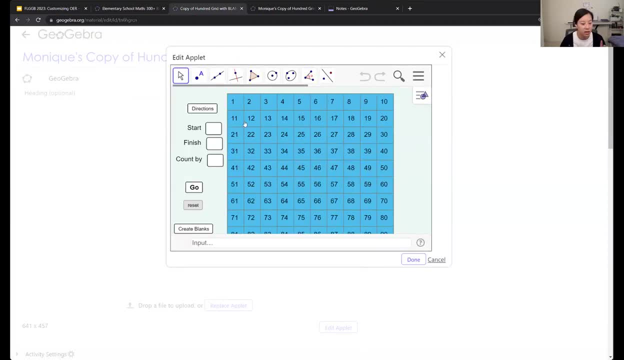 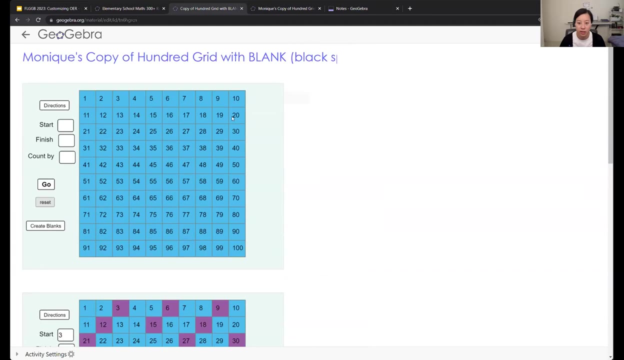 And bring this to the top. What I can do is I can have The. oh sorry, I did not show how I did that, So I clicked on the applet. So it looked like this. I clicked on it And what I can do is I can go to this button: edit applet. 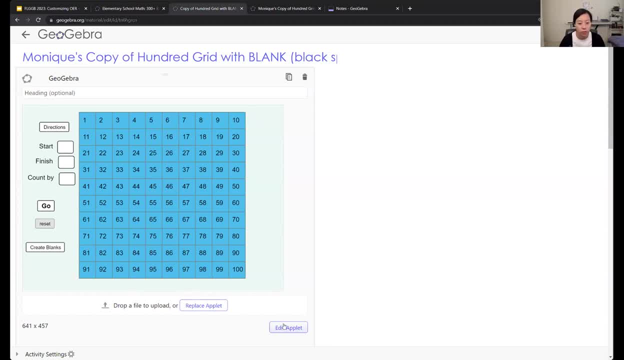 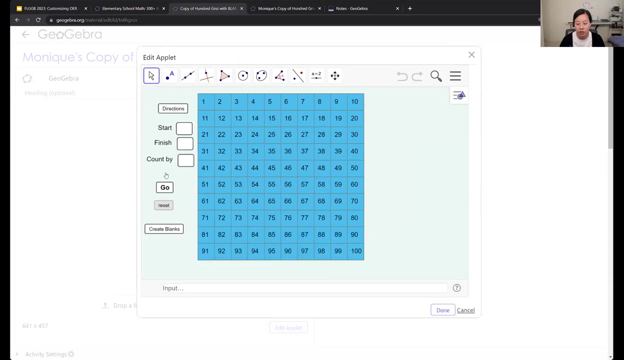 And if you are an avid user of Geogebra and you really know how to use Geogebra classic and create your own resources, you'll be very familiar with this. But if you're not, do not be alarmed. You can click on edit applet and you'll see a bunch of tools at the top and a bunch of menus. 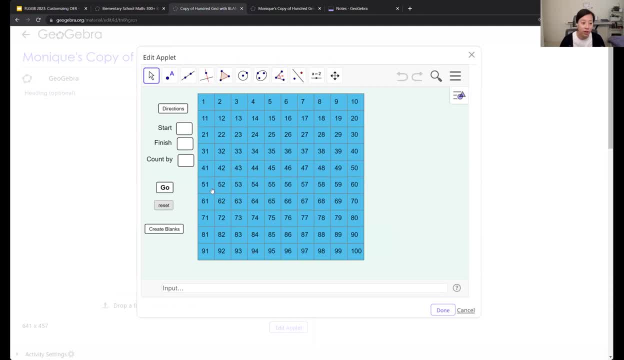 You do not need to know everything about Geogebra in order to be able to use it. Okay, So let's go ahead and start customizing this a little bit more, The ways that I recommend people. just get started into customizing a little bit. each of the individual applets is just hiding elements. 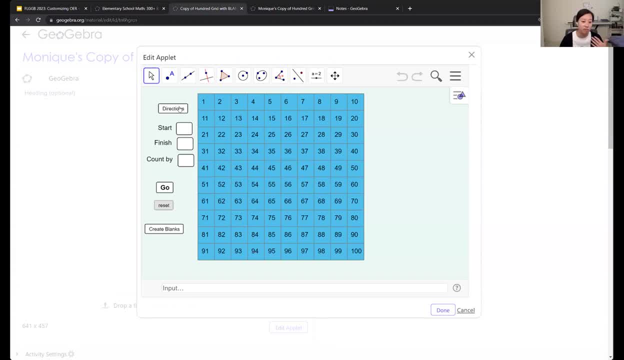 So, for example, here's the directions button. Maybe I want to have the students explore what these buttons and these input boxes and these squares do by themselves, So I might right click here on the button and this menu pops up. I'm going to uncheck show object. 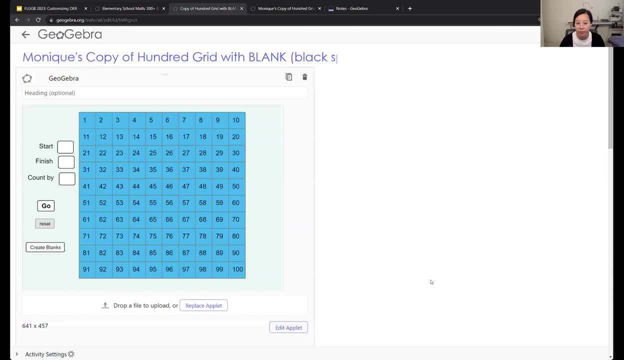 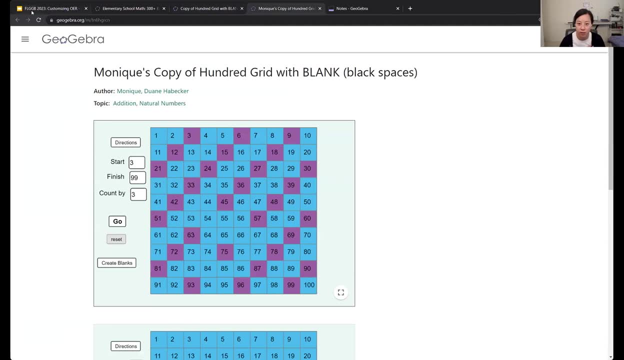 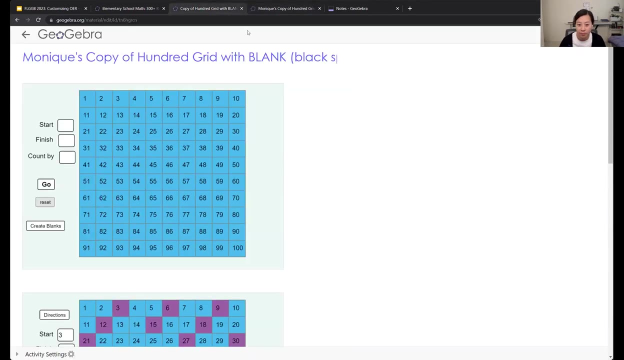 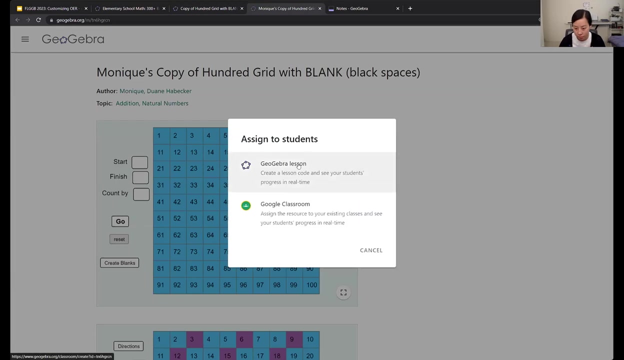 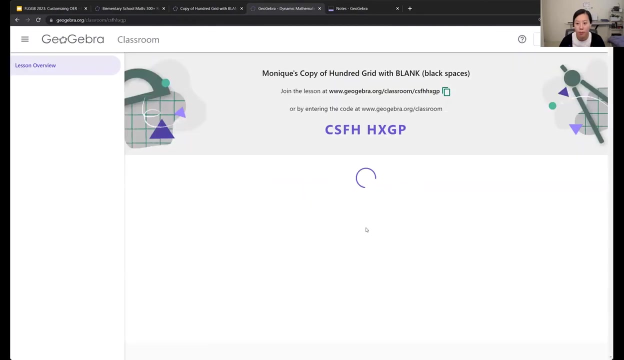 There we go, And then I might save this as is, And I might save it like that. They're refreshed. There we go. Something I also wanted to show is I can assign this to you. Let's see In this classroom. 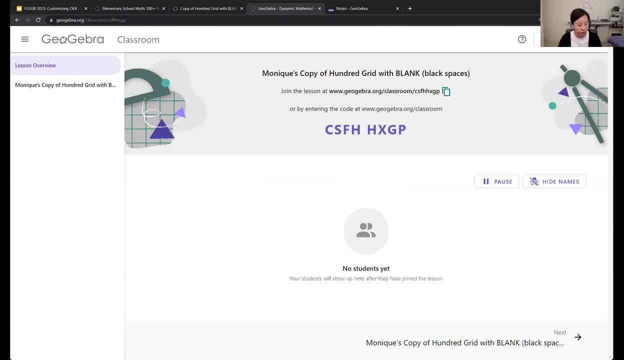 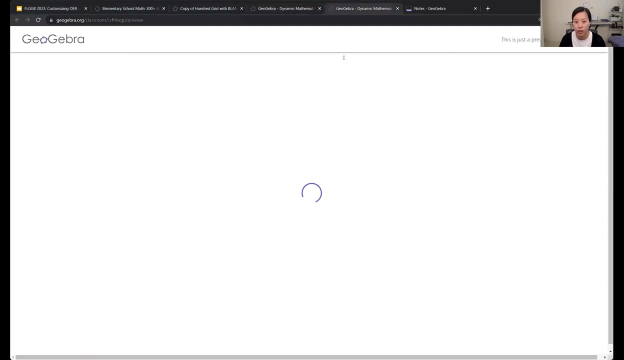 Then why don't I copy and paste the link here And then, hopefully, someone can share that with the general public? Um, but you can also just go to Geogebraorg slash classroom and type in this code: Um, but what you will see is I'm going to open a student's view of this. 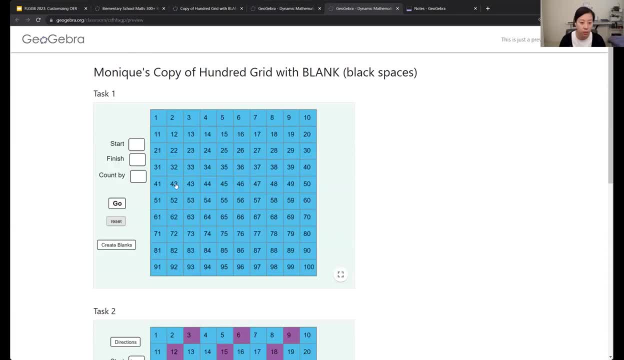 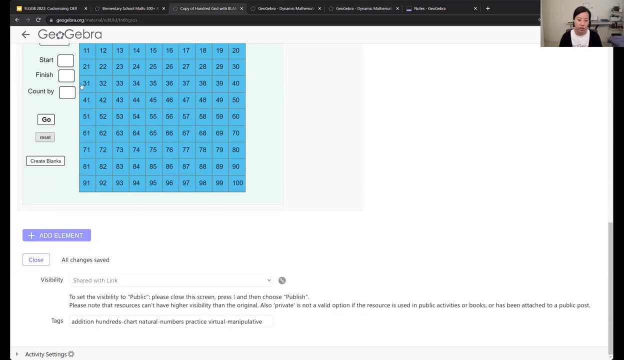 So if the student joins the classroom right now, they'll see one, two, three tasks. First one doesn't have the directions. What I can also do is maybe I add a question. So underneath everything, I'm going to add a question, even after I've distributed it. 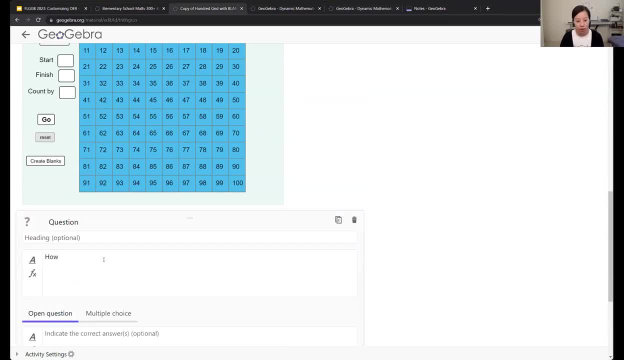 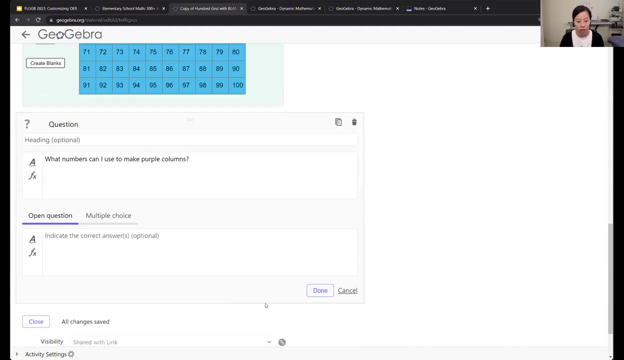 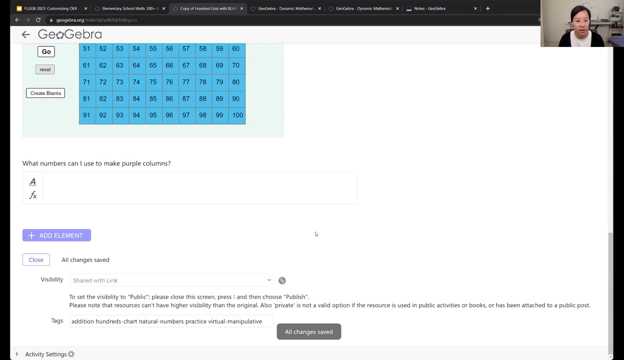 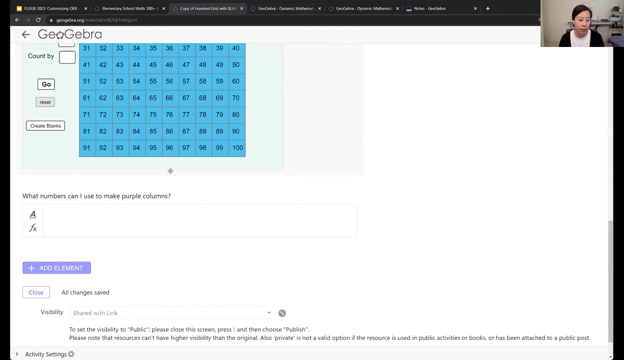 And say, uh, how? Yeah, Uh, What? Yeah, there's a better way to word that question, but Maybe I want to make, have them make notes of just the patterns and the shapes that they can make, while they're skip counting on a hundreds grid. 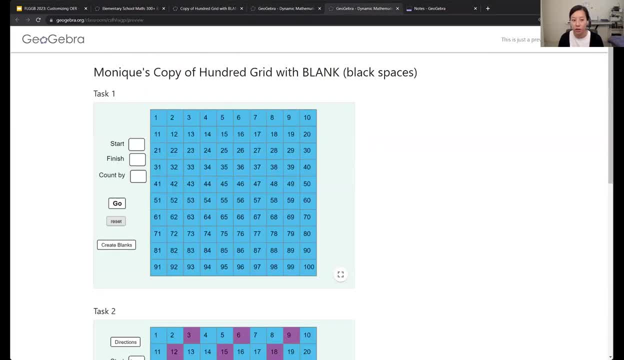 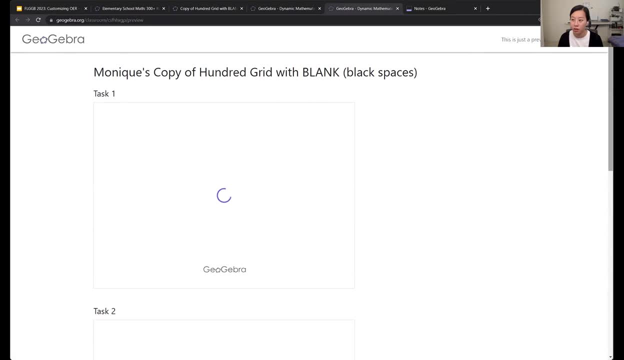 Um, So, um, I'm going to go ahead and add a question. Um, So, right now I just I can ask my students: Oh, just refresh your page. And then, as I scroll down, Oh, Did I save this? 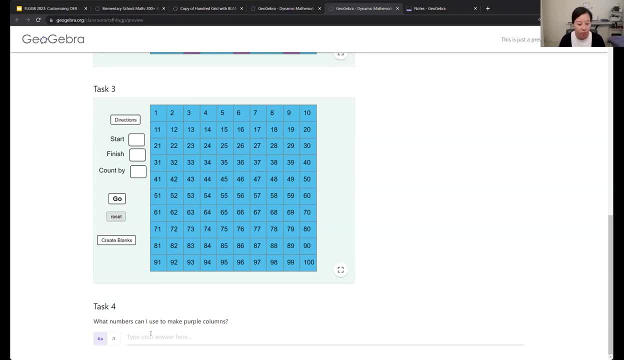 Should. Oh, there it goes. There it pops up Um. after students refresh the page, they'll be able to see: oh, I added this new question, So I like to show this feature, that, um, you can even make changes as the students go through the course. 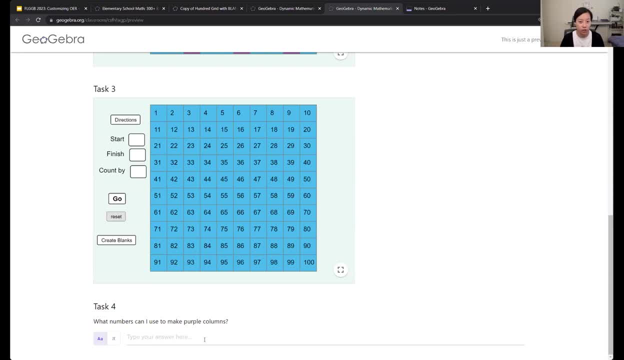 Um, you can even make changes, as the students are going are in your classroom and you've made a classroom out of your activity. Um, so if you wanted to add an extra question at the end, like, say, this is your exit ticket. 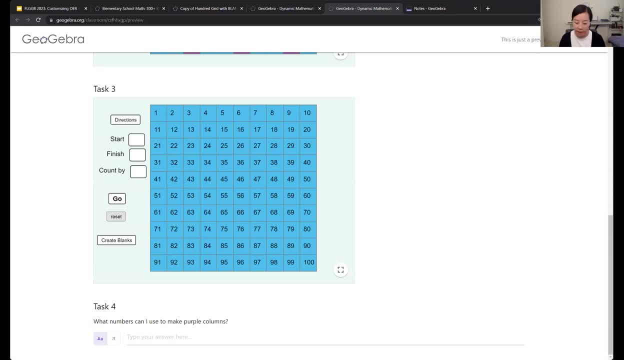 Um, that works great, Okay, And so this was me showing how you can take something. Uh, you can re revise it and you can remix it and you can distribute it. Um, so you can make changes And then you can add another one. 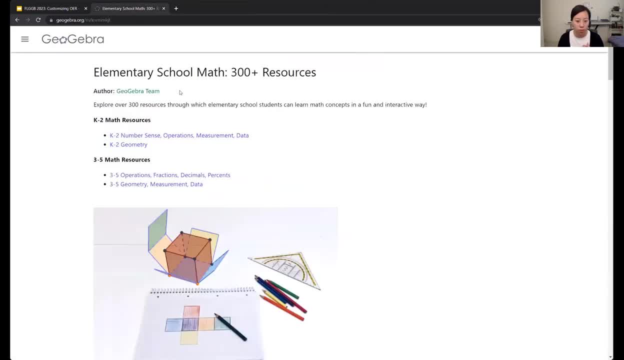 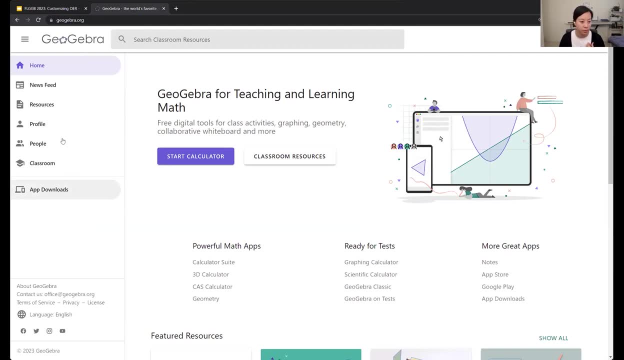 So I'm going to show you how to do that. Um, let's say, I'm at Geogebra, I'm using Geogebra classroom, Um, and then one last thing I wanted to do And show Before Our time is up. 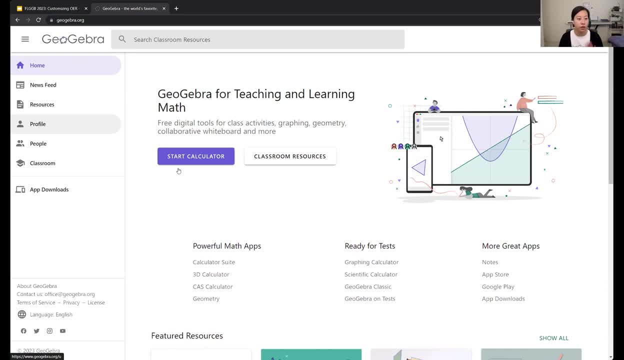 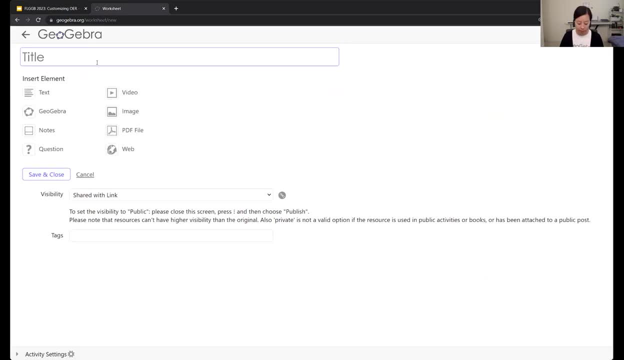 Is how to make something from scratch. So let's say, I'm at Geogebra, I want to make my own activity from scratch, And this will make something completely blank. So here is my activity from scratch. Um, and so I can start, of course, you know, inserting a text. 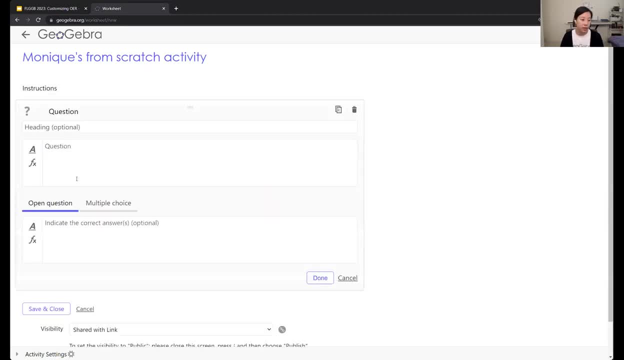 Or questions, Um, and so I like to have a question at the beginning of the class, just As a Starter. So, Uh, what Did you Eat? or breakfast, Just to kind of warm everyone up. Beginning of the class time. 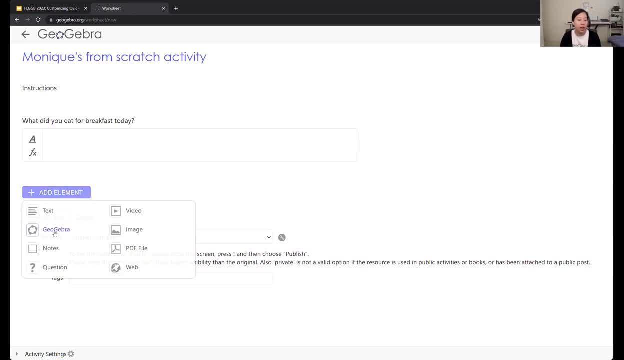 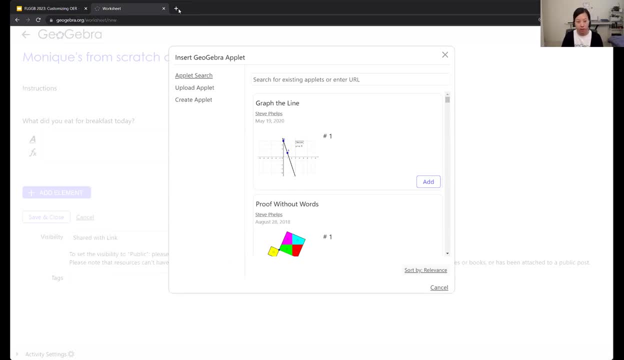 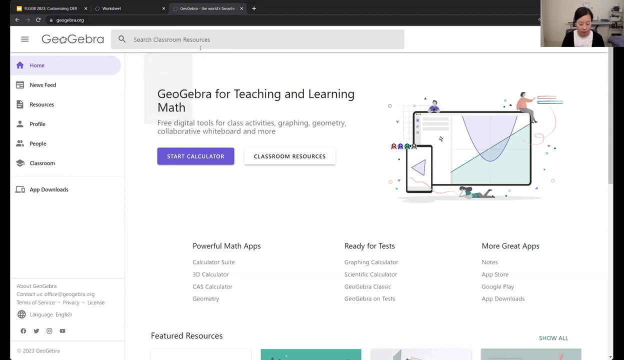 Um, and then something that you can do is you can also add a Geogebra element, And so you can search for something and then input it. So if I am teaching something about Um, Uh, Adding integers, Maybe I see this. 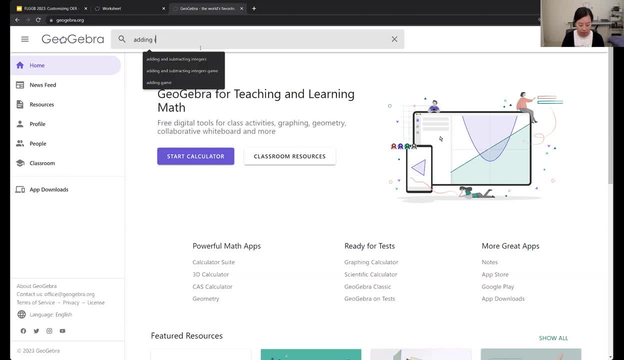 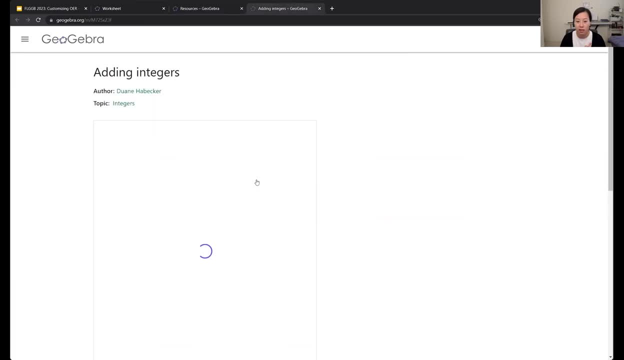 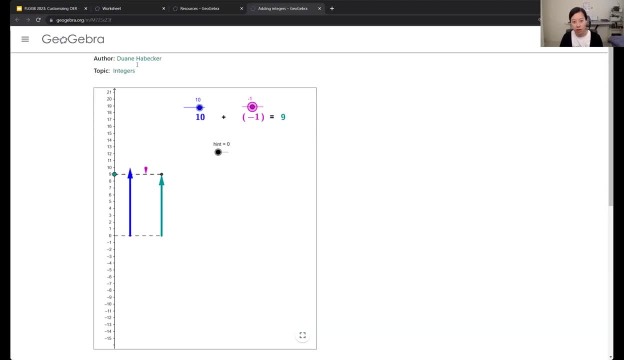 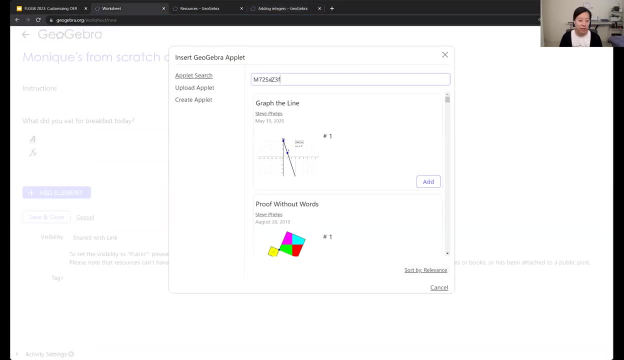 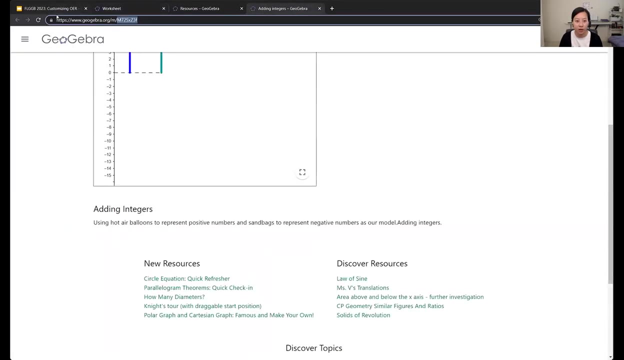 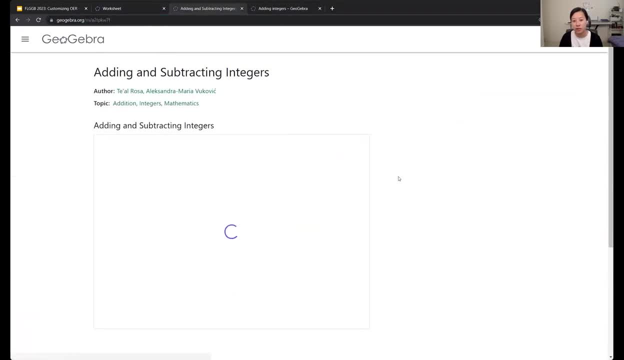 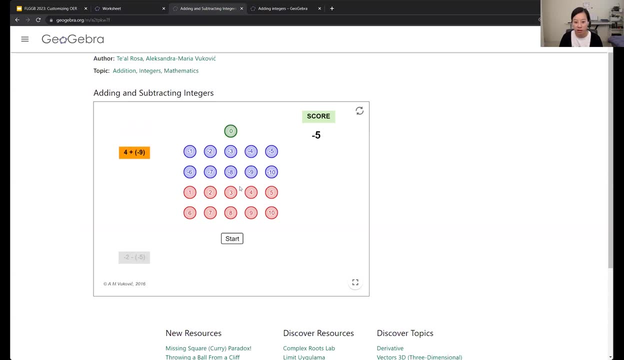 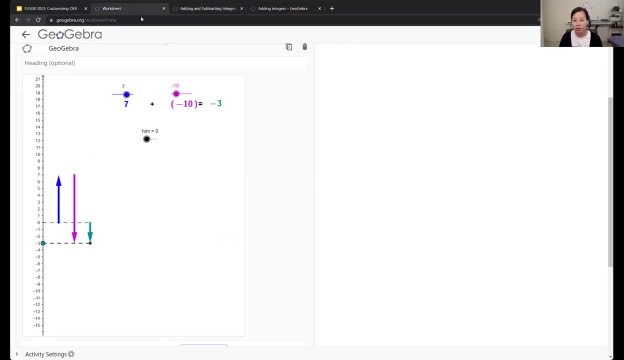 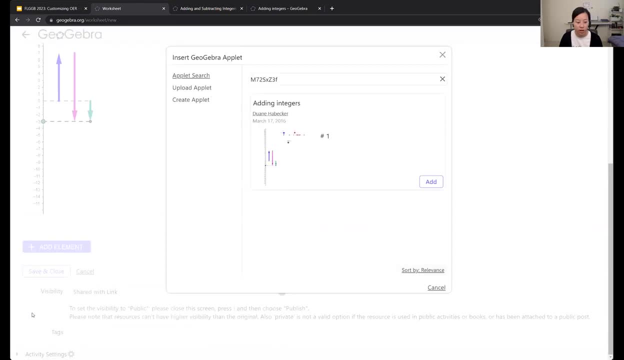 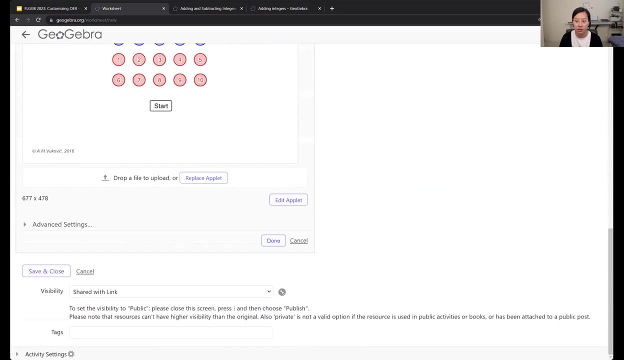 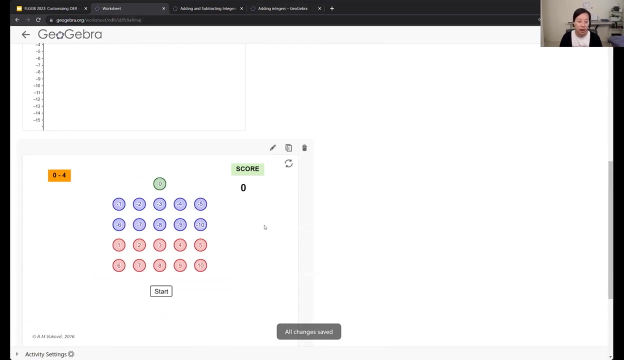 Make a copy of this And have it. at the very end Click Something. So I clicked on add element GeoGebra. I'm going to paste this new applet in, add it in save And when I save it to classroom it's when I look at the thumbnails of the scores. then I can have, we can have like a scoreboard going and we can kind of have a competitive class game at the end of our time. 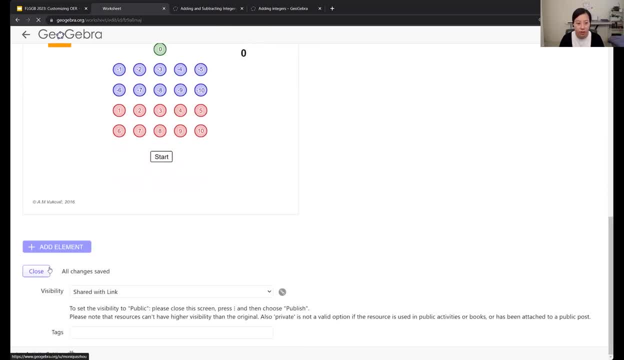 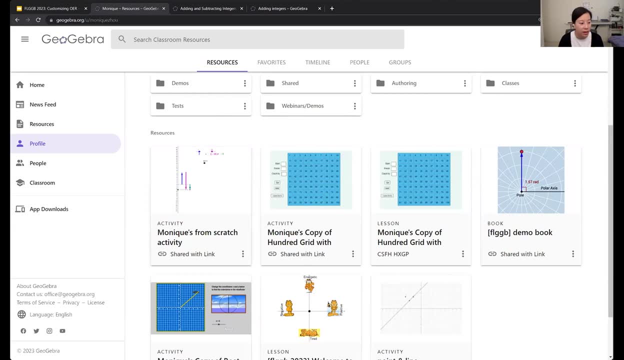 Yeah, And so I saved it. I will close it. Yeah, So that's one thing that we can do as well. And then, something that was mentioned earlier I wanted to just continue to show is when Tanya and Millie were talking about the present and the future of GeoGebra, they mentioned a content project that we've been working on. 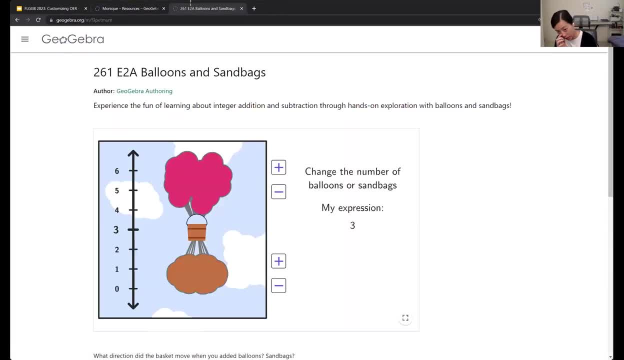 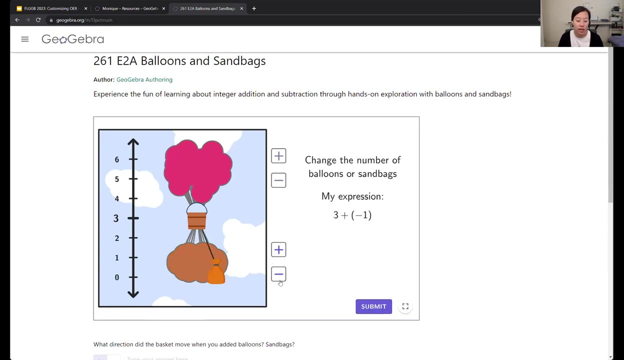 So I've been working on this content project as the lead and one of the resources that we might feature- That we are going to feature- is something like: this is a visualization of adding or subtracting integers, positive and negative numbers and what that could mean. 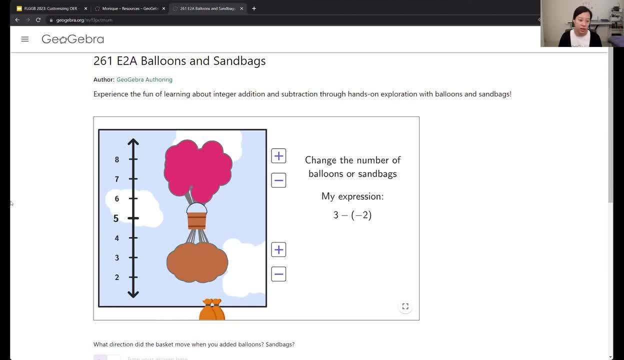 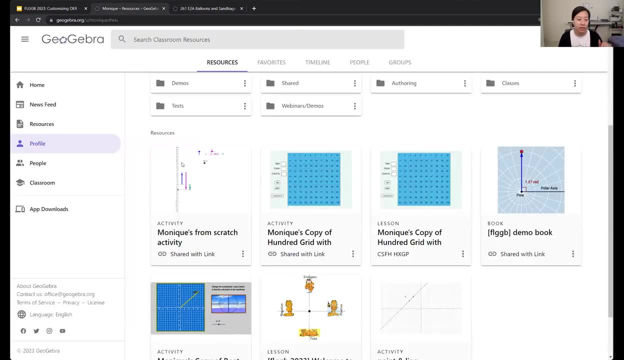 And so when these features get are these resources get released, they will also be available to customize or even just add on to add into books and share and things like that. So just keep your eye out on that content. I'm very excited about that. 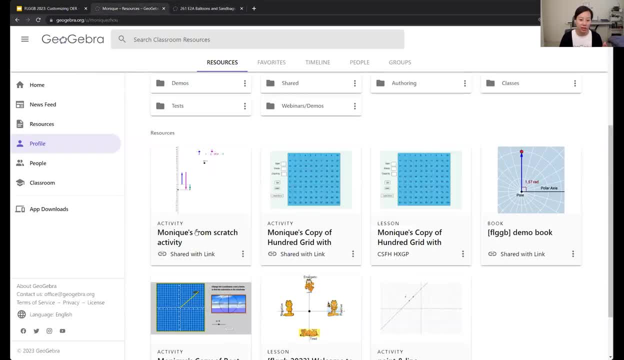 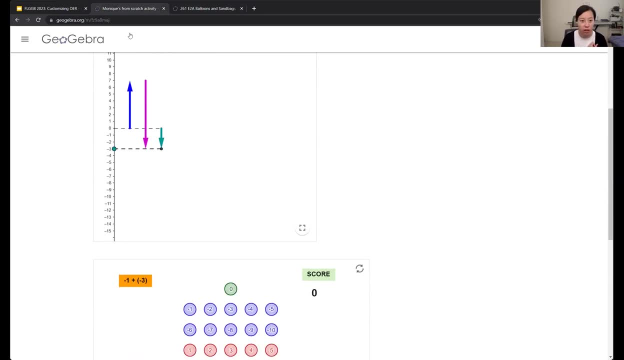 I'm very excited about that, But this is something that might go along with some of the this lesson that I was building earlier today. I know that was fast and I was running out of time, but I wanted to Just be available if there are any questions. 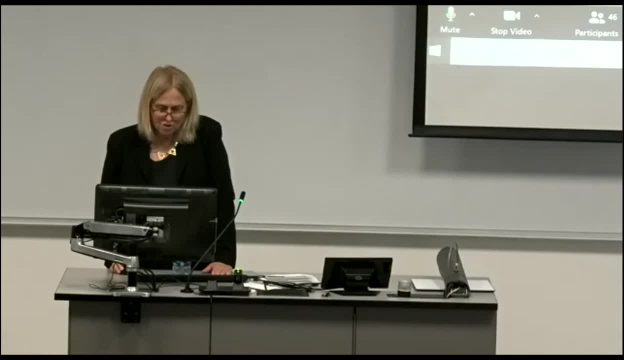 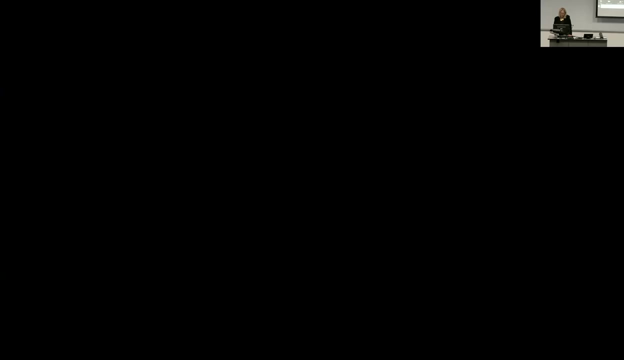 Hey Monica, Thank you so much. Let's see if there's any question. which For you all. here we are, as I said, Face to face, are people having a workshop in the person. So I think that that we don't have a question here. I hope you can send us some links or the link to the classroom You were sharing. Yes, So we can. 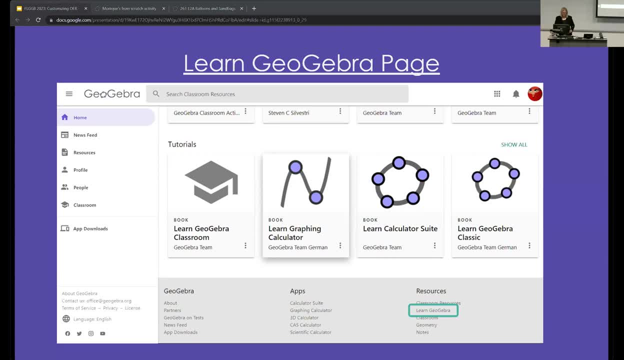 Yes, I can take, We can post it. Yes, I will take these links and I will put them in my slides as well. So it's all, all the links will be collected. Yes, I can take these links and I will put them in my slides as well. So it's all: all the links will be collected in one nice place and I will send it over. 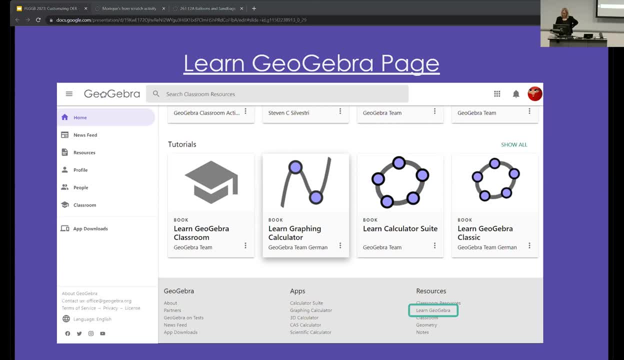 Thank you so much. send it to either someone down to me So we will post it on our conference to Gibraltar. Thank you so so much for you get this so great that you have supporting us. I'm repeating that, but this is: it feels so great that we have such a great speakers and sharing all the knowledge. 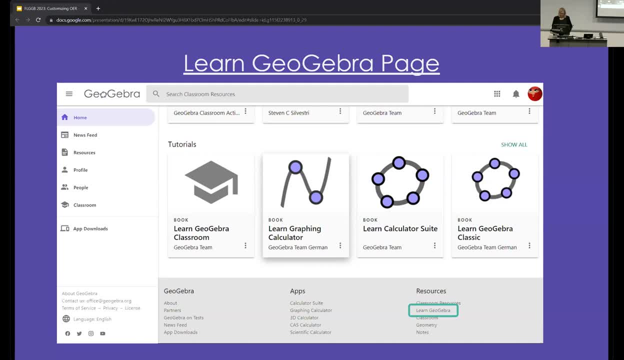 So thank you so much. Are there any questions right now to Monica? I don't know. OK, so thank you once more, We will have a break. Thank you, Oh yes, By the way, if you, any of you online- are still looking for more help, if you wanted, if you had more things you wanted to learn, I recommend just going to the home page of GeoGebra. 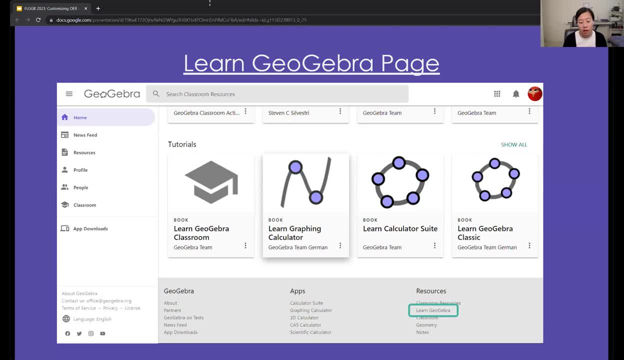 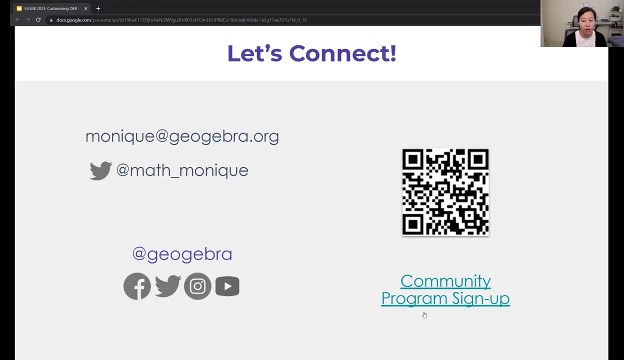 You scroll down, There's tutorials in some of the thumbnails, but there's also a link- that's a little bit hidden- for Learn GeoGebra. You'll find tutorials and forums and FAQs and things like that, And then, of course, my contact information will be here. This QR code on the side is for our community program. 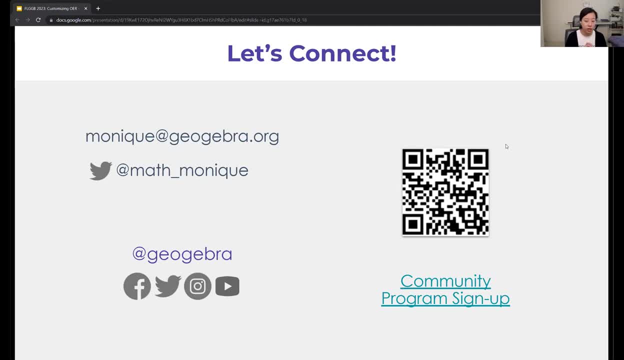 So if you wanted updates, especially about the content project that I'm working on, or more information about things like webinars or other events that we might also have from the GeoGebra end, it's all here. Thanks so much, Kasia, Wonderful, Wonderful. Thank you so much. 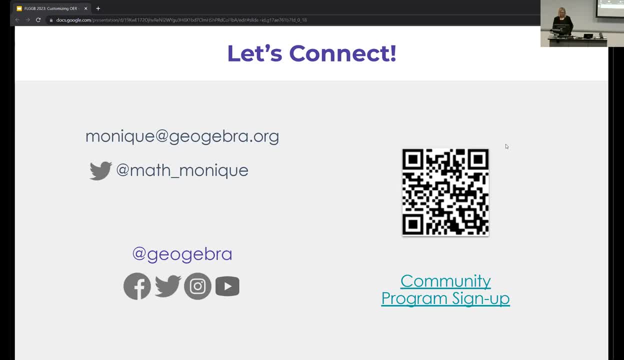 Thank you. OK, so we are stop stop recording Now and we will have some. 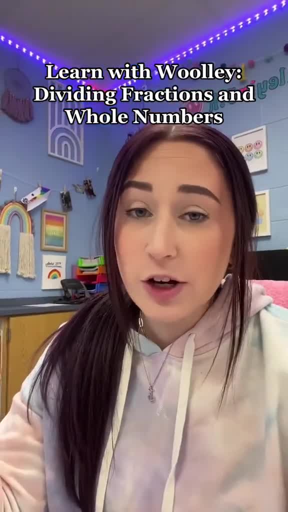 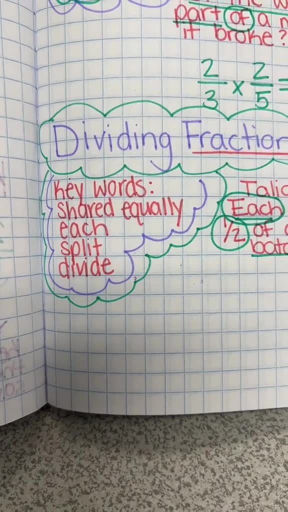 Let's talk about dividing fractions and whole numbers, Just like multiplying fractions. when you divide fractions from a story problem, you have some key words. The lights went off. In story problems you might hear words like shared equally each split. 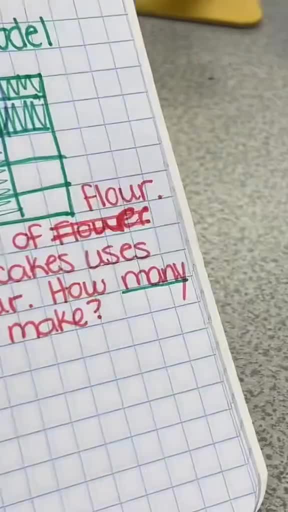 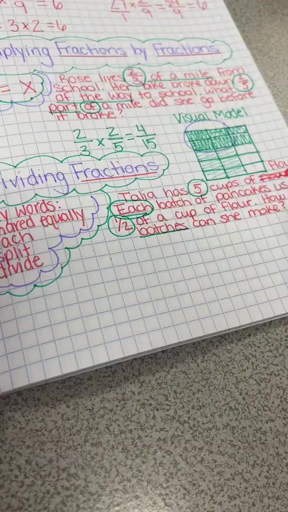 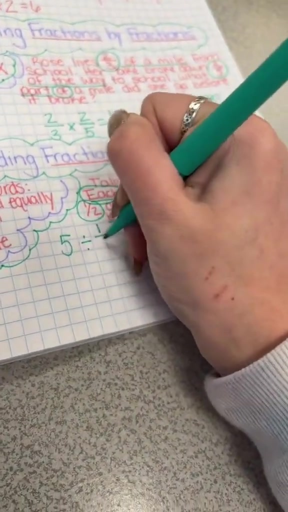 divide. For example, Talia has five cups of flour. Wasn't paying attention, spelled it wrong. Each batch of pancakes uses one half of a cup of flour. How many batches can she make? Well, let's see. She has five cups of flour to start with and I need to divide it by one half because 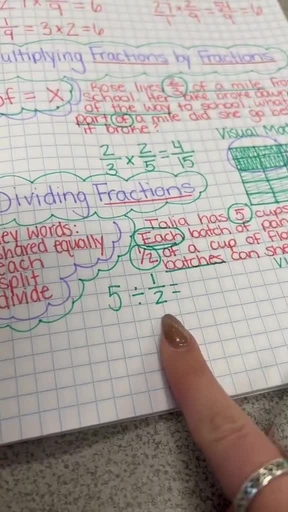 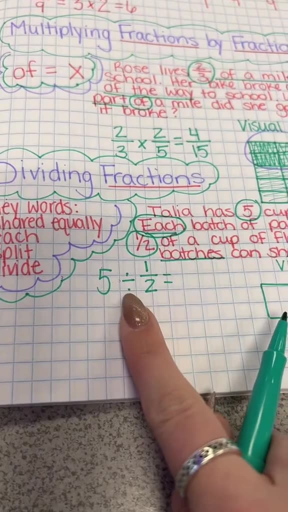 each of those batches takes one half of a cup. It's like I'm trying to figure out how many groups of one half I can get out of that five cups of flour. So first I'm going to draw my five cups of flour, Then I'm going to divide each of them into two parts, Then I'm going to put them into 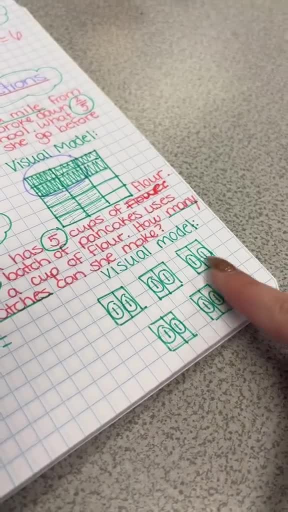 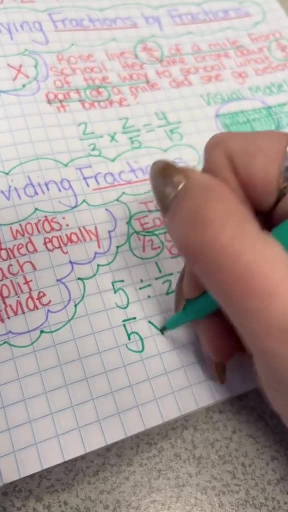 groups of one half and see how many I have. Each of these is a half, so I can make 10 batches of pancakes. I can even check my work by multiplying by the reciprocal Keep, change, flip. Keep the first number, change the operator, flip the second number. Five times two is ten. Hope that helped.